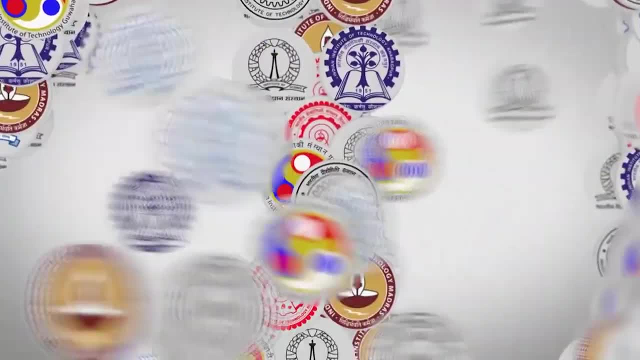 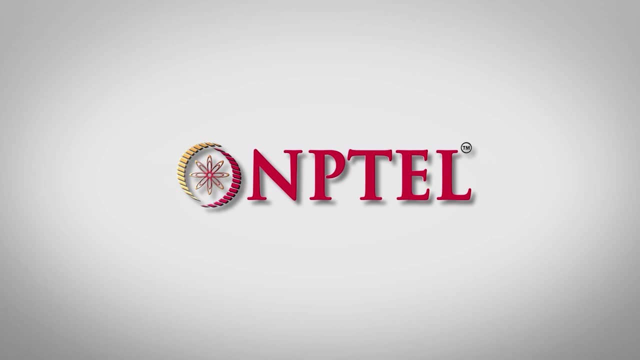 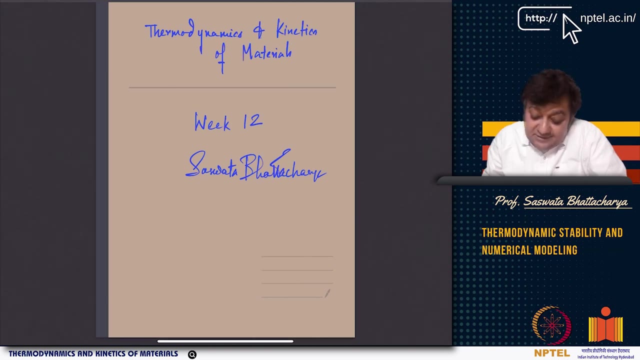 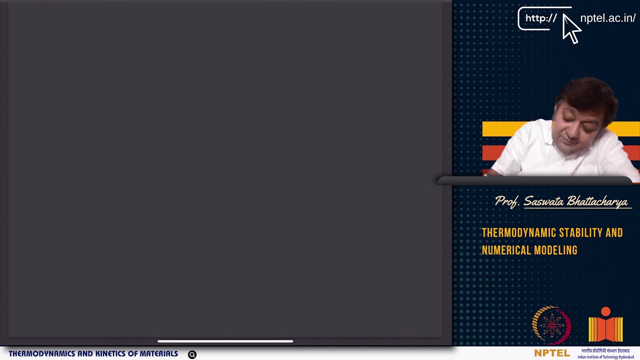 Welcome to the twelfth week that is the last week lectures and of this course Thermodynamics and Kinetics of Materials and this is Shashwatha and so in the last week in the concluding week we look at. So, we have so far looked at equilibrium right phase equilibrium. So, we have looked at phase equilibrium, we have looked at phase diagrams, we have looked at binary phase diagrams. We did not look at the ternary phase diagrams, but in ternary phase diagrams it is basically as you know we use isothermal section and if required later if you want some pointers to ternary phase diagrams please contact me. So, I will be ready to help you. So, we looked at phase equilibrium and we looked at conditions. We looked at unary systems, we looked at multi multi phase multi component systems, we looked at the fundamentals of thermodynamics principles how they apply to phase change, how they apply to solutions and different solution models. However, we had to look at so we always talked about extremization of entropy as one of the criteria and then we looked at all this for simple systems. We looked at the conditions, we looked at arrived at the different thermodynamic conditions for example p alpha equals to p beta. If alpha and beta are in equilibrium you have p alpha equal to p beta equal to p gamma say alpha 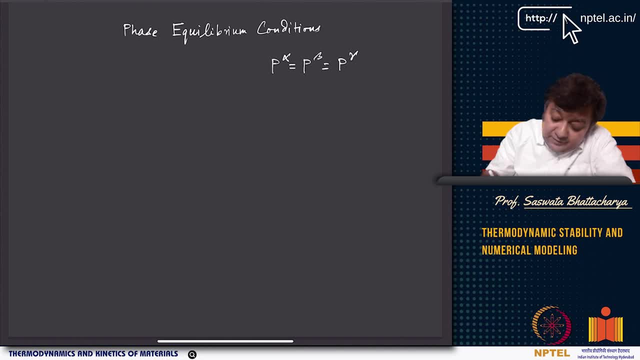 beta gamma are in equilibrium. Then we looked at also for each constituents say you have two constituents mu a alpha equals to mu a beta equals to mu a gamma. So, this is another equilibrium condition similarly for other component if I have a binary system u v alpha equals to mu x. Hence mu x equals to the equilibrium condition. When we try mu b beta i plus 2 mu b gamma. We also looked at the thermal equilibrium T alpha T beta 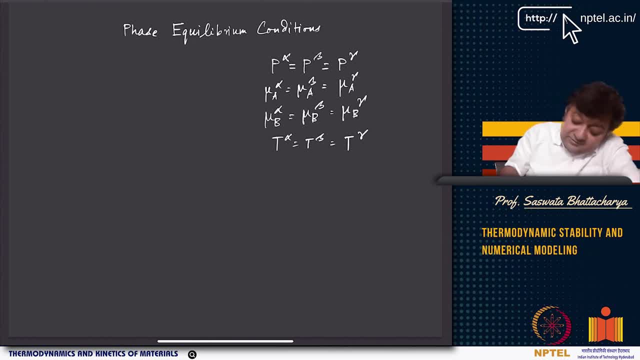 T. However, we need to discuss about stability right stability which is related to the second derivative right. Stable equilibrium whether the equilibrium is a stable equilibrium that is some metastable equilibrium we have discussed metastability, but we have discussed even unstable systems right we have discussed instability gap below at a temperature below which a solution becomes unstable and phase separates. We have looked at that, but how we formally treat stability is something that we will discuss. And instability in the context of stability we look at some aspect like numerical modeling. So, if I numerical modeling means we basically 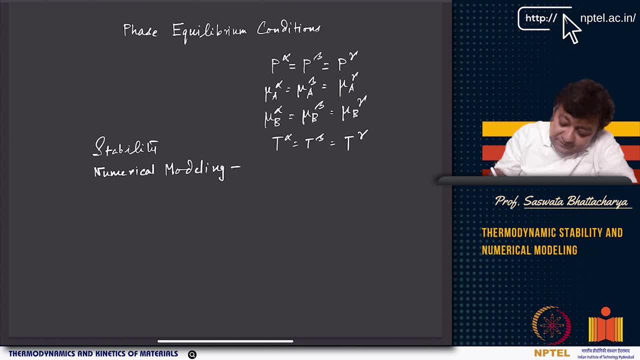 will use Newtonian model and then we can use something called Newtonian model. 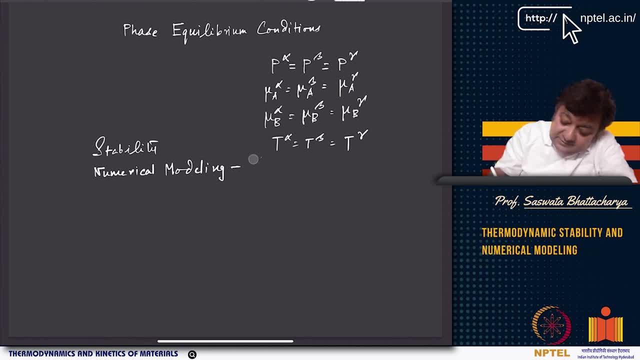 So, the from the g x curves that is from the solution models g x curves we will see some g x curves and from that if we can use common tangent construction. So, basically that is something that we will do right g x curves and common tangent construction and also we look at thermodynamics of reacting systems. 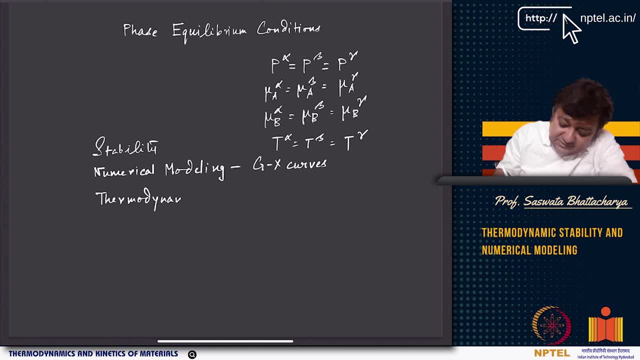 So, we initially at the initial stages we discussed from the thermochemistry thermodynamics of reactions involved in terms of reactions whether they are endothermic or exothermic, but here we will go a little bit more detail we will look at Ellingham diagrams as example. And finally, and finally we will look at some examples of interfacial thermodynamics. So, 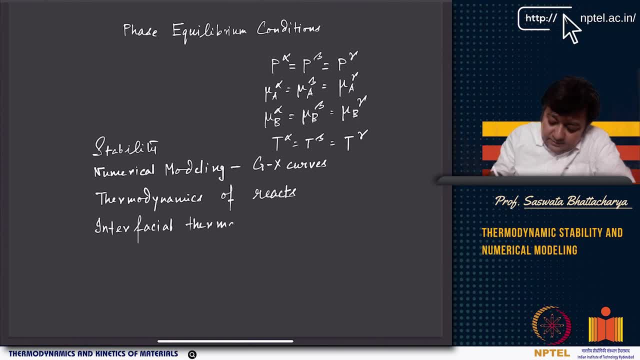 these are the three lectures are there. So, over the interfacial thermodynamics and a brief introduction to irreversible thermodynamics which is basically the basis of kinetics. And, there we will look at the, we will look at the interstitial thermodynamics. And, there we will look at the interstitial thermodynamics and the interstitial thermodynamics. This is, at particularly how it applies to this flux force relations right. 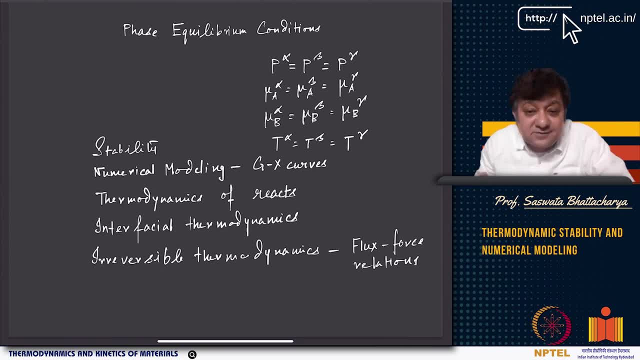 And this is where we will conclude although the irreversible thermodynamics part if you 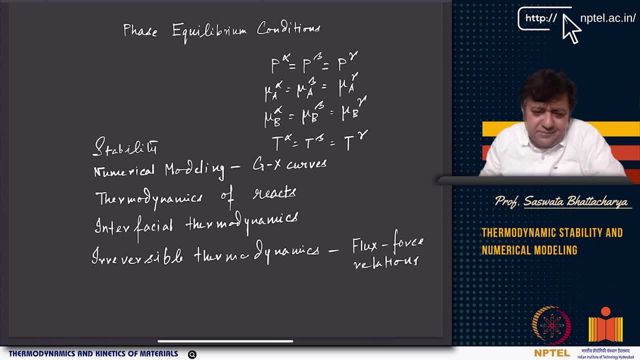 want further information because it is just an introduction of very preliminary introduction. So, if you want to go further deep into the irreversible thermodynamics part as you can see in the layout of the course, we initially had lot more on diffusion. However, we changed it the layout a little bit on because you see there is a we discussed the all thermodynamic principles in details ok. So, we basically did not want to get into a lot of kinetics, but we wanted to get into the idea behind kinetics the principles of kinetics and that is what I will talk about and that is where irreversible thermodynamics comes about. However, as you can see that these are very important. 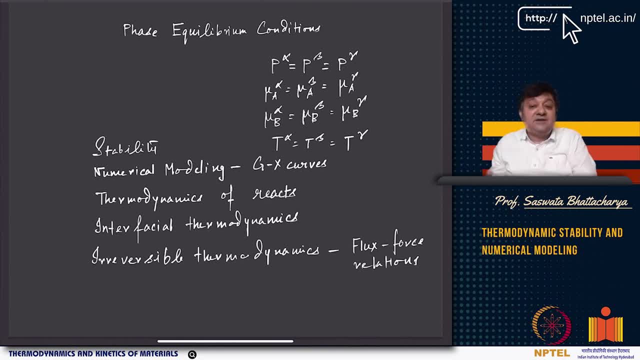 So, it is very involved and detailed and it may require a separate set of lectures right and and we can we can also have discussion offline. So, as you know you can reach me at my email id and if you have any doubt and also there is a forum right now, but in the forum mostly what is discussed in the class is what will be what will be discussed further, but beyond the forum if you want to know something more advanced you can always contact me by my over my email. So, thank you very much. 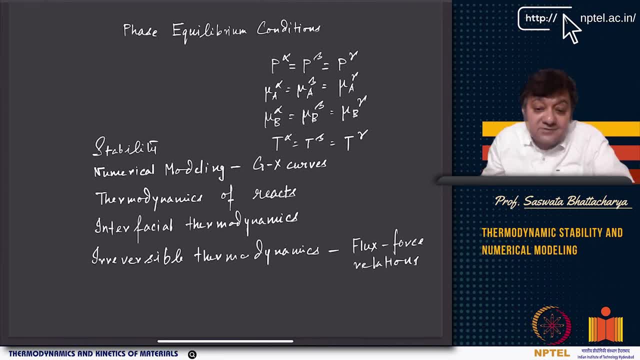 I will send you an email and send me an email and I will try to help you as much as possible. 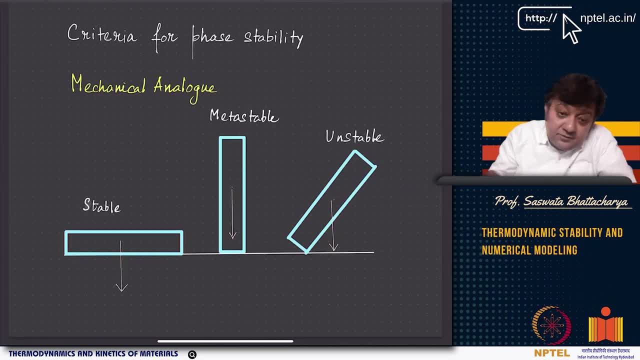 Now I will start with the criteria for stability. Now you know when we talk about stability one of the easiest ways to understand stability is by using a mechanical analog. So, if I take a mechanical analog think of a piece of material which is in the form of this box as you can see here. So, this is like a rectangular parallelepiped. So, if you look at it you can see that it is it is it is a it is a it is not a bar it is like you know in a cross sectionally think of this is like a book to see. So, and you are looking at a book. So, basically you are looking at something like this and then you have this and this right. 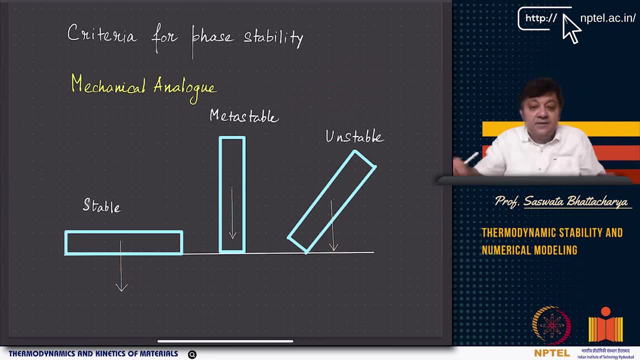 So, you are looking at that. Now, if you look at this this this squarish bar or bin or you if you can call it a this this material you can immediately see here there is a long edge and there is a short edge of this material right. You you are looking at the cross section here you are looking at the cross section here, but if you can think of it is like like like a column a small column rectangular column like this think of a rectangular column. If you have played a game of Jenga you will see in the Jenga there are these pieces these wooden pieces. . So, these three dimensional wooden pieces or blocks. So, I am talking about one block which has a long edge and which has a short edge right which has some thickness and which has which is also having some height and some width ok. So, I am not looking at the width as such, but we are looking at the thickness section and the height. Now, if you see the long edge if the long edge rests and my centre of mass is somewhere here see at the lowest level where the long edge is resting on the ground or on the surface. 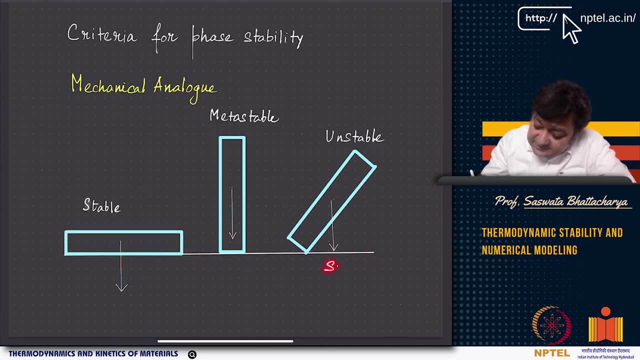 So, this is your surface this guy is your surface on which the long edge is resting. 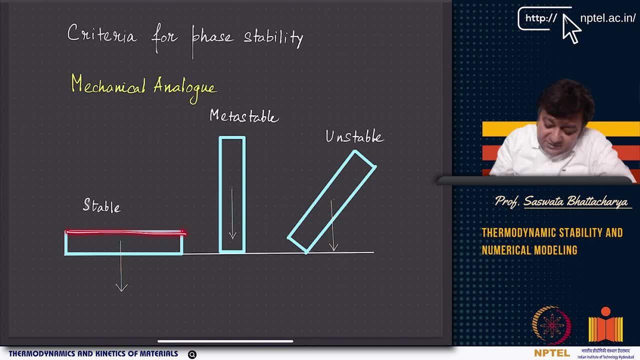 Now, if you the long edge is resting if you look at this orientation here is your centre of mass roughly here is your centre of mass right this is the weight of the block. Now, 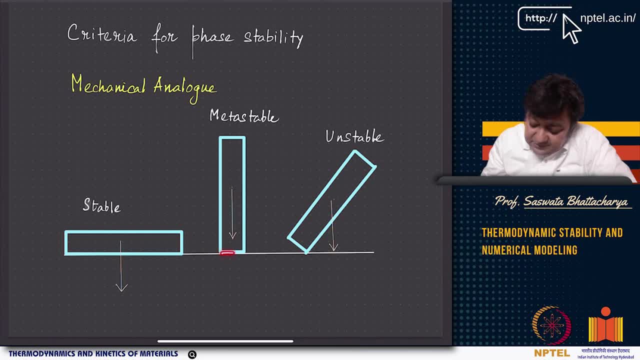 however you can also set the block in such a way that it is resting on the short edge instead of the long edge instead of the long edge it is resting the the the the it is resting on the short edge. Now, in this case in this case for example even if I move if I try to 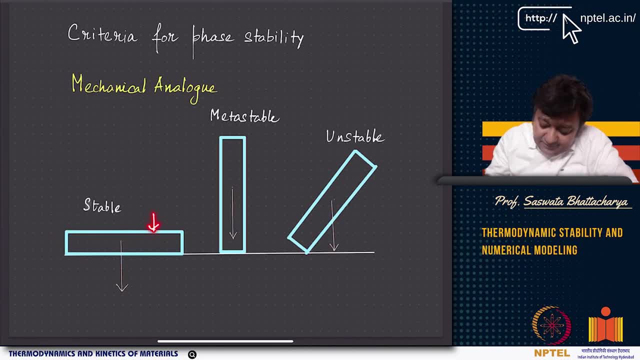 force it if I try to apply some force on it if I try to apply some force on it it will move here and there slightly, but it will not destabilize right it will not destabilize 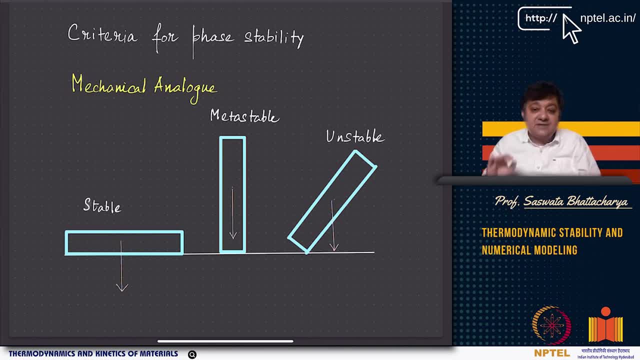 the stable equilibrium right it will just remain as it is. However, if you look at this the metastable the if you see you can immediately understand why it is metastable because as you can see the centre of mass has gone up of the right the way I have stated on the short edge the centre of mass is somewhere here and if you push it slightly then right 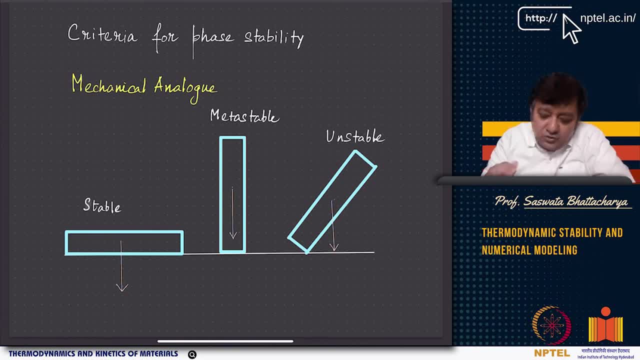 not very slightly, but yeah you give it give a little shove then basically if you if you give a little shove then it falls right it falls such that it again. So, if I if I say for example produce a force like this it will fall and once it falls it will rest on this 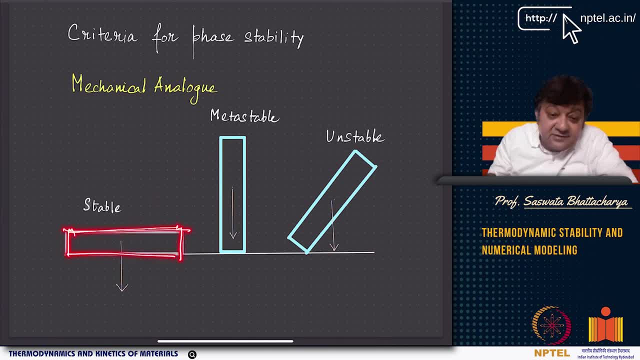 stable equilibrium. So, if you see stable is the lowest the if you look at the stable equilibrium this is 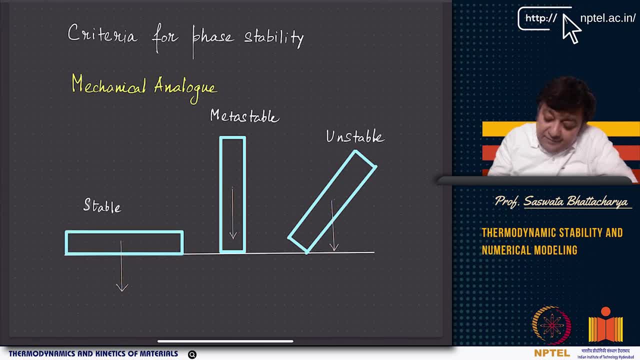 the lowest energy state. Now, if I push it or shove it a little bit then it will fall in such a way that it comes comes to a more stable equilibrium. So, the metastable equilibrium so that is why this is called metastable because from metastable I can go to further more stable 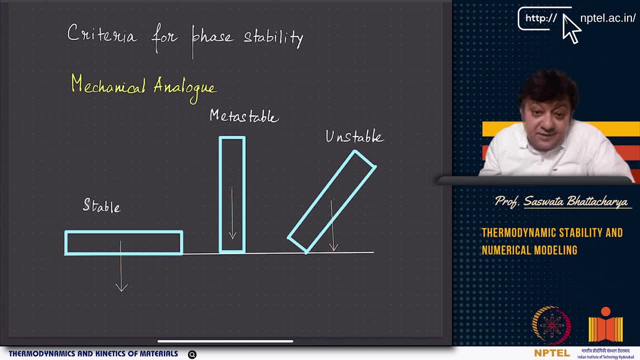 equilibrium. Now, if I look at unstable say there is something called unstable equilibrium something like I am basically somehow I am balancing it on one corner somehow I know or somehow I like like like a magician I have balanced it on some corner and it is just barely there. So, you can see a small touch a small touch or small disturbance even a small sound it can immediately if you you will see that it will immediately fall on the launch right. 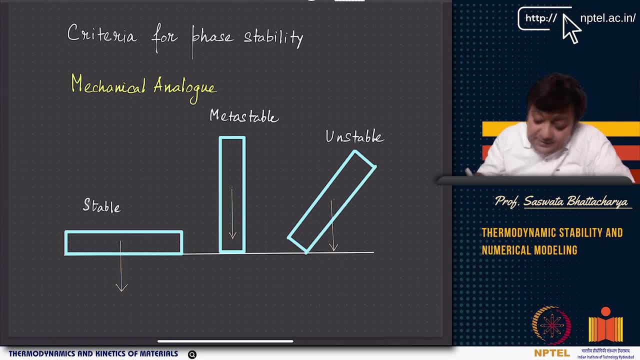 it will fall on the long edge. It will again the unstable one will tend to go. So, there is there are two things that can happen here. This unstable one can fall like this and then it will rest on the long edge. It becomes a stable equilibrium. So, this guy if it falls like this. However, there is also a possibility that I force it like this. Then it will just go up and it is possible that it will come to a metastable equilibrium. So, the unstable one can either be metastable or be stable, right. The unstable one can either be metastable can either reach a metastable equilibrium if I basically force it this way. If I force it this way, if I just touch it this way immediately it will fall to a stable equilibrium, right. So, stable equilibrium is the one that it does not want to change at all. Unless we have regressively disturbed it, unless we have moved it from there and we have we have we have forced it to be metastable or unstable, it will remain in stable equilibrium. 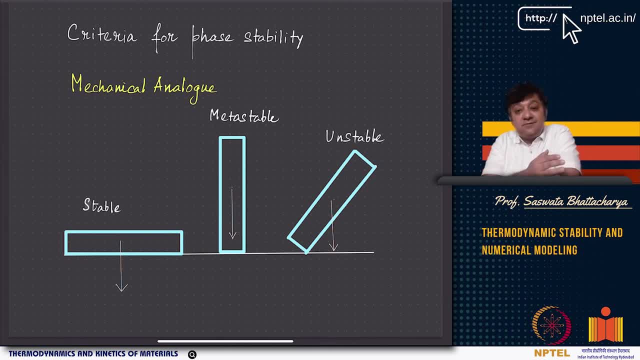 However, when it is in metastable equilibrium, if there is an energy or a driving force metastable equilibrium will change to stable equilibrium, correct. Metastable equilibrium will change 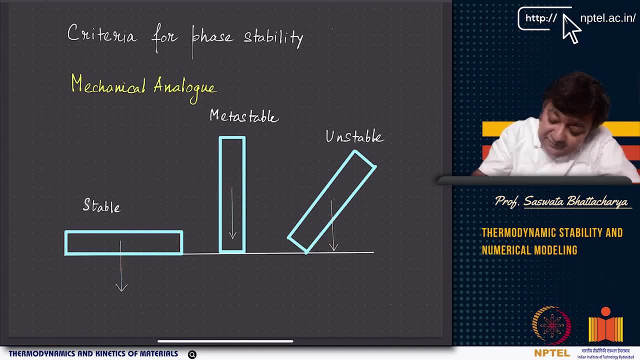 to stable equilibrium. Now, if I look at this from an energy point of view, if I look at this from some energy point of view, then it is the energy and think of this. You are somewhere here. Okay. 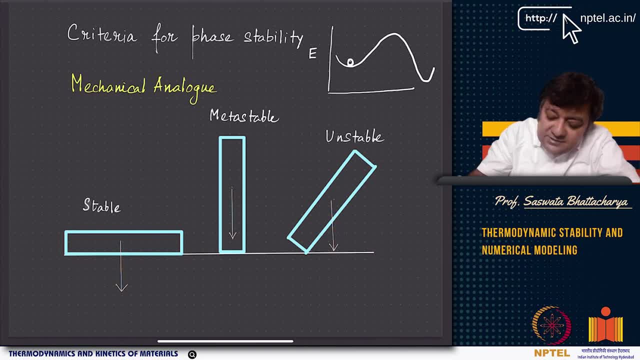 So, this is the energy landscape. Now, here I will call it it is locally stable equilibrium, but if I it may here for example, the ball will roll either this way or this way, right. I have a ball I have a ball here, if you can see there is a ball here. And the ball can either roll this way, right you have a heel here you have put a ball here and this is the energy. So, this is the highest energy, as you can see this is the energy landscape, right. This is the energy landscape that I am talking about. It is a beautiful energy landscape. 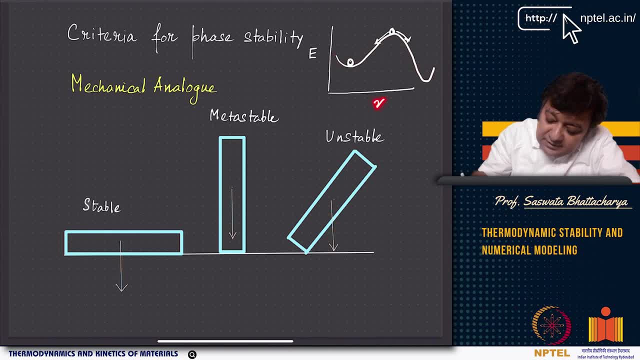 Okay. and say this is my position coordinate r, okay, position coordinate r. So, if I have such a coordinate and if I have some particle here resting, the particle here will be in a highly unstable state. A little push can either push it down this hill, this hillside or along this hillside. Now, if you see the driving force for going here is much more than the driving force for going here. However, if it starts rolling in this direction, if it starts rolling in this direction, it will reach metastable equilibrium rather than the stable equilibrium, right. It will reach metastable equilibrium. In fact, I can think of a better diagram. Say, for example, I have this. Now, you see I have a ball here, okay. So, let me just this here. 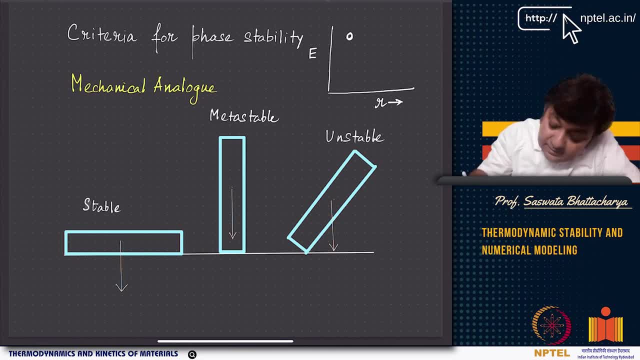 Now, if the ball is rolling, this part is becoming a neutral equilibrium. So, that is where I want to change it a little bit to a stable equilibrium. So, basically, make it a little unstable. 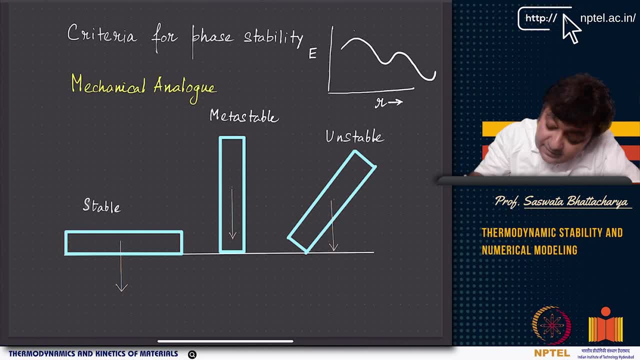 Now, You are here, somewhere the ball is somewhere here. Okay. Now you have just given a little displacement, means you have displaced it a little from the position. So, you have given a little displacement from this position. What happens? It falls in and it goes here, right. The ball has 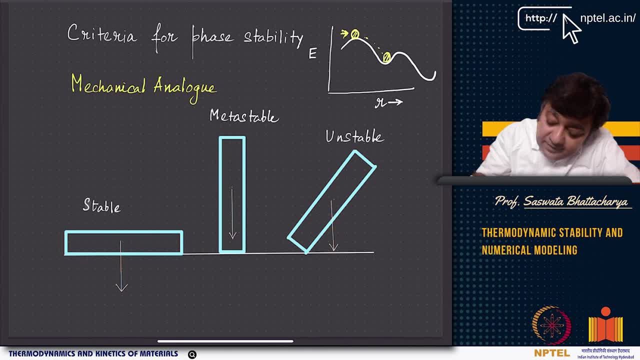 gone here, right. It, it is going going here. However, if I force it a little more, if I give it up more than a slide push, if I give it more than a slide push, if I give it more than a slide push, it goes everywhere, you see, you do not like that. It is living right here, right. Now, I am doing the work Rita. It has shown you this, right. Like, you give the momentum why you are giving 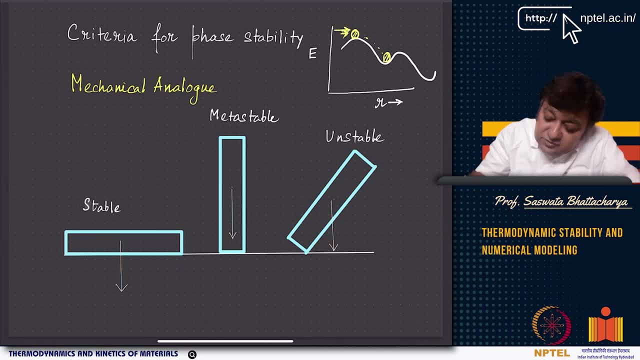 the momentum why you are giving the momentum. This is very important. Now, all right. So, you than a slight push if I make it a larger push, then it is possible that ball will basically 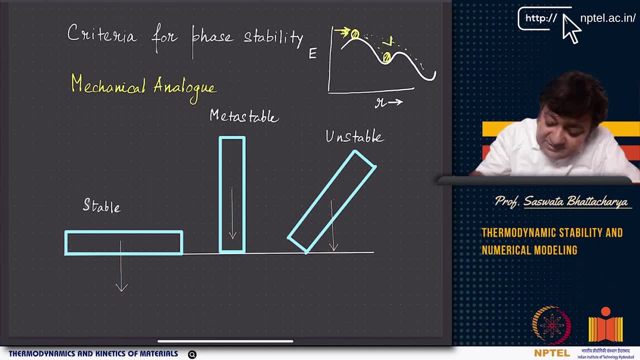 directly follow this trajectory and come. Now, as you can see this is the stable equilibrium, this is the metastable equilibrium and this is the unstable equilibrium, right. So, you have metastable, metastable and unstable. So, as you can see here, so if I want to apply 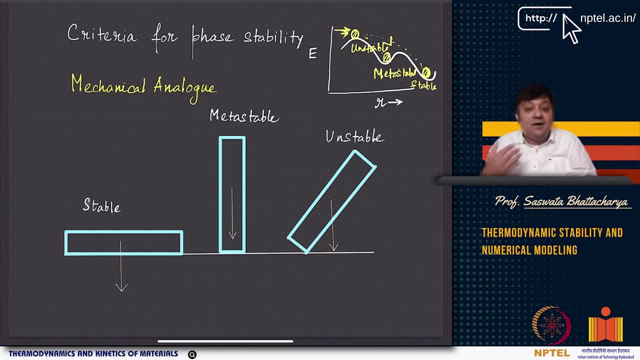 this mechanical analog or this energy surface, how do I basically understand it in terms 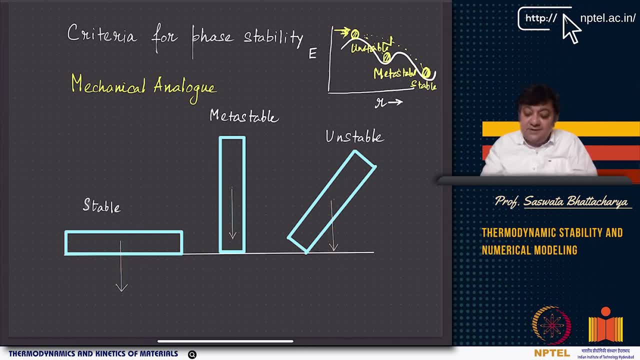 of phase stability, in terms of phase stability is what we will discuss now, right. So, we have given a mechanical analog, see look at this, you have given a mechanical analog of phase stability and you have also given energy surface, you have drawn some imaginary energy 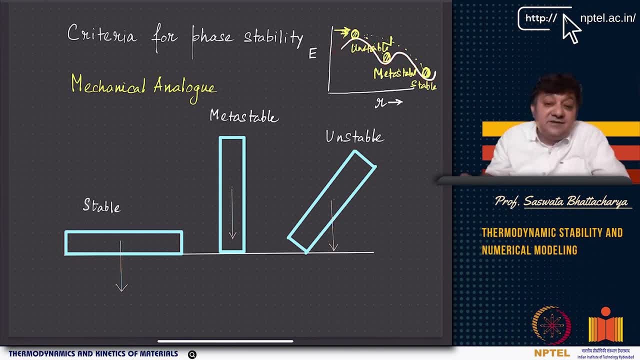 surface. . We look at the energy surface, we look at the energy surfaces we generally encounter and this is energy surface of functional position, 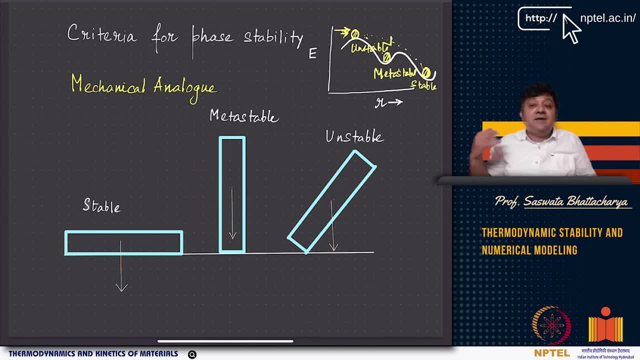 right on the energy surface. So, if you see there are positions where the equilibrium will be unstable, there are positions where the equilibrium will be metastable and there are positions where the equilibrium is the most stable one and once you have gone to the metastable that to the unstable one, you do not sorry to the stable one, the most stable one. Once you have gone here, you do not want to there is no way unless there is a big external force, you cannot go to the unstable one or the metastable, right. However, a very little disturbance to the unstable equilibrium will lead it to either a metastable equilibrium or it may lead it to the more stable, most stable equilibrium, right. So, this is what 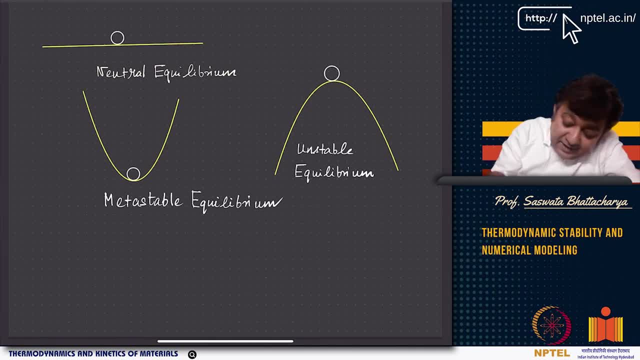 we are talking about and here is an example here and I am talking about another interesting case here. So, you have a very flat surface and the in the particle is here, the particle is here and you have very flat surface. Now, this has same energy, this has same energy, so if I am here same energy, if I am here, if I am here in all these points along this surface the energy remains the same. So, this is called a neutral equilibrium, right. You just remain there, if you displace it slightly the energy does not change, so it is called a neutral equilibrium. . 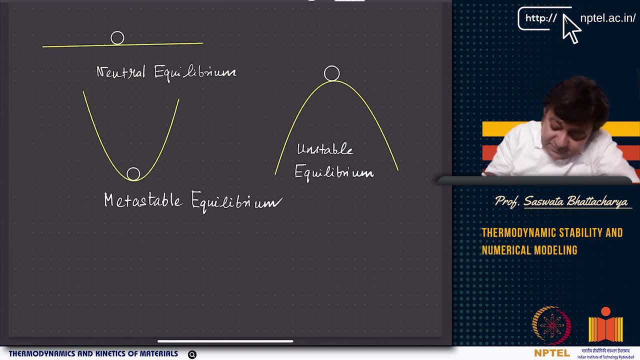 A metastable equilibrium, why am I calling this metastable? Because there is a possibility that there are there is say a further, means there is a further downward slope somewhere. 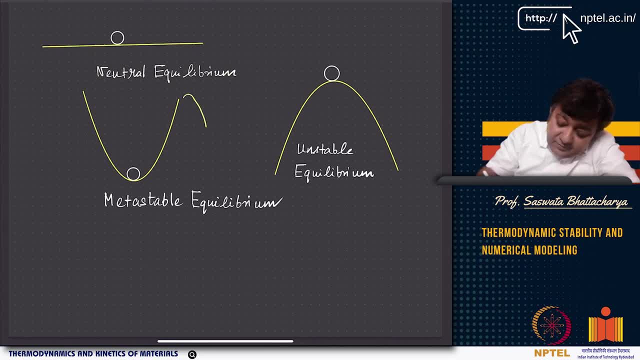 So, you have say for example, some more downward slope here, right. So, it is possible, right. So, that is why we call it a metastable equilibrium, right. We call it a metastable equilibrium. 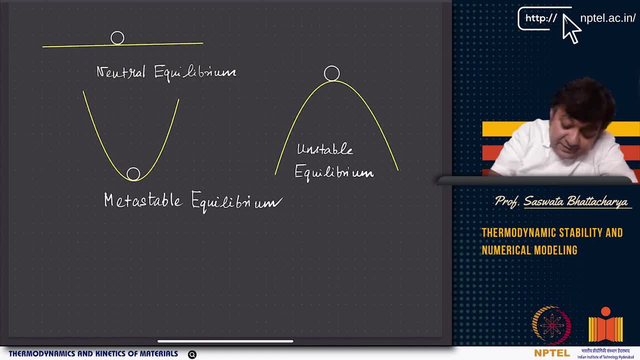 You can also call it stable equilibrium, if there is no such metastability, if this is the lowest energy position, if this is the lowest energy position, then you can call it a metastable equilibrium. . 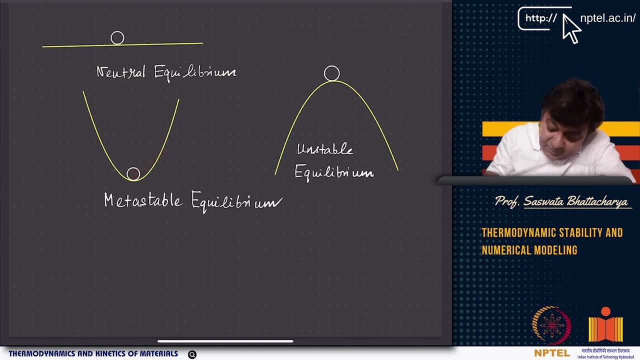 So, you are at the lowest energy position of the ball, this is the lowest energy position of the ball then this metastable equilibrium becomes a stable equilibrium, right. Metastable 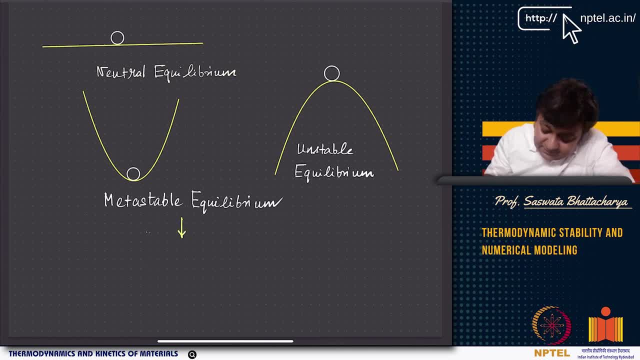 equilibrium becomes a stable equilibrium. However, have a look at the instability. Say have a look at this position, where you are at the top the hill the peak and if you are at the peak of this energy barrier. So, if you are in the peak, this peak is very, 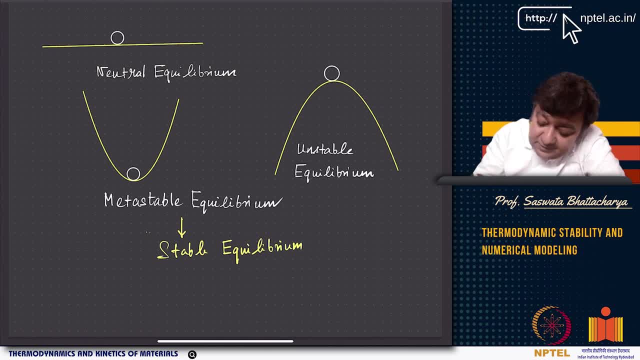 This peak is basically the giving you the unstable equilibrium condition, unstable because if I displace it this way or this way the ball will just roll, right. 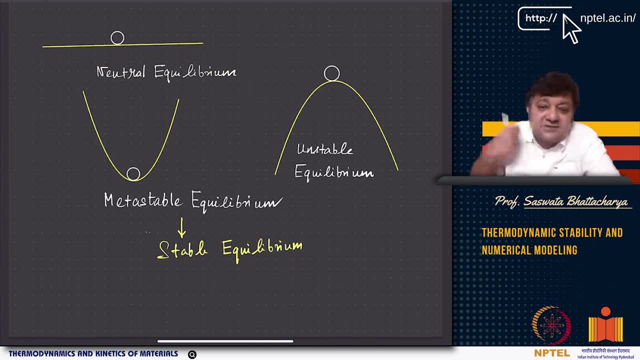 I displace it very slightly the ball starts rolling, a little disturbance it will just go to either a metastable equilibrium or a stable equilibrium, right so that is the idea. 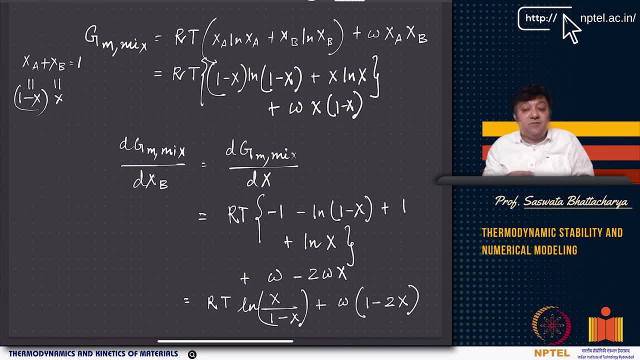 Let us look at that in the context of this solution model, right we have already looked at something called phase separation, right we have looked at the regular solution model where we looked at something like phase separation where A atoms favor A atoms and the B atoms favor B, right. So, basically if I want to write the excess energy due to mixing or the energy due to mixing then it has one delta S mix, right it has a delta S mix this is your delta S mix contribution and there is a T delta S mix, right. So, minus T delta S mix basically gives you R T x a L and x a plus x b L. 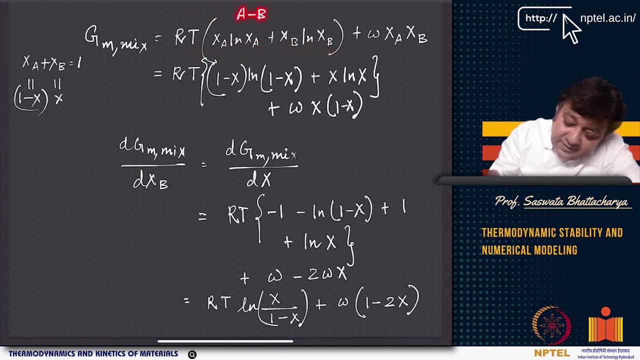 So, this is the E minus delta S, right. Now, let us get the two units, which are equal to one delta S mix and one delta A x b for a binary solution. If I take a binary solution this term is basically minus T delta S x, right this has a mix. And then you have the regular solution parameter so this is the delta H x, delta H x, right x a and x b are the mole fractions of A n. In fact if I if since x a plus x b is 1 I can take 1 minus x and x. 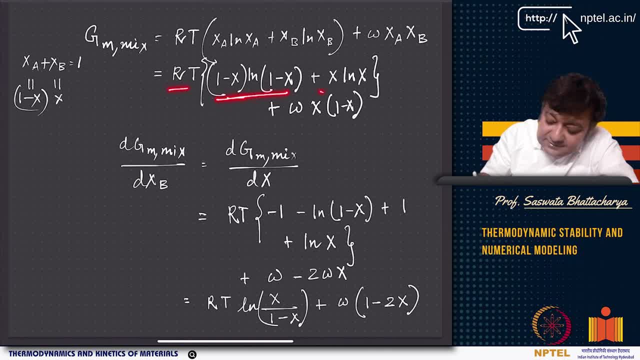 . So, basically this becomes R T 2 x delta x. So, here what we can do if we work with t 1 minus x ln 1 minus x plus x ln x is the same term here and then this guy becomes omega x 1 minus x just writing it this way right. Now, I want to basically take a derivative of it I want to take a derivative of it. So, d g m d x d g m d x basically comes out to be r t ln x by 1 minus x plus omega 1 minus 2 x ok. So, basically this basically gives 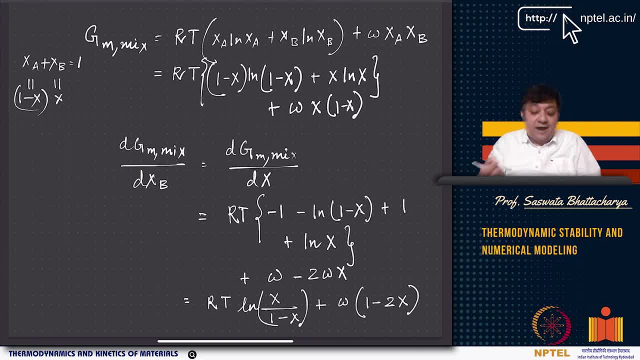 me a slope right of the curve the slope of the curve at any point right it basically gives me a slope of the curve at any point. So, if I have a curve like this, so if I have a curve like this one single curve. So, if I have a curve like this I have a curve like right and then basically this is my, so if I have this curve for example, as a function 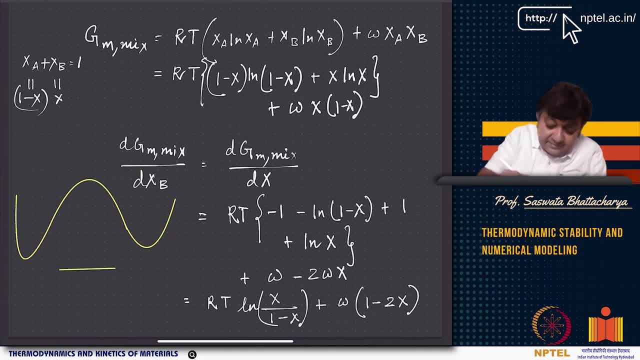 of x. So, if I look at this as x, x is the composition of, it is a mole fraction of v say and this is my, the y axis, y axis is say g m. Now, this is g m mix for example, the energy of mixing. Now, I take any point here, I take any point here, I take any point here. 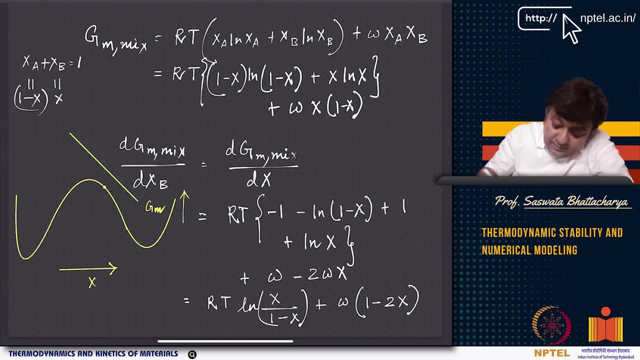 So, then I draw a slope and this slope is basically given by this relation, right. This slope is given by that. So, this is the slope of the curve. So, I can take this point here, I can take the same point somewhere say, say, say, say here, I can take this. I can just take a slope. If I want a slope by couple tangent, then this is the tangent. So, I can do that. So, basically this is the first derivative is the slope of the tangent drawn 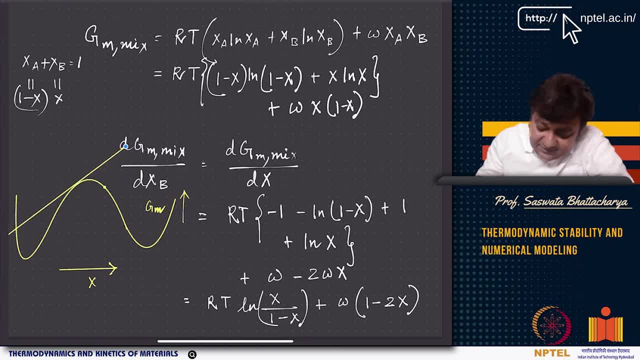 at some composition x. This is the slope of the tangent drawn at some composition x or xp, ok. So, that is the first derivative and see the first derivative. And if you can understand this, so basically if you can have a look at this, but you see, so this is exactly what I want to tell. There are some points where the slope becomes 0. See there is one point where the slope becomes 0, there is another point here where the slope becomes 0 right, you can notice that point. So, this is one point where slope 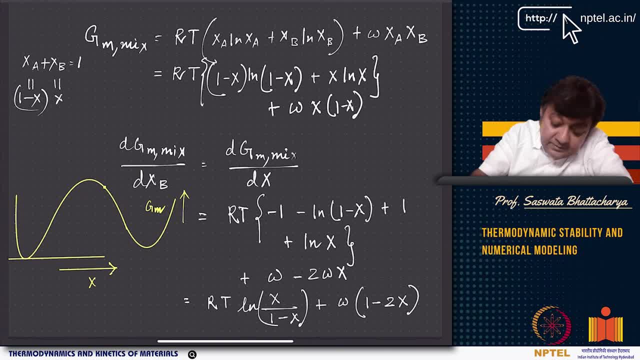 is 0, this is another point, this is another point. So, basically if I draw three tangents like this and this is another point where slope is 0 right, there are three points on this curve where slope is 0. Now, let us let us let us have a look there is something other 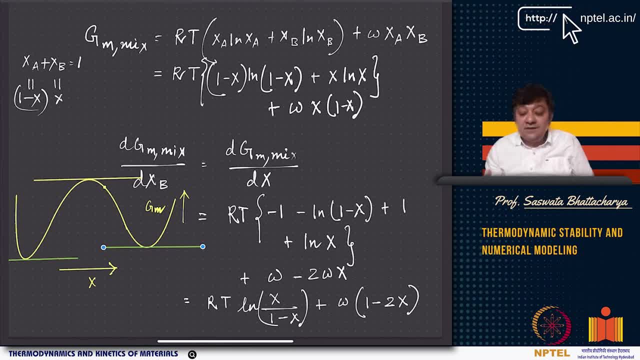 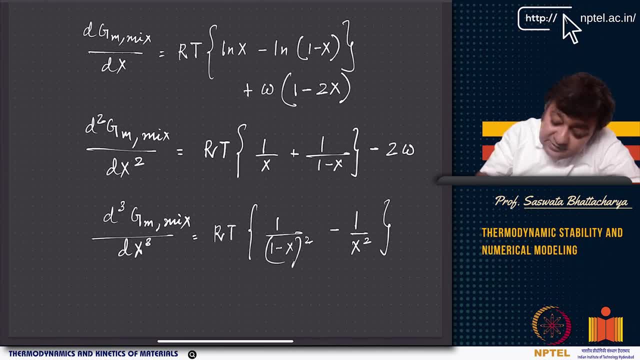 DGM matrix right which is RT, so which have which is RT ln x minus ln minus x plus omega minus 2 x. Remember when you plot this curve when x equal to 0, ln 0 is undefined, when x equal to 1, ln 0 is again undefined. So, as a result when you plot this first derivative right, you can plot the first derivative, you can plot the free energy and if you plot these things, remember to use an axis where the limits are 0. 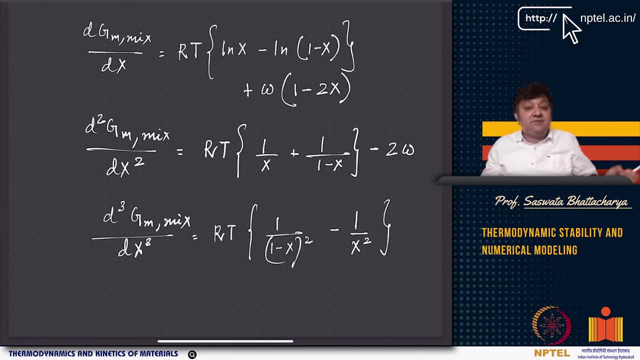 So, that means that between 0 and 1 but not exactly 0 and 1 because that 0 and 1 the logarithmic terms are undefined. Now, have a look at the second derivative, now you have the first derivative so you can go further and you can do second derivative. So, you have RT, RT remains, RT remains and you have now ln x becomes 1 by x and this becomes plus 1 minus 1 by 1 minus x, why because you have a 1 minus x and here you have minus sign. So, ln 1 minus if you take differentiation, so it becomes 1 by 1 minus x with a minus sign outside, so but there is already a minus sign, so minus minus becomes plus, so you have a plus sign, you have a plus sign, note that, that there is a plus sign, right. So, this one has a plus sign here and then you have the third derivative, I go further, I take the third derivative, then you have r t, so if you look at that, you have r t and then 1 minus x whole square, right, 1 minus x whole square, right, right 2 omega, omega is a constant, right. 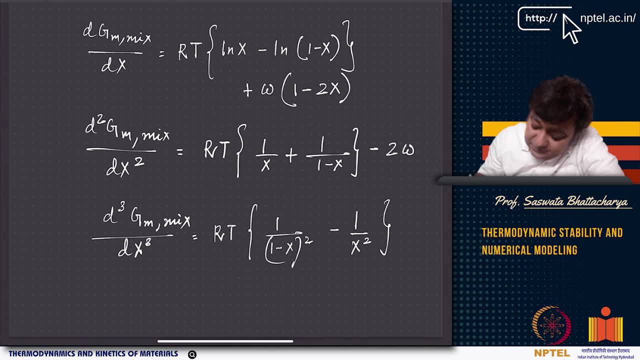 So, this goes to 0, now you have 1 by x square, so minus 1 by x square, see minus 1 by x square, but here it is minus 1 by, so this is 1 minus x whole, so minus of 1 minus x whole square, but there is also minus x here, so this becomes plus. 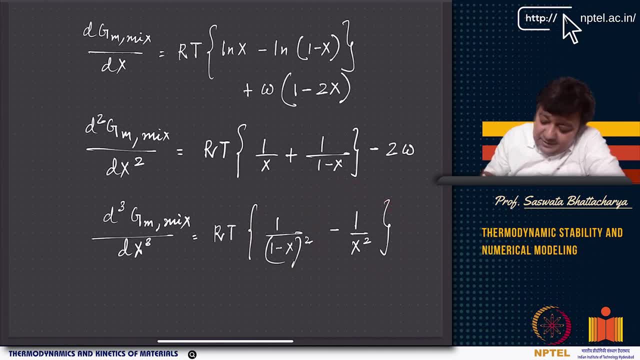 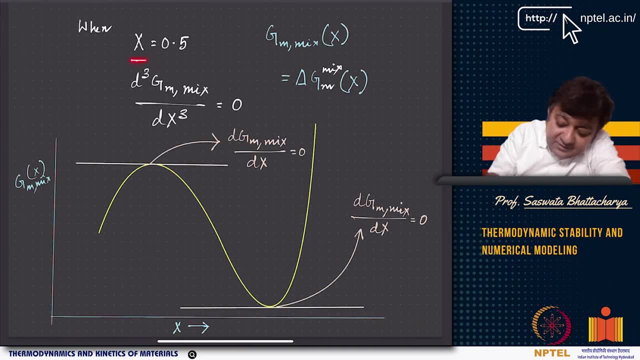 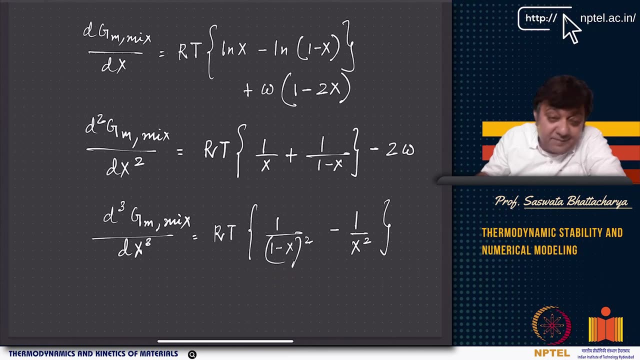 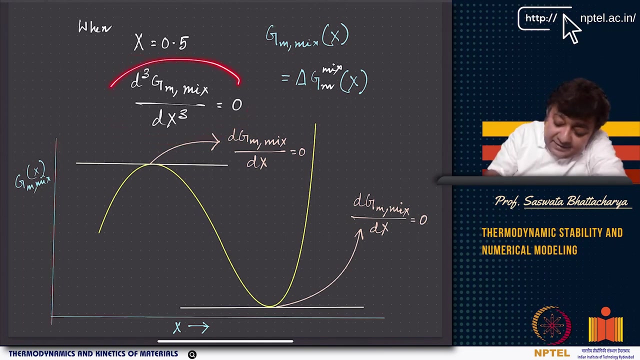 So, plus. 1 minus x whole square minus 1 by x square into r. Now, if you look at the third derivative and basically put x equal to 0.5 now you see you have 1 by 1 minus 0.5 which is 0.5 1 by 0.5 whole square minus 1 by 0.5 whole square. So, at x equal to 0.5 this guy basically becomes 0. Now, these guy if you see if you have d 2. So, basically if you have d 2 g d x square d 2 g m d x square as some quantity say let us call it some some quantity say y. 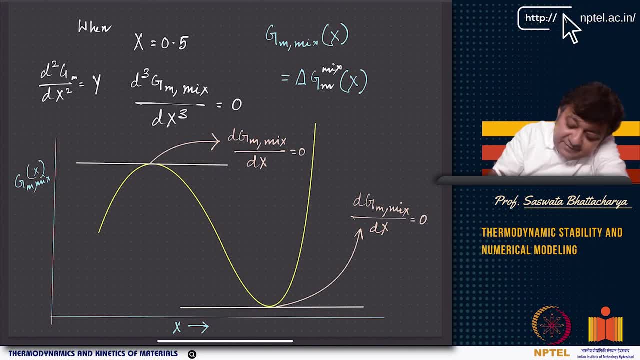 Now, if that is so d 3 this is basically d 3 g m d x cube which is nothing but d y d y. 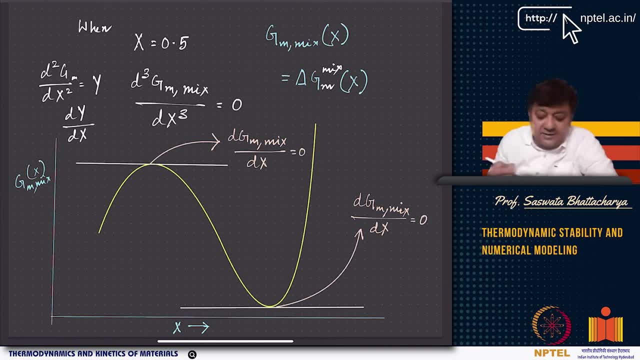 So, basically this is slope of the second derivative right say slope slope of the curve slope of the curve that is of the second derivative right. So, basically now if you look at this 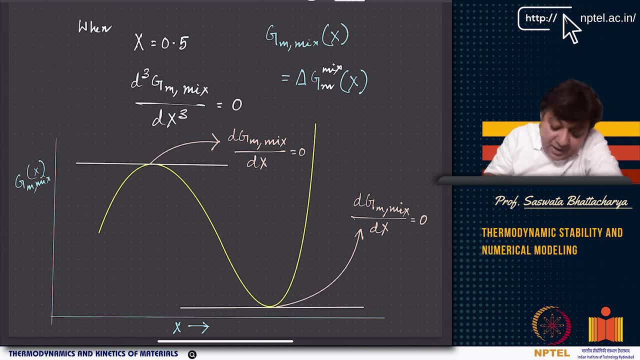 if you look at this. So, you have g m x say for example, you have g m x here. So, you have g m x here and you have one point where the d g m x d x equal to 0 this is the g m 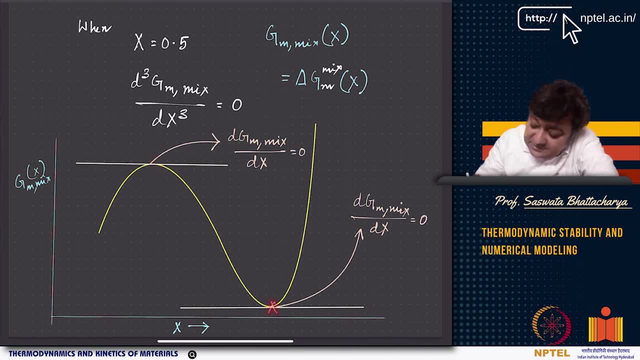 this is one point where it is and this is another point where d g m d x makes d x equal to 0 and these points are basically where the tangent line becomes parallel to the x axis. Tangent line is parallel to the x axis, the slope is basically 0. But when you look at the d 3 g m d x cube equal to 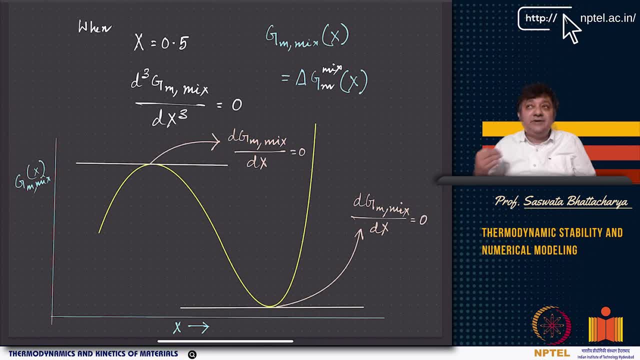 0, then you get a value of x equal to 0.5. What does that really mean? So, basically you have a curve and you have it slope and the second derivative basically represents its curvature, 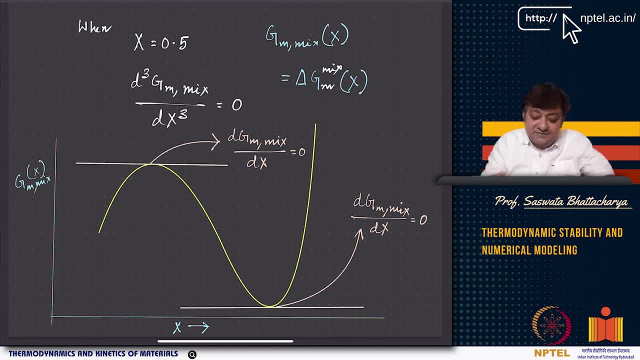 second derivative represents its curvature. Now, if you look at the curvature the second derivative. 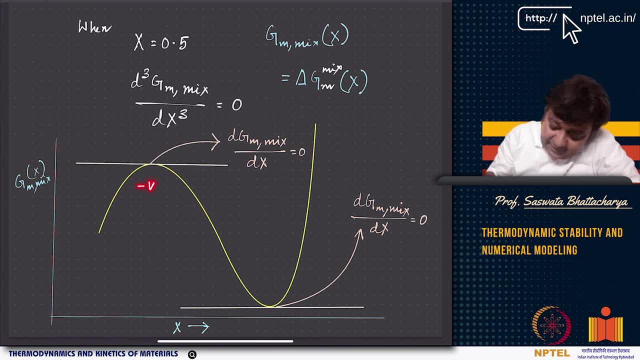 So, in this case the curvature is negative right, in this case the if you see this, this is curvature is negative and this is where curvature is positive. Now, if you see you have a negative curvature here, you have a positive curvature here and the curvature is changing. So, here so, you are looking at this point this point where you are in the maximum so, you have a negative curvature here. Negative curvature means the second derivative is negative means the second derivative is negative means the function is the the the the the the the extremum of the function is a if I have a function f x. If I have a function f of x, if I tell f prime x equal to 0 and I get x equals to x t, Now, I do f double prime x. Now, at x equal to x e, I get less than 0. That means x e is a at x e the function is a maximum right, the function is a maximum. If the second derivative is negative, now the curvature is that means the second derivative is negative means here what we are talking about? Here the second derivative is indeed negative right, the curvature indeed is negative. Here the curvature is positive right, which has a positive curve. 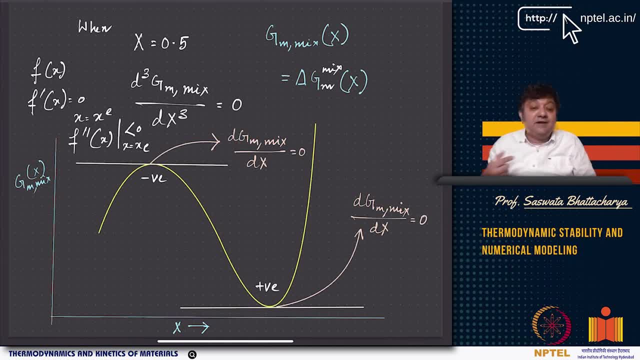 Positive curvature means it is a minimum right, when f double prime x at x equal to x e is greater than 0. That means x e is where the function has a minimum right. So, this is the idea right. So, we are just looking at the same idea. So, basically what we are telling is ok, you have calculated the function, you have you know the function, probably you have for example energy or say free energy, you know the function. Now, you take the first derivative and equate it to 0. What do you get? You get the extremum values. Now, you want to check whether the extremum values indicate a maximum or a minimum. If it is a maximum as you can see, if you remember the ball rolling example, then if the ball is here, then obviously this is basically an unstable equator. However, if it is a minimum, it has nowhere to go right, it is already in the minimum energy level. It wants to remain there. If you can see the second derivative, the second derivative now will be positive. 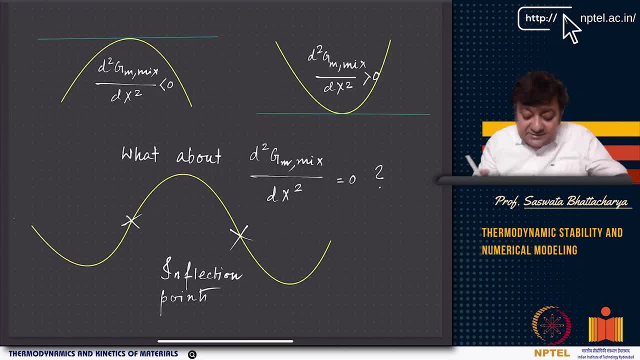 So, positive indicates minimum, negative indicates maximum. We can immediately see that right. So, this is basically the maximum, this is maximum and this guy tells you minimum. So, you have positive curvature. Here, you have positive curvatures, you have positive curvatures, so basically what you have here is positive curvature. That means the second derivative is greater than 0 at the extremum value right. The extremum value is where the slope is basically 0. The extremum value you calculate by making the slope 0 and then at the extremum value, if you calculate the curvature, the curvature is positive. That means there is a positive curvature means it is a minimum okay of the curve, it is a minimum of the curve. Now, again slope is 0 here also right, slope is 0 here also. This is an extremum value. So, as you can see, this is the extremum value. Now, at this extremum, the second derivative is less than 0. Second derivative is less than 0 means this extremum is nothing but a maximum right. In this case, this extremum, this extremum that you have, this extremum, right. 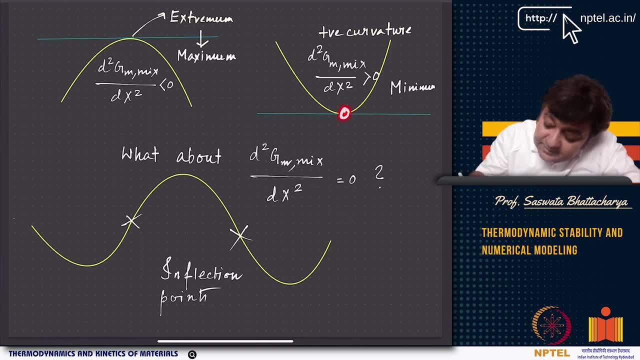 . This extremum is nothing but a minimum right. So, now if you look, if you look at, if you look at this term, so there is also a possibility that the second derivative is 0. Now, second derivative is 0 basically gives you the point of inflection okay. This is called the point of inflection. Inflection is where from positive curvature, you are changing to negative curvature. So basically, you are changing from positive curvature to negative curvature. So, basically, you are changing from positive curvature to negative curvature through 0 curvature. This 0 curvature, so these are 0 curvature points and these points are called points of inflection. The points where the curvature becomes 0, so 0 curvature are the points of inflection. 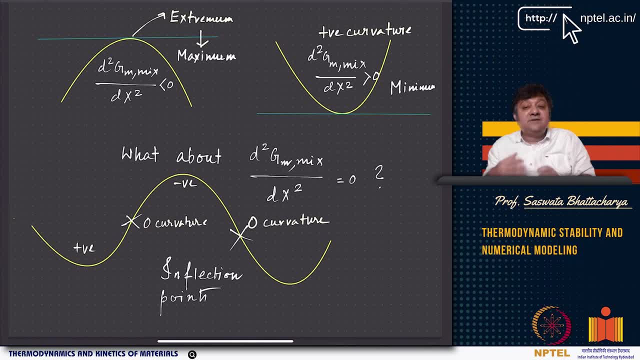 By the way, the 0 curvature points indicate something called as spinodal decompositions. Spinodal decomposition is where you have a oil-water mixture which is homogeneous. Now, you are taking it below at 0. So, you are taking it below at 0. So, you are taking it 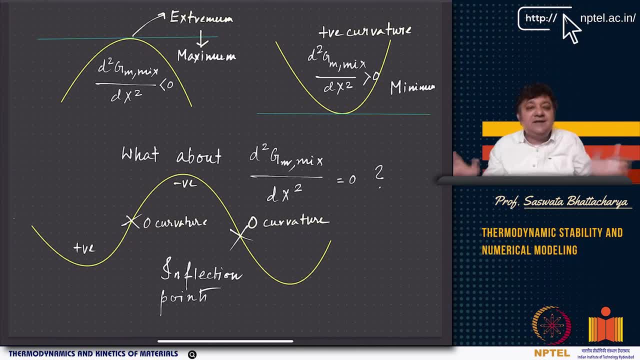 at some temperature which is below the spinodal. It spontaneously phase separates without any change points okay. So, this this inflection points, but what I want to tell you, what 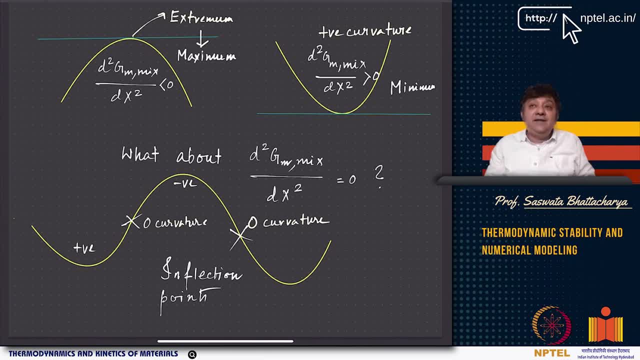 I want to whats I want to emphasize is that, there are these these there, so if you have this type of doublewell potential, doublewell means it has two wells right it has two wells. one well here and one well here right and this energy, I am drawing now as a function of composition. Tomorrow, I can draw it as a function of some water parameter and how parameter. So, now if you see that it has one minimum here, one minimum here, but there is one maximum. So, there is one maximum. Now, if it is maximum then it has negative curvature, this is positive curvature, this is again positive curvature. So, from positive to negative, if I have to travel, I have to go through 0. Now, 0 curvature is where basically it indicates the locus, locus of the points for which, for which any, any energy, any fluctuations, if I have a ball here, any small fluctuation will reduce the energy. See, here the energy 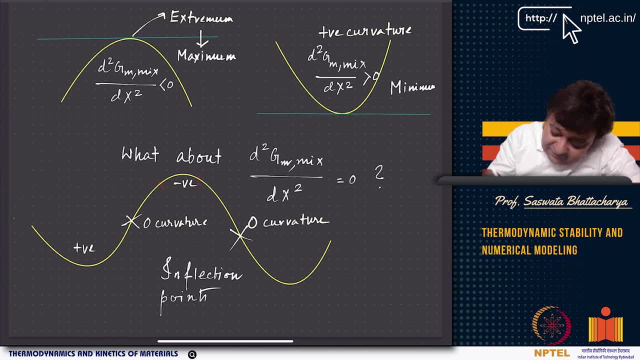 work. Now, the energy is now, if you see the energies, so if it reduces, if I come here, then the energy has reduced, right, the energy has reduced because I have this thing and this thing, so average state I can think of this energy. Now, if you look at that, I go further down, and my energy decreases. So, my energy decreases until I finally reach the common tangent, right, common tangent basically gives me the, the equilibrium states, the two equilibrium states that I reached, that is the double well, that this well and this one, right. So, this is right. 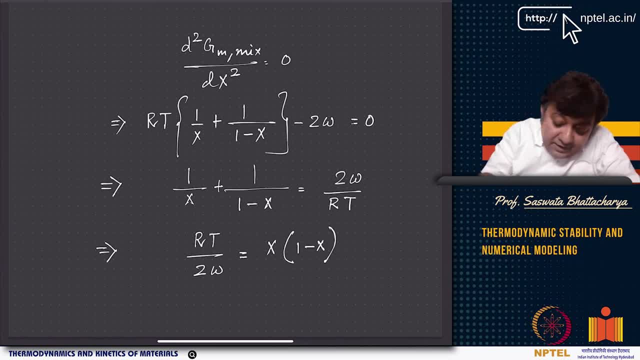 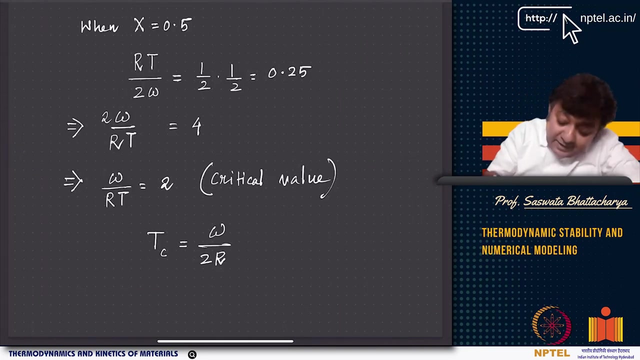 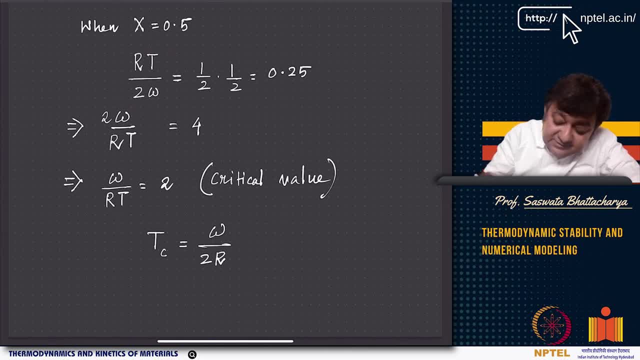 becomes x times 1 minus x, where x equals 0.5 and 1 minus x is 0.5, so R t by 2 omega equals to 0.5 or 2 omega by R t equal to 4, right. If I do the inverse, if it is 0.25, 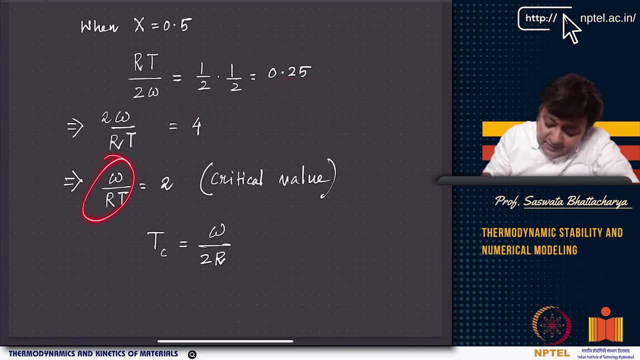 then 2 omega by R t has to be equal to 4 or omega by R t has to be equal to 2. So, now this value 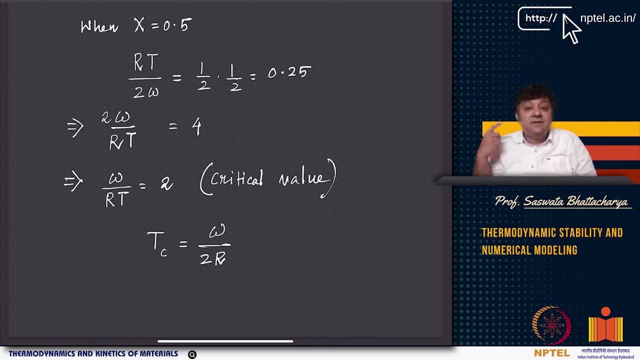 at 0.5, right, at 0.5 gives the, so first we have to understand why 0.5, why did I look at 0.5, 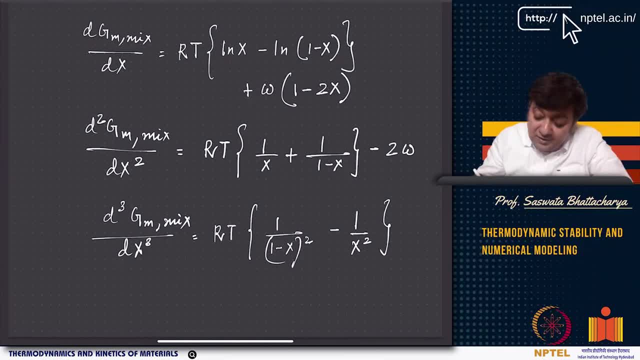 because if I basically use 0.5 in this equation, so what I get ln half minus ln half, which is basically 0. So, this term becomes 0 and this one 1 minus 1, right, 1 minus 2 x, 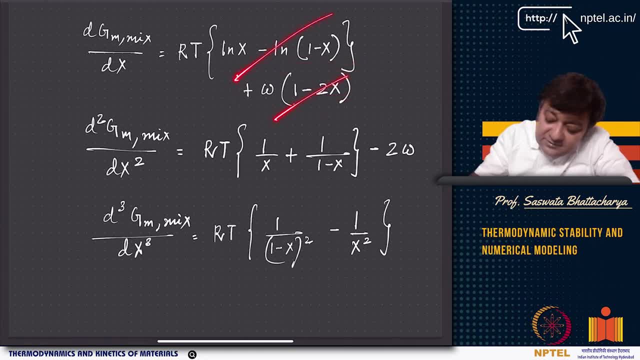 so this also becomes 0. So, this is 0 and this is 0 at x equal to 0.5. 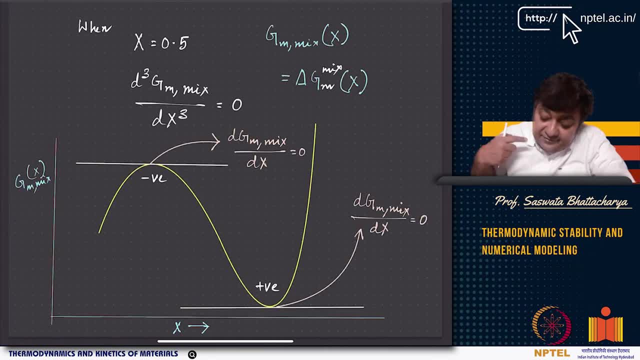 Now, at x equal to half, the second derivative, the second derivative, because with that x equal to half, the second derivative, what happens to the second derivative at x equal to half? It is basically, if I look at the second derivative at x equal to half, what is the second derivative? This is the second derivative, right. So, 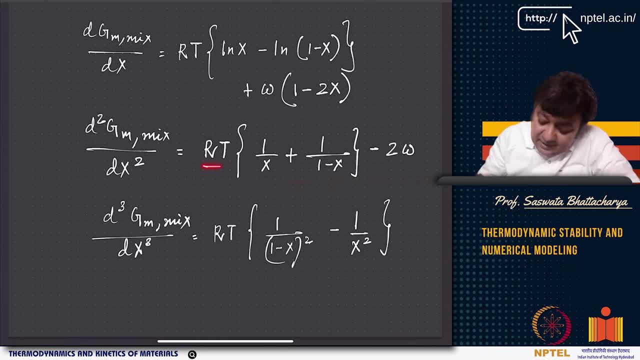 second derivative at x equal to 0.5 is basically R t 1 by x is 2, 1 by 0.5 is 2 and this is 2. So, 4 R t minus 2 omega. Now, this has become 4 R t, 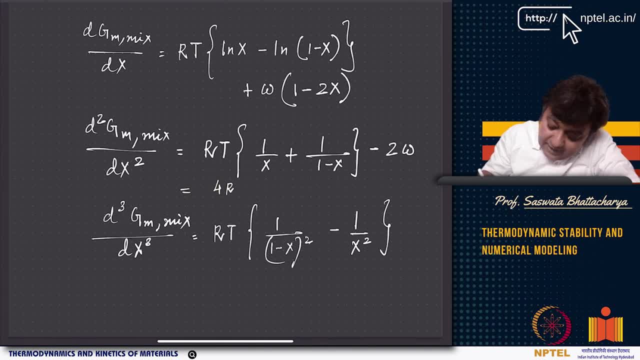 right, 4 R t at minus 2 omega at x equal to 1 by 2, right, 1 by 2, yeah. So, it becomes 4 R t minus 2 omega at x equal to 1 by 2. Now, 4 R t minus 2 omega, if it is negative, 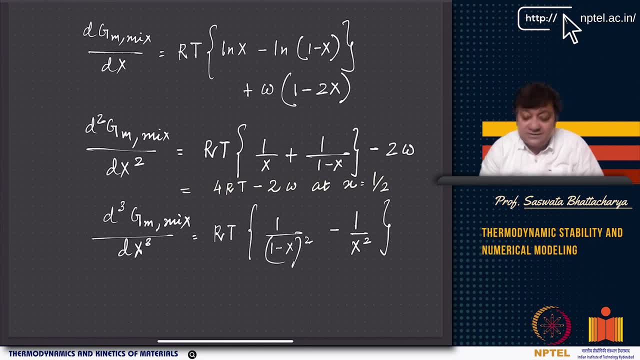 then only, 4 R t minus 2 omega, if it is negative, that means, if 4 R t minus 2 omega has to be less than 0, then basically 2 omega has to be, 4 R t has to be less than 2 omega or 2 omega has to be greater than 4 R t or omega has to be greater than, 2 R t. So, if omega is greater than 2 R t, then basically you will start seeing that 4 R t minus 2 omega is negative, that means, it is a maximum, right, it is a maximum. 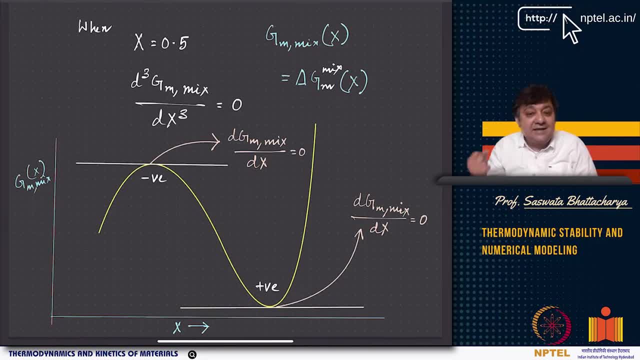 So, the maximum, now at exactly x equal to half, it is a maximum. Now, at exactly x equal to half, if I want to find, if I want to go to t 2 g m d x square equal to 0, which is the inflection point, 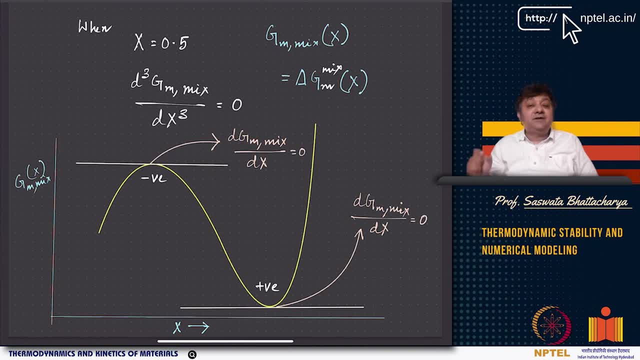 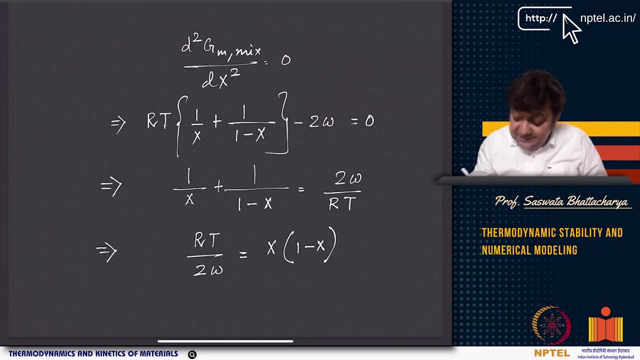 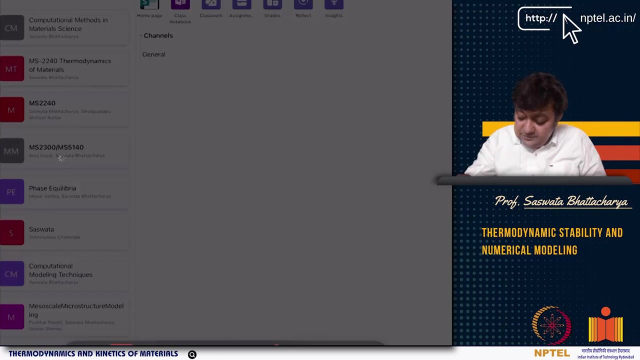 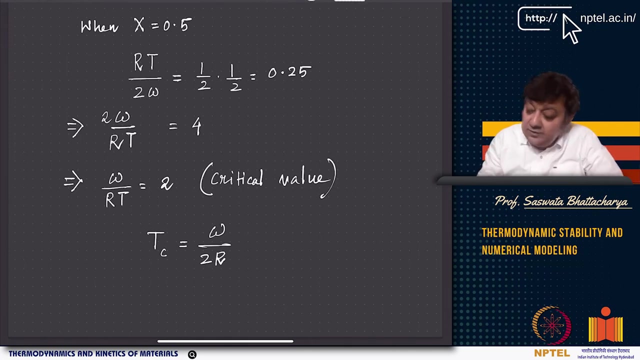 I basically get a very important quantity called the critical temperature, which is t c equal to, t c equals to omega by 2 R, right. We have got t c equals to, comes out to be, so R t by 2 omega will be x into 1 minus x. Now, put x equal to half, so then it becomes half into 1 minus half, which is half into half, which is 1 fourth, right, it becomes 1 fourth. So, R t by 2 omega equal to 1 fourth, right, or 2 omega by 2 omega, R t equal to 4 or omega by R t equal to 2 and t c equal to omega by 2, right, this is the critical temperature. So, if you look at a miscellaneous gap phase diagram, if you look at a phase diagram with a miscellaneous gap, if you look at a phase diagram with a miscellaneous gap, 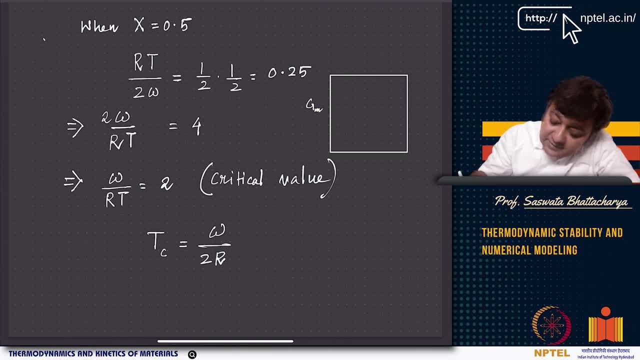 this is my g m and this is my x and 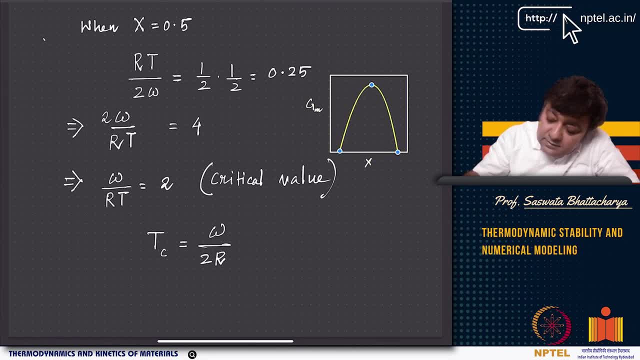 I am approximating it, okay, it is, so if you see, this is your, 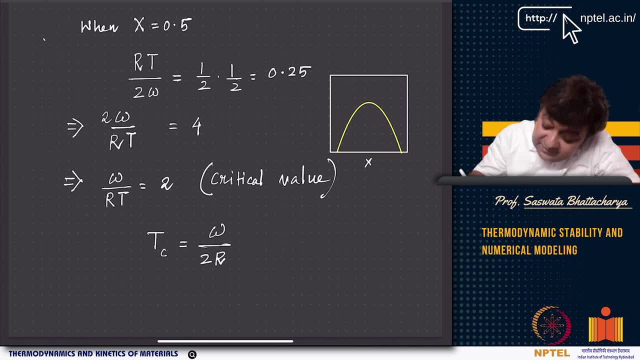 I am sorry, this is not g m, this is basically the phase diagram, so this is t and this is x 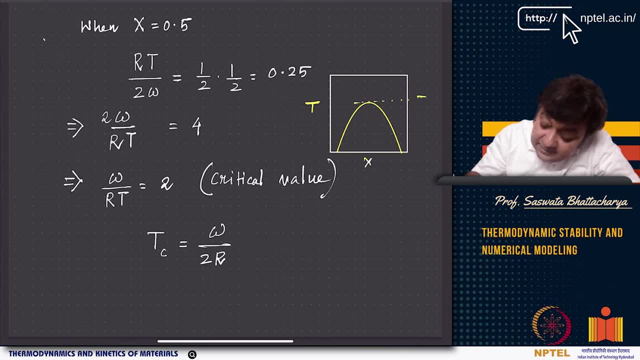 and this point is t c, above t c you have alpha, below t c you have alpha 1 plus alpha, right, above t c you have alpha, and below t c you have alpha 1 plus alpha. Now, if I take, these are the two phases or I 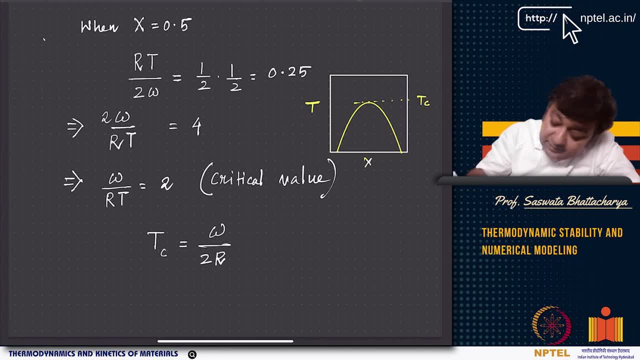 can call this like I have one homogeneous mixture beta and this is beta 1 plus beta. 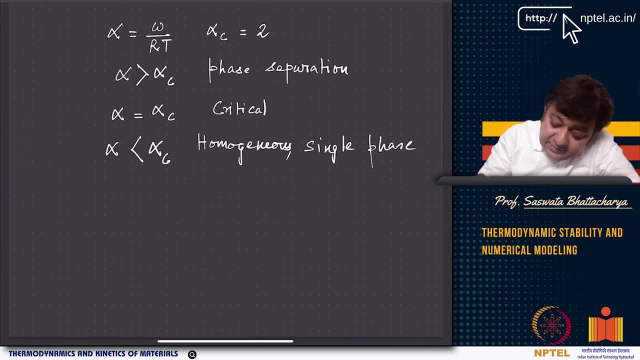 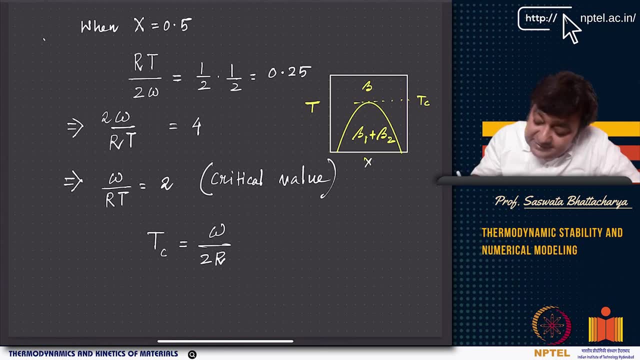 Now, if I tell alpha equals to omega by R t, okay, so that is why I do not want to use alpha because I have used alpha for denoting this parameter, right. So, this beta is basically a phase, right, beta is a homogeneous 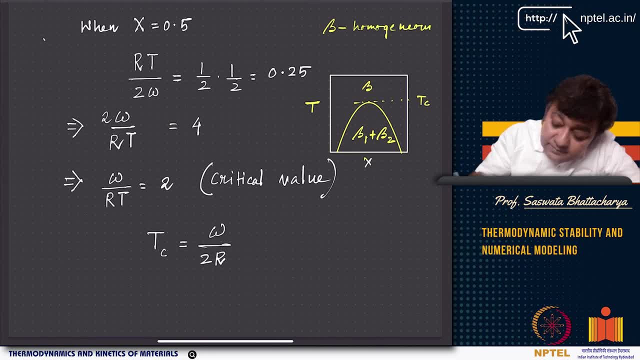 solution and say this is a and this is b of a and b. Now, below t c, once I go below t c, what I see is that beta decomposes into two phases, beta 1 and beta, right, beta 1 and beta, okay. So, there are, so if when you learn about phase transformations, you will see that there are two ways for beta 1 and beta 2 to form. In one case, you have beta 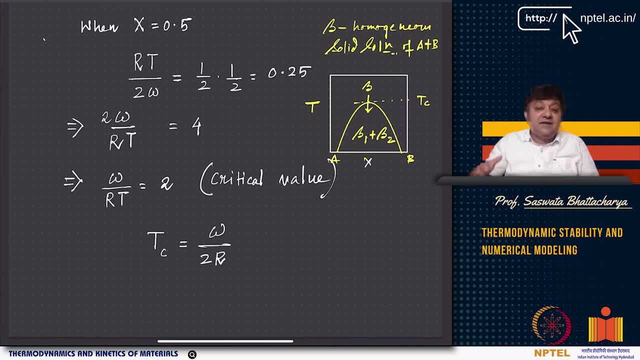 1 matrix in which there is beta 2 nucleation. In another case, the beta for example, at, 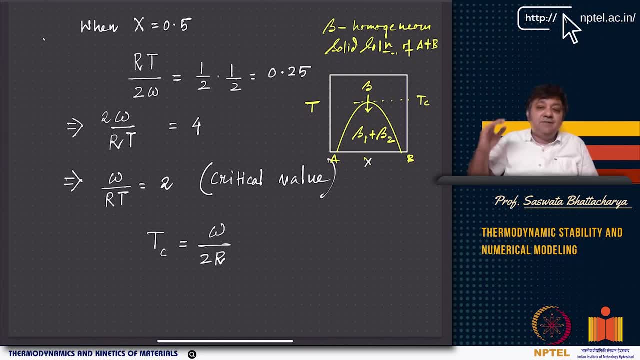 if the composition of beta is 0.5, then you will see that below the critical temperature, beta will spontaneously decompose without any push, without any driving. So, it, it will spontaneous because, why spontaneous? 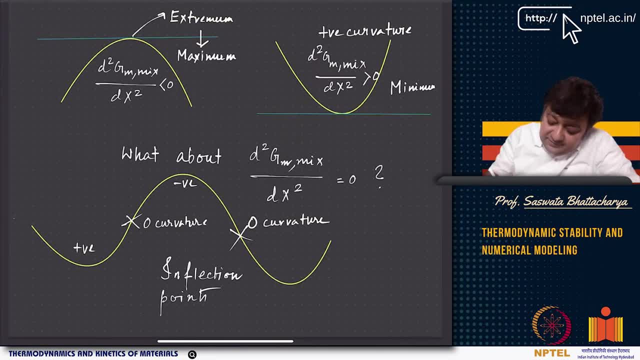 Because if you look at the free energy composition diagram this is what, so, you are here, so again as I told you, you are here and you are getting the . So, what we see is that, this will, so and so, right, the velocity will be interesting whether it will peak here, whether it will peak here. For the free energy composition diagram, then beta is 0.5, because the香港 temperature frequency is 0.7 degrees is 0.3 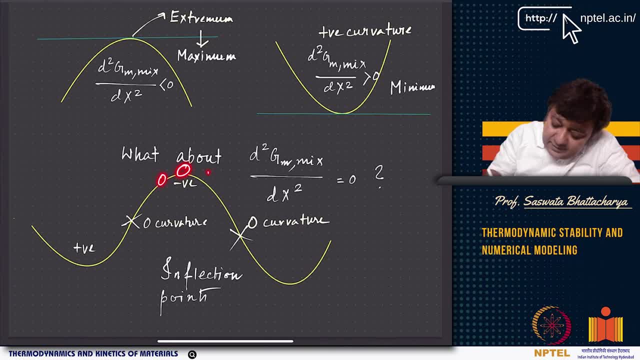 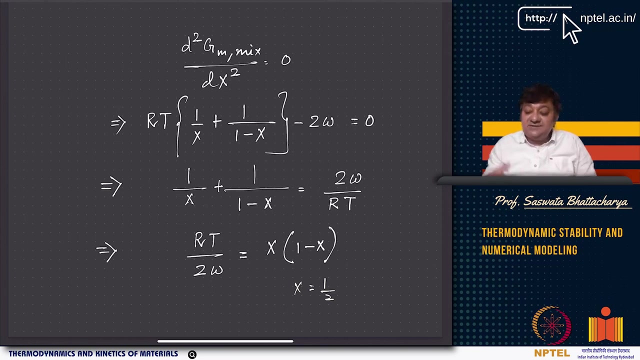 you are here. Now, if you go a little bit here or here, your energy has decreased, right, your energy was here. Now, the energy has come here or energy has come somewhere. So, energy is basically continuously decreasing, ok, if I basically come, if I start falling like this way or and this way, right. So, this is exactly what is the root cause of this spontaneous phase separation. So, if you are within the negative curvature region, even a small fluctuation will lead to reduction in free energy. As a result, as a result, there will be spontaneous phase separation of the slug solution into two phases, right. 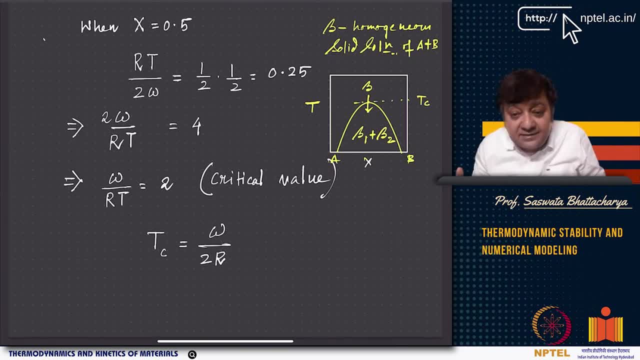 One is A-rich phase and another is B-rich phase. And as you can see here, the diffusion is not, so previous diffusion is down the chemical potential gradient, but it is not down the composition gradient, right. It is not down the composition gradient because if you see, A becomes richer in A and B becomes richer in B, right. 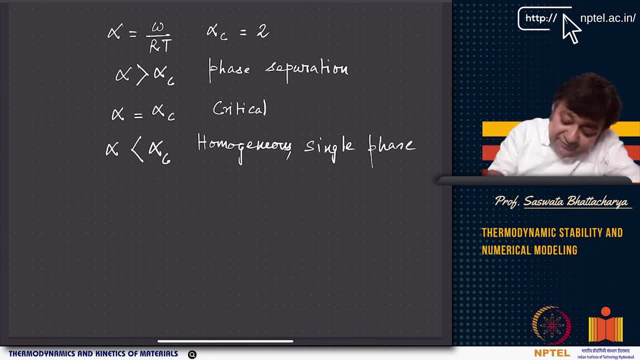 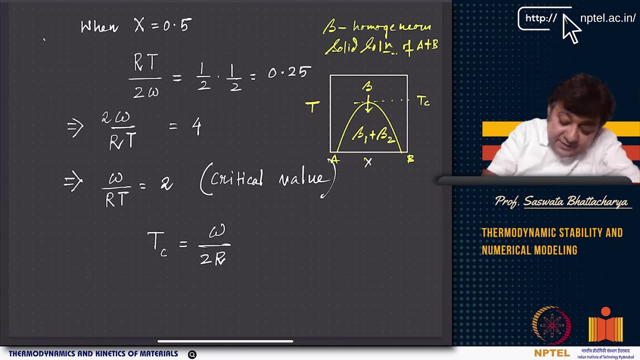 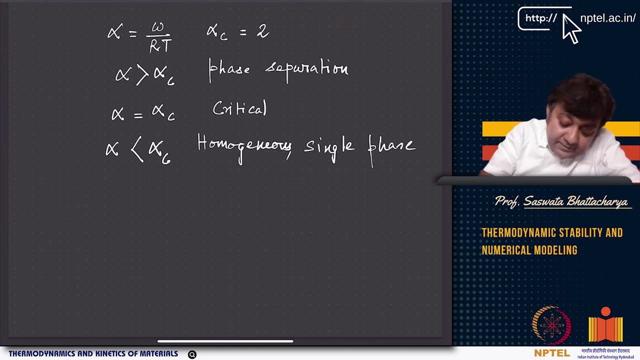 So, this is something that you will keep and look at. So, if you see, if alpha equals to omega by r T and if you see that omega by r T equal to 2 is the critical one, omega by r equal to 2 is the critical one. And from there, you can write T equal to T c when T c equals to omega by 2 r, right. Oh 2 you take this way, T you take this way. So, you get T c equals to omega by 2 r, but you see omega by r T is the critical one. Now, you Now if as I told you if omega greater than RT sorry alpha c is the critical value. So, 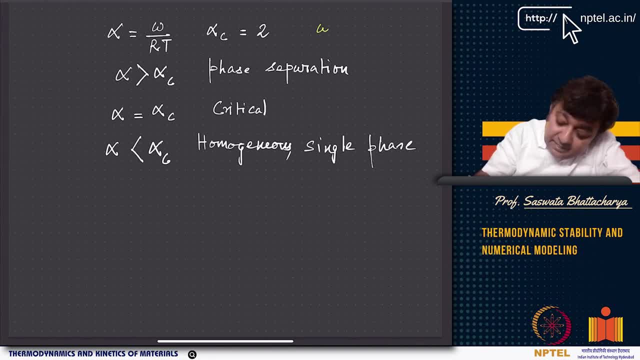 basically if I tell omega by RT greater than 2 or as I told you omega greater than 2 RT then basically what you get is phase suppression right you get is phase suppression. If alpha is greater than alpha c alpha c equal to 2. So, omega by RT equal to 2 is the critical point. So, if alpha is greater than alpha c what you basically get is phase suppression. 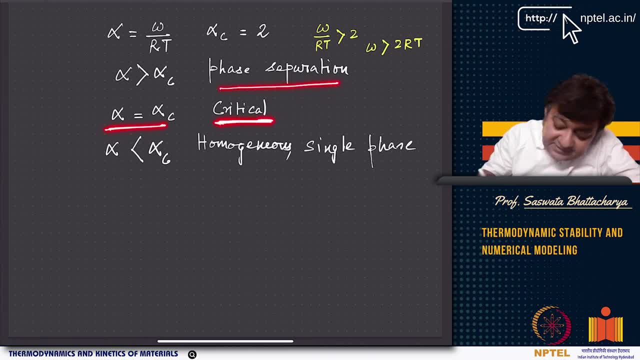 If alpha equal to alpha c you get critical right that is the critical point. So, this basically gives you a critical point. And if alpha less than alpha c right if alpha is less than alpha c what is what what does this mean omega by RT greater than alpha c. Right. So, basically if you see that means omega omega is omega minus 2 RT is less than 0. So, in this case you basically get a homogeneous single phase. This comes again from this right 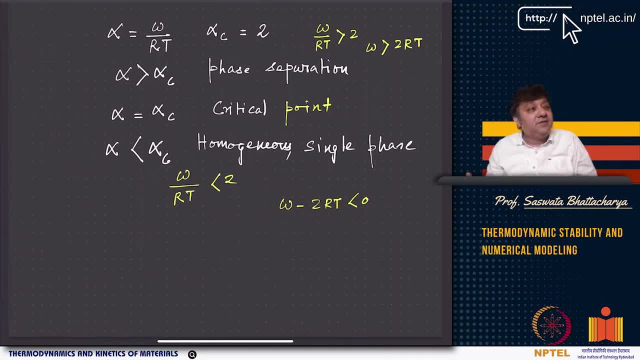 this is no longer a if omega minus 2 RT is less than 0 then basically 2 RT minus omega is basically 0. 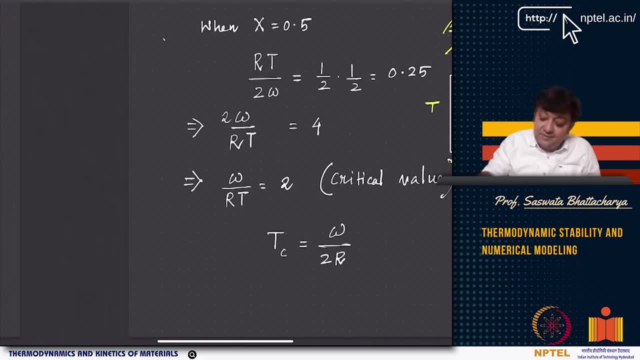 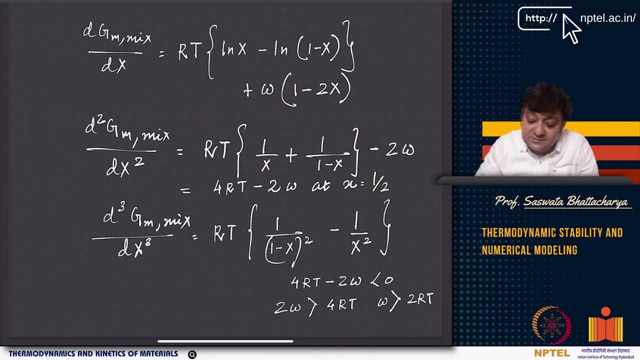 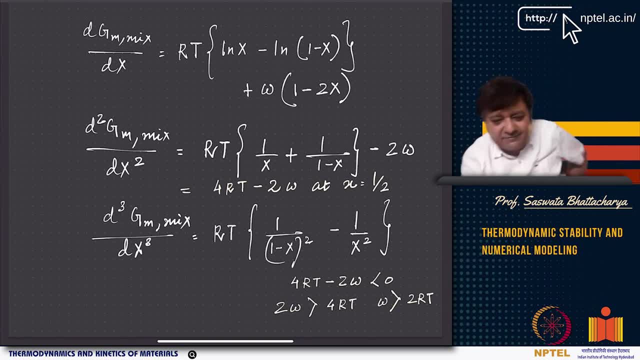 a positive. So, this is the minimum value. If 2 RT minus omega is negative then only 2 RT minus omega is negative means omega is greater than 2 RT. Omega is greater than 2 RT means omega by RT is greater than 2 or alpha is greater than alpha c. Now, if alpha 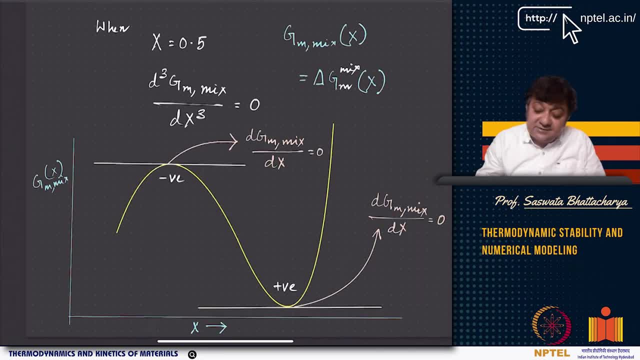 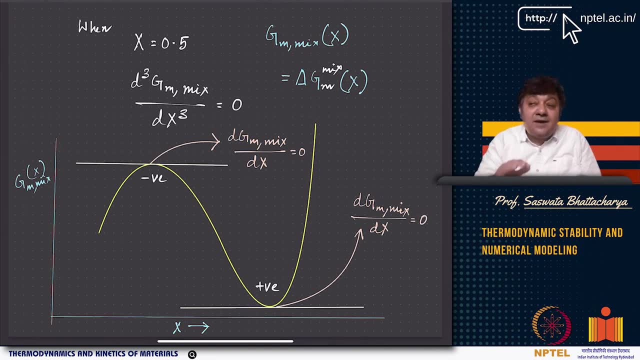 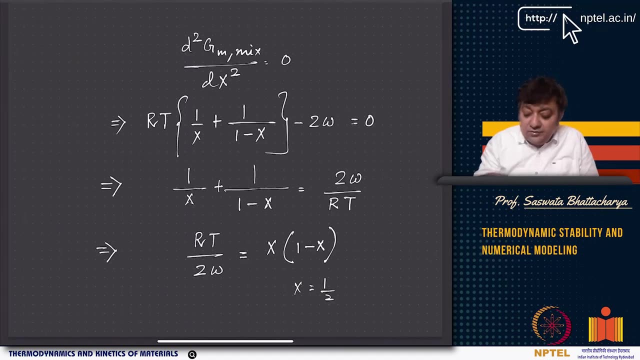 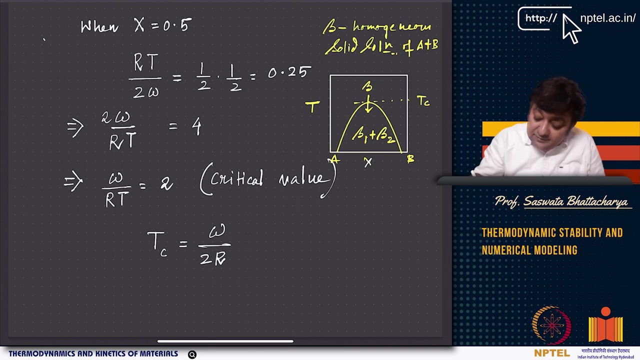 is greater than alpha c basically what you will see is phase separation. Alpha equal to s alpha c you see you basically see a critical point . Critical point is where the beta phase coexist with the beta 1 and beta 2. So, it is critical phenomenon and critical phenomenon your free energy looks a bit like a neutral equilibrium. So, basically it becomes a bit degenerate and what you basically see is something like this. So, if I draw, so it becomes much much flatter right the energies become much right as you are approaching the T c the energies become start becoming flat. So, at one point at T equal to T c you have some sort of a neutral equilibrium any state is possible right you cannot really apply the normal way of applying phonemics. So, you use something called there is a new there is a branch to understand the critical phenomena ok. So, the understand the critical phenomena where you use some other most of the statistical mechanical theory to understand that critical phenomena. So, so at the critical value basically you are telling. 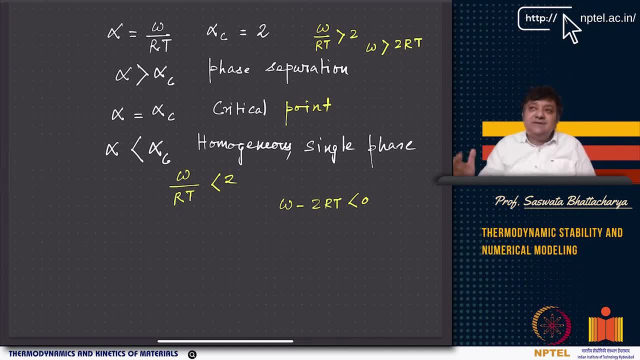 That is a critical point where you cannot basically tell what is means what is the state of the system whether it is a homogeneous state or it is a phase separated state you cannot really tell because all have become all of the states have become degenerate right. So, that is the idea. 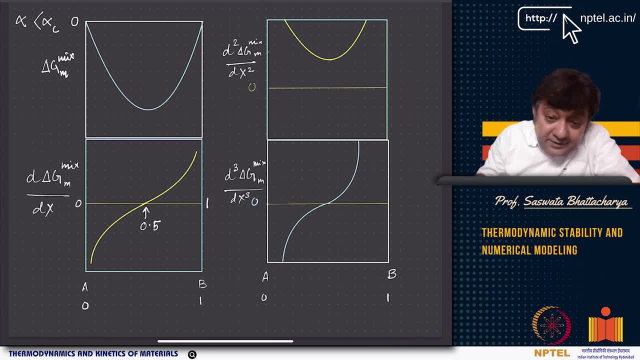 So, if you look at that if alpha. So, if I if I want to plot it if you see if alpha is less than alpha c what you get is a minimum right what you get is a minimum. So, alpha is less than alpha c. So, alpha is less than alpha c and if you look at that this is how your free net does first derivative looks like and as you can see it intersects the x axis at 0.5 correct 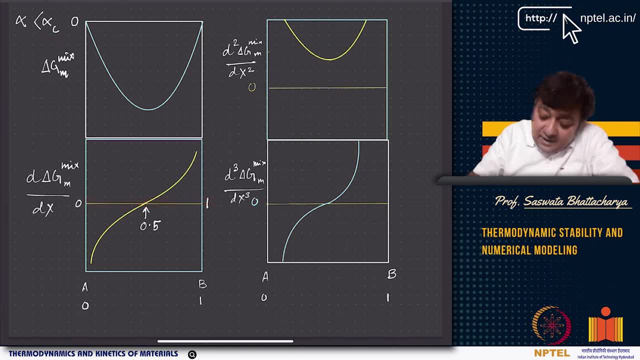 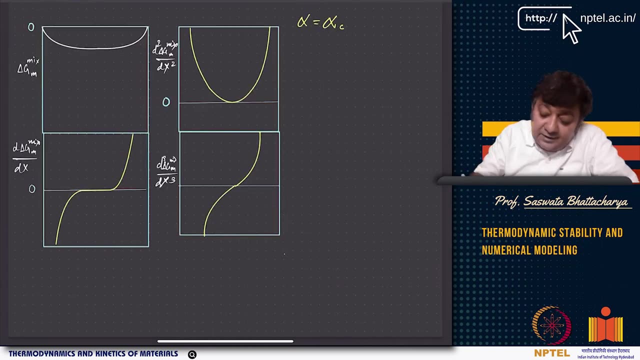 when alpha is less than alpha c. And if you see the second derivative second derivative looks this way and the third derivative again looks this way again with a value at 0.5 right again with a 0.5 right this is the your at 0 line right. Now, if you look at alpha equal to alpha c you see again as I told you it is not very flat and you have this type of a curve where you see it extends right, it is like it is not exactly 0.5 it can be here it can be here right. So, this is like these are the points like it varies between 0.21 and 0.79 by the way this basically defines your negative curvature region right, this is between these two points it is not exactly 0.21 and 0.79 in this case. So, you can basically 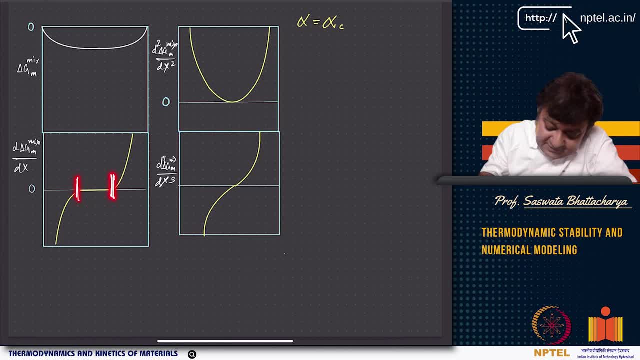 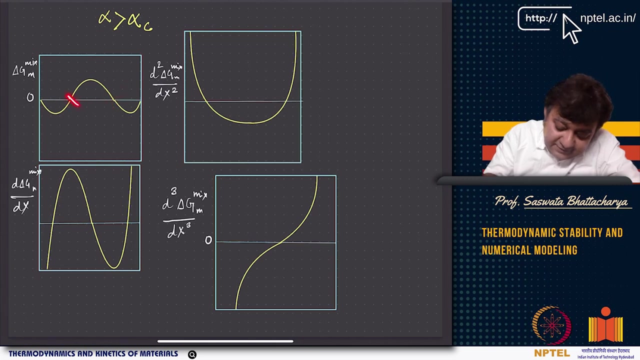 calculate what are the these values these two end points basically tell you the confine of the negative curvature. This is the negative curvature as you can see here that you have this curvature value here where curvature value is 0 here and then the curvature value increases right. So, basically if you look at this critical phenomenon it becomes slightly interesting here. It becomes very flat line here the curvature becomes flat line right you can see the curvature here right if you are saying g m x here. So, it becomes a x right and then you have obviously the alpha greater than alpha c where you have this intersection points right where the second derivative basically goes to 0 and then you have a maximum and you have two minima and if you look at this this plot you have one root here right this is x equal this is basically y equal to 0 or d, so, this the slope right slope of the curve becomes 0. So, slope of this curve becomes 0 here the slope of the curve becomes 0 here here and here, so that this are the corresponding groups right. But at these two points and these two points you have minima this point corresponds to this point, this guy corresponds to this point, and this one corresponds to this point. 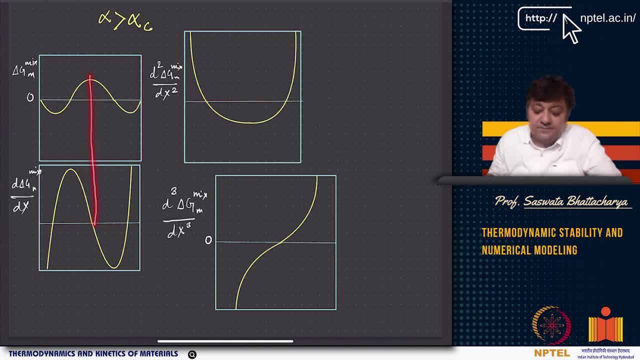 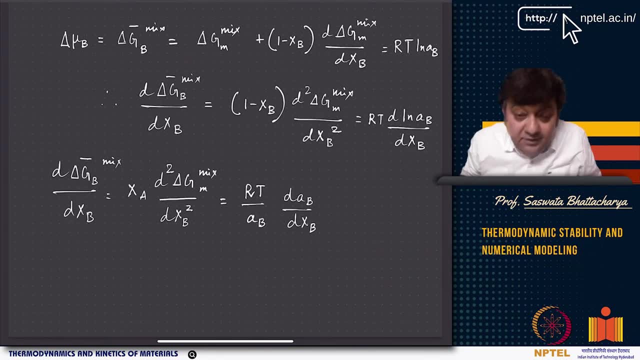 Ok. So, similarly you have the third derivative here and the second derivative here, right. 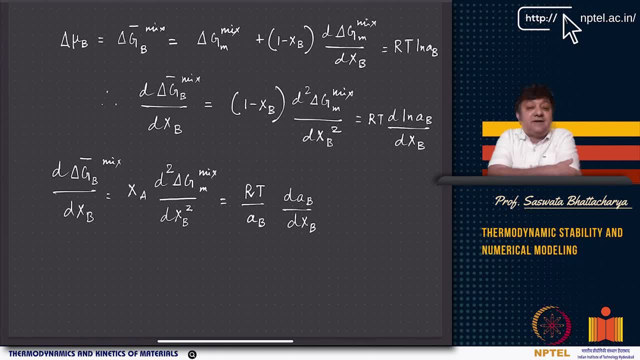 Now you can also calculate delta mu B, delta mu B is basically nothing but mu B solution minus mu B solution minus mu B pure, right mu B pure state. So, basically if you look at delta mu B, delta mu B is basically delta G B bar mix, right. This is the partial molar viscous energy, but this is the partial molar viscous energy of mixing. So, this basically equal to delta G and mix plus 1 minus x B d G delta G and dx B. You can look at the previous partial molar quantities lecture and you can basically see this is what we have written and if you if you calculate simplify then you will basically get this guy because it is a difference between mu B minus mu B 0, this is nothing but a partial molar equals to RT ln AB where AB is active. Now, unlike an ideal solution model where AB equals to x B, here AB will be different, right. And if you look at this first if you look at the first derivative again you get 1 minus x B d 2 delta G B x square and this becomes RT d ln AB dx B. Now, if you do the if you do the second derivative basically what you get is this RT by AB d AB dx B or d ln AB dx B. 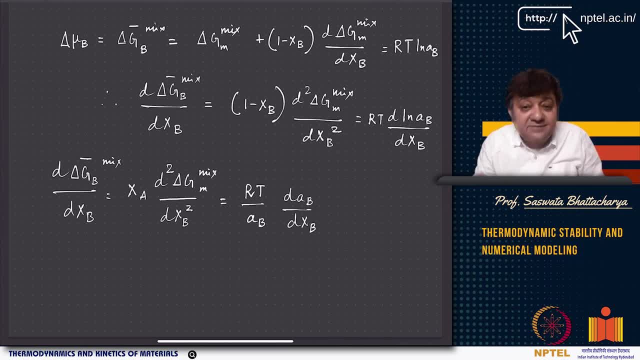 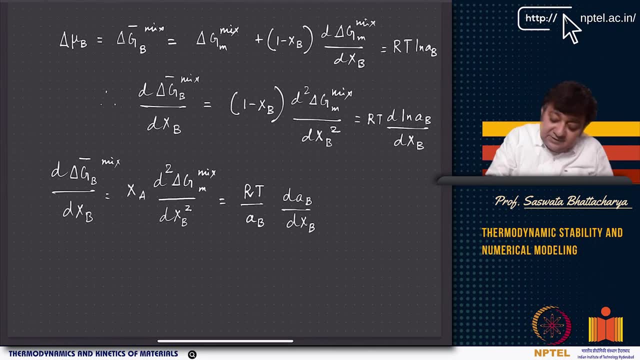 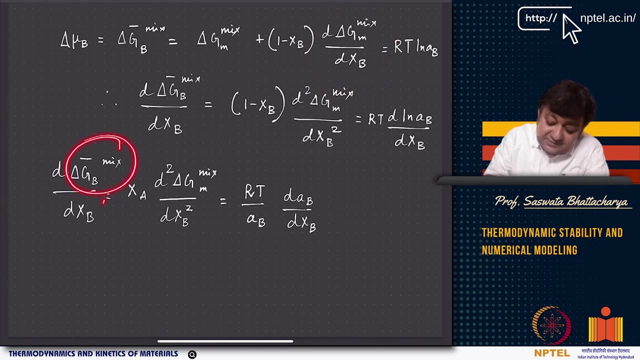 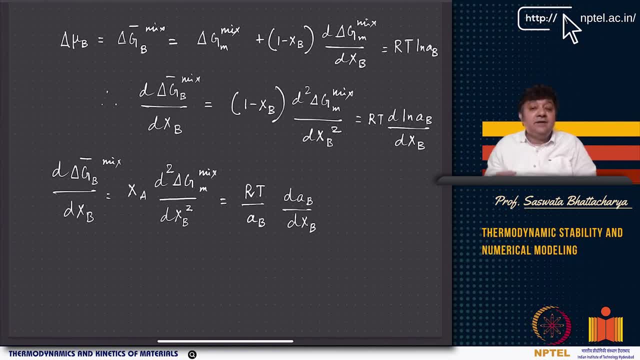 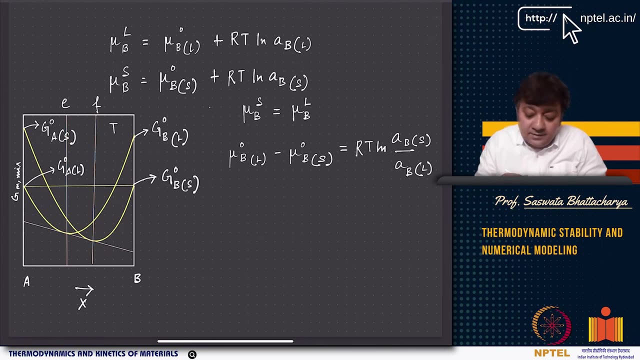 So, basically as you can see here you can calculate the partial molar partial molar quantities of mixing or partial molar potential of right partial molar chemical potential for mixing right for the for the element B as well as for the element D right. 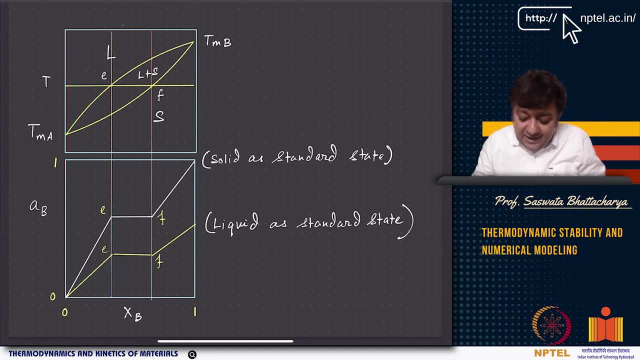 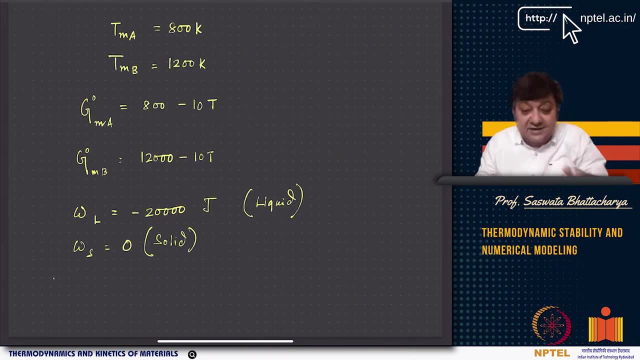 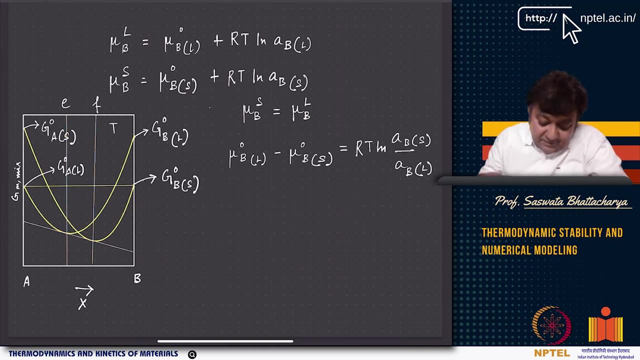 Now basically what I want to say is that there are as you know already and we are we do not I do not want to again discuss because I have already discussed the standard states ok. So, if you look at that if you always have the standard states you can use any standard state as whatever possible. However, this is something that I wanted to tell you because 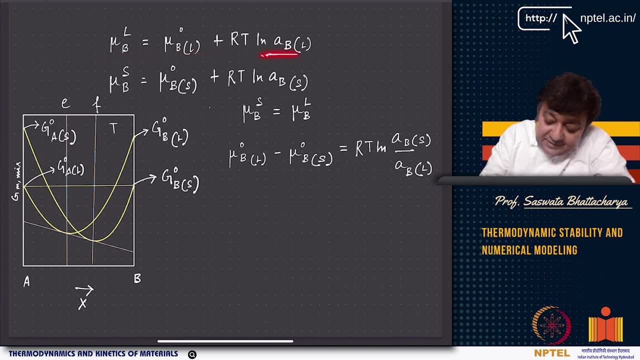 when you look at regular solution models instead of x B right more in most of the cases we have been using ideal solution model so far. 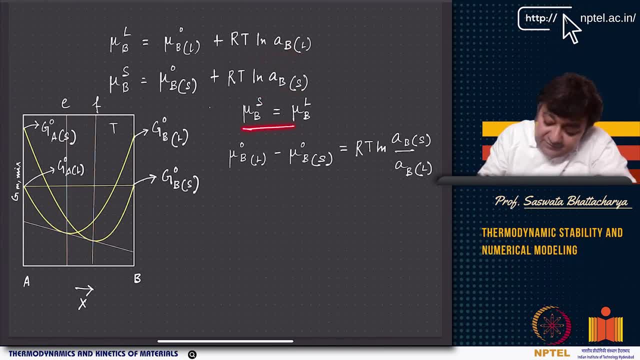 . But, if you look at regular solution models you can also use regular solution models like this, but you have this like mu P S because mu B L because this is your this is your solid this is your solid free energy right this is your solid free energy and this is your liquid free energy right. And if you have that so you are seeing that this guy minus this guy now this has to be equal to this, but you have this part and this part. So, basically this equal to this this minus this equal to 0. So, this becomes RT ln AB by AB solid by AB liquid right AB solid by AB liquid is basically if you take the other way. So, this becomes liquid minus right this is the pure B pure B liquid to solid. So, this is solid to liquid. So, this is solid to liquid transformation or melting right. 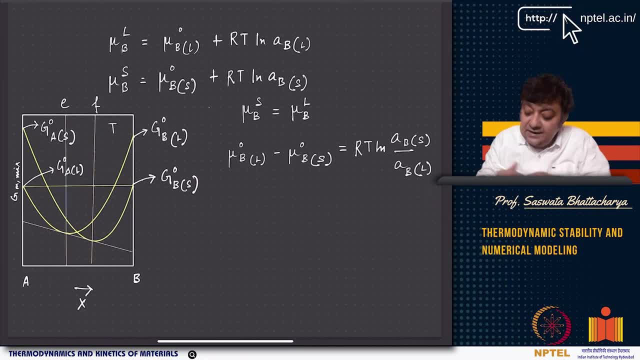 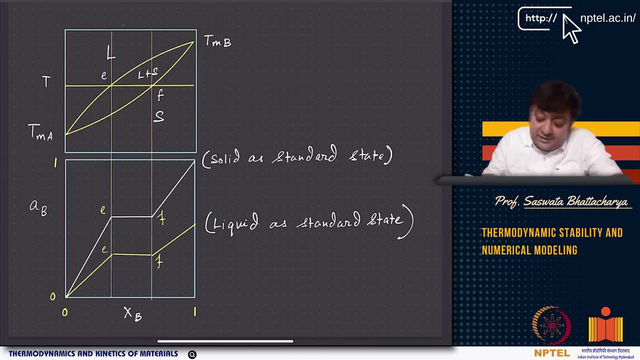 So, this is the transformation now this is basically again comes as a ratio of the activities right in the solid state and the liquid state. Now, if you look at that so only thing that I want to tell that you can use solid as a standard state or a liquid as a standard state 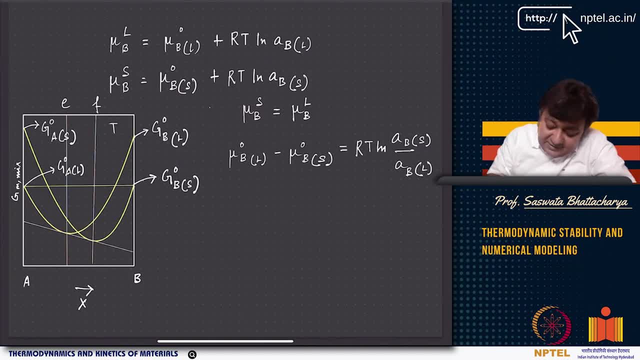 does not really matter the tangent construction does not change the tangent construction does not change the common tangent construction does not change that means the equilibrium values do not change whether I am using this one or this one that really does not matter. 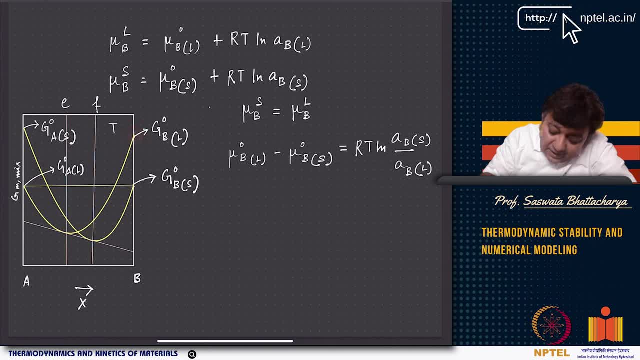 As long as I am consistent that I am taking B liquid as the pure as the standard state and A also I am taking the A also I am taking the liquid as standard state or A for A I can take the solid as standard state while that for B I can take the liquid as standard state or vice versa. But whatever I take whatever I take the tangent construction which basically gives me the equilibrium compositions and all that do not 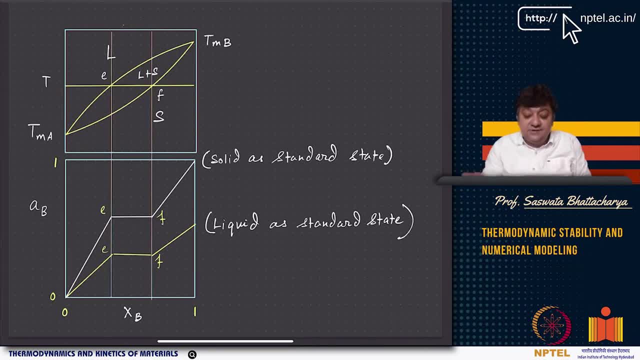 change right that do not change. And if you see the activities if you look at activities and if you look at if you think that I actually I am taking the liquid as the pure as the standard state. So, I am taking that activities same is based based on the mole fraction take the as you can see this activity and mole fraction you have a slope here. But as soon 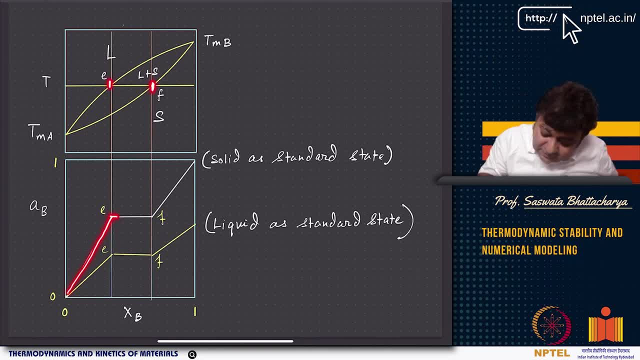 as you go to the two phase region right this two phase region E F in E and F here you basically see there is no changing activity. Again the activity changes in the as soon as you see the as soon as you cross F right you are in the solid state right. So, basically it becomes solid. 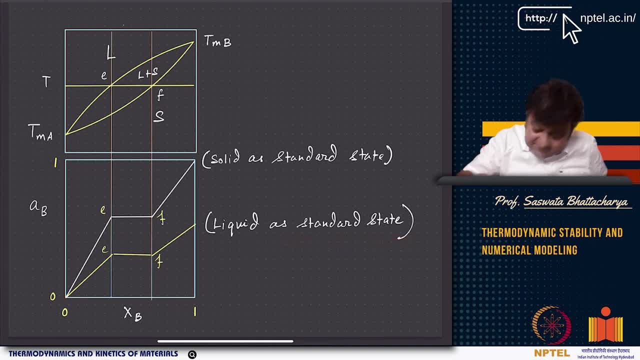 So, you take liquid as standard state what happens you go liquid is standard state. So, basically again you are reaching E you are reaching E and then you have E F where you have the activity constant and then from F you are going to the solid state right from F you are going to the solid state. So, it does not really matter only thing that matters 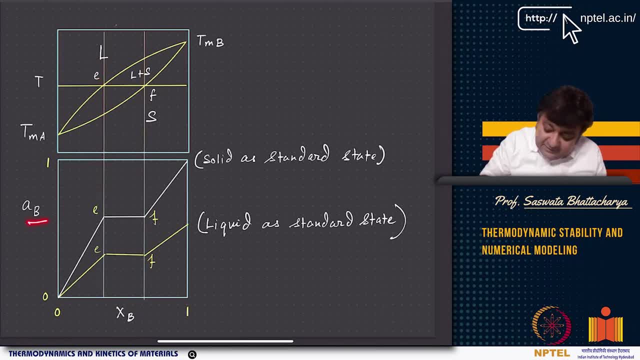 is. So, E F nothing changes only thing that matters is the activity is the activity. So, If I do it with respect to the solid as standard state activity goes to 1 right because the solid is the most stable state at the in the most stable standard state. So, that is why 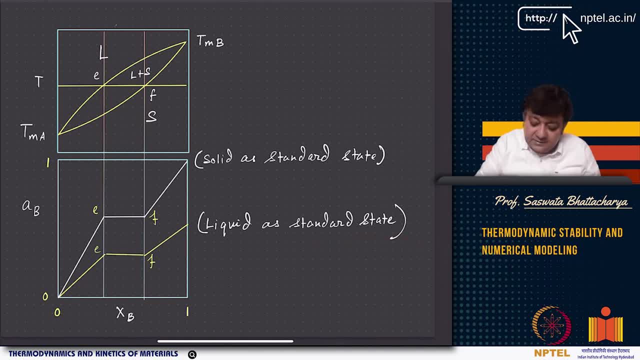 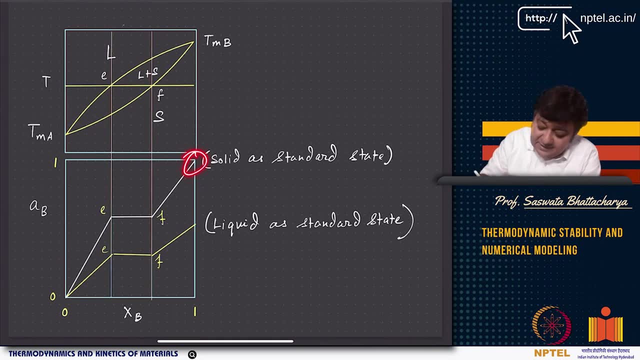 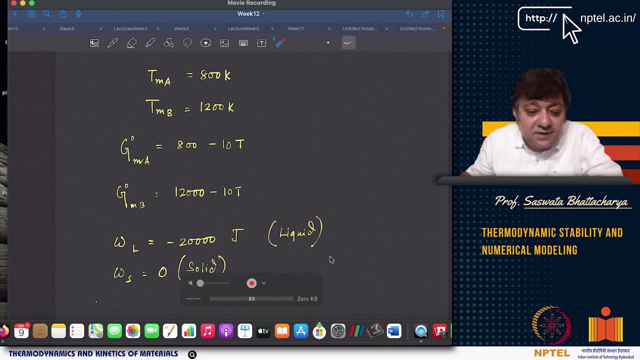 the activity goes to 1, but here if I take liquid as standard state then the activity is not equal to is not equal to the same as x B, but if I take solid as standard state it becomes exactly equal to it. Now, I will just show you so all these things I can basically model. So, I will try to find quickly tell you how to model this. So, if 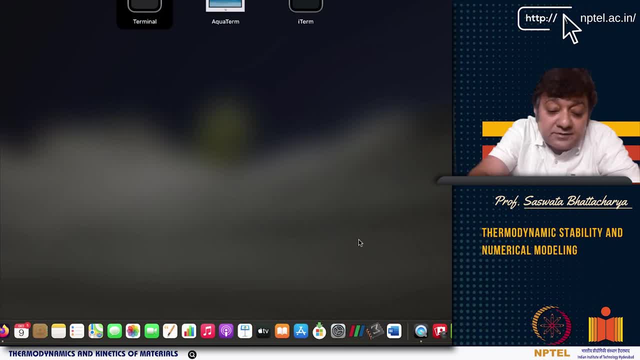 you just open terminal I will just open terminal and show you how to I model this stuff. So, 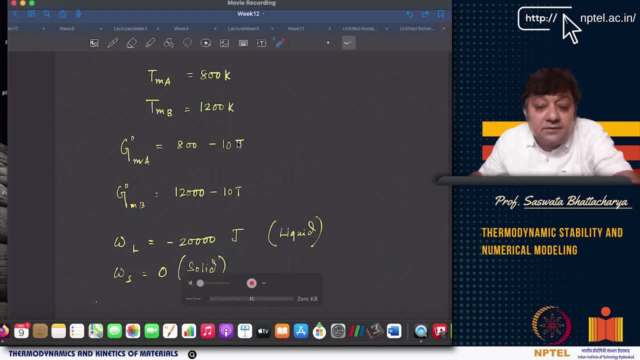 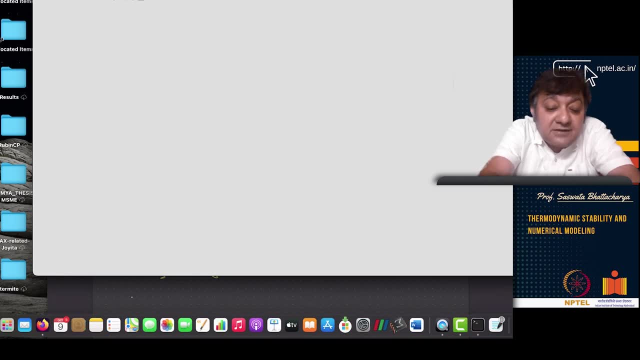 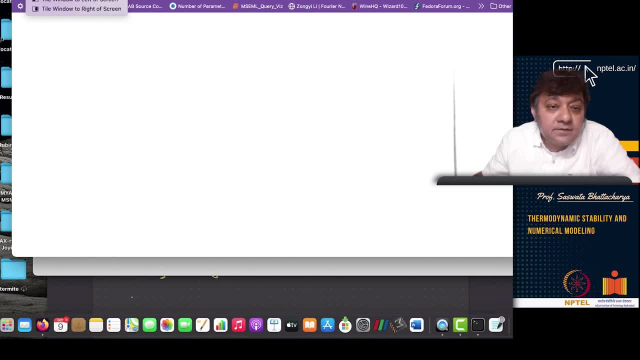 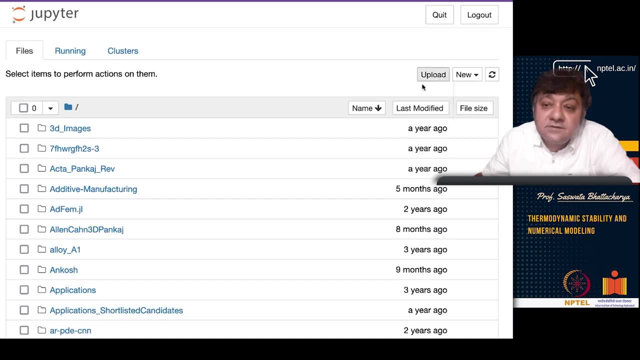 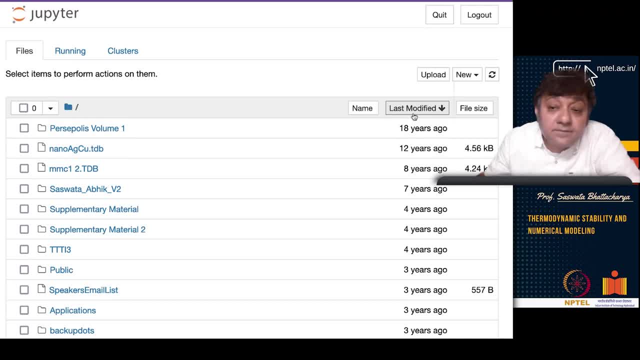 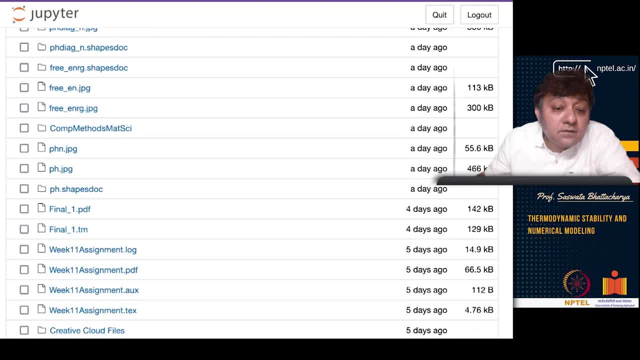 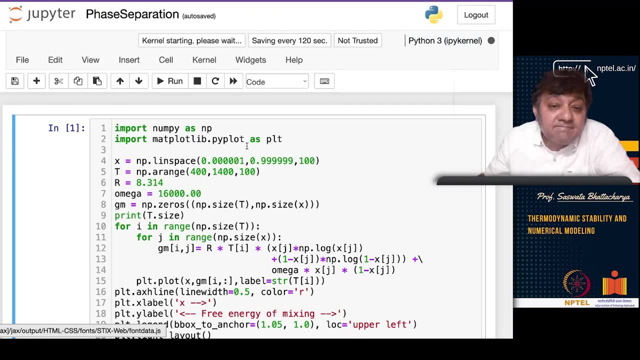 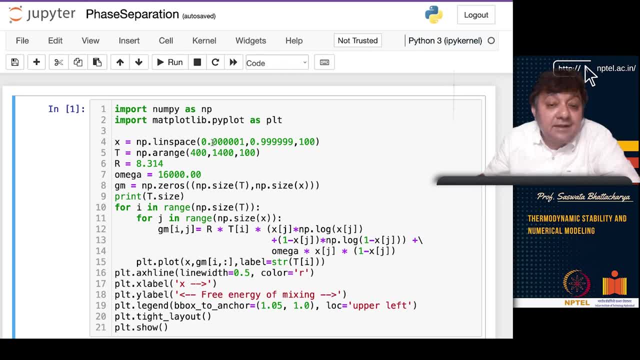 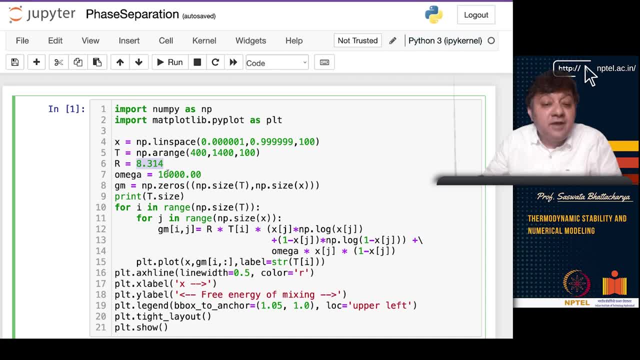 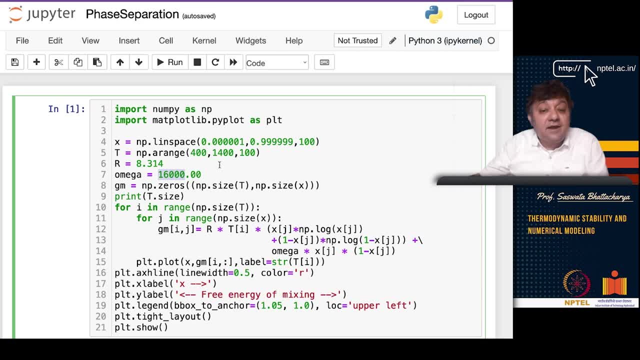 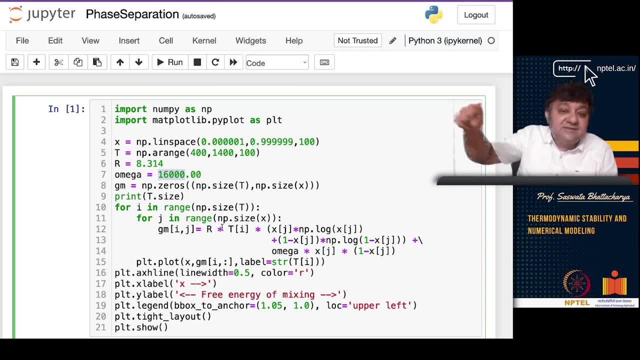 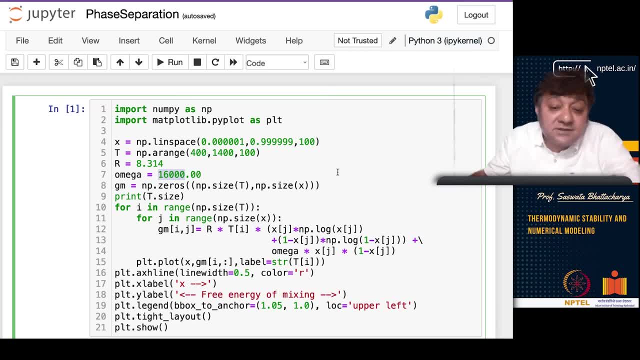 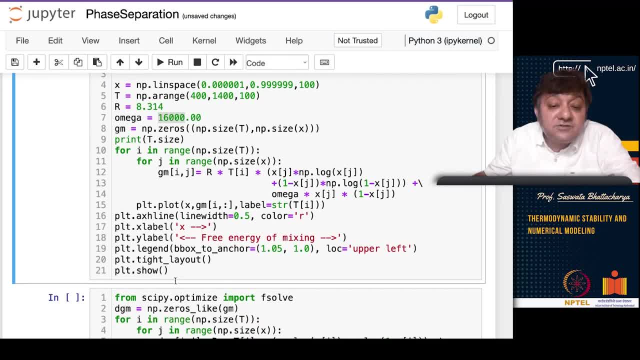 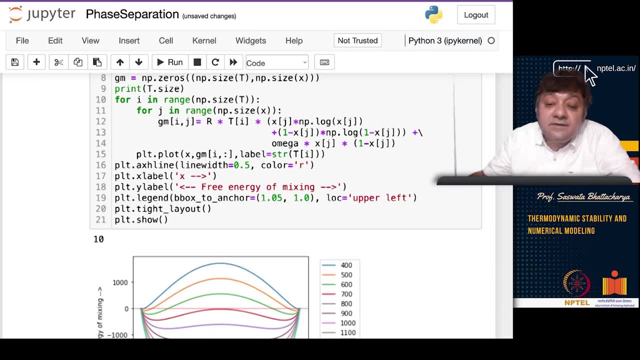 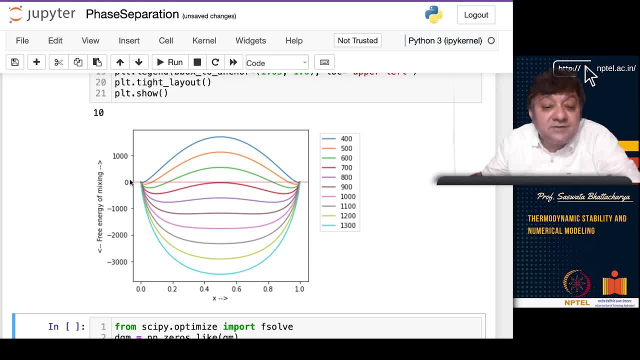 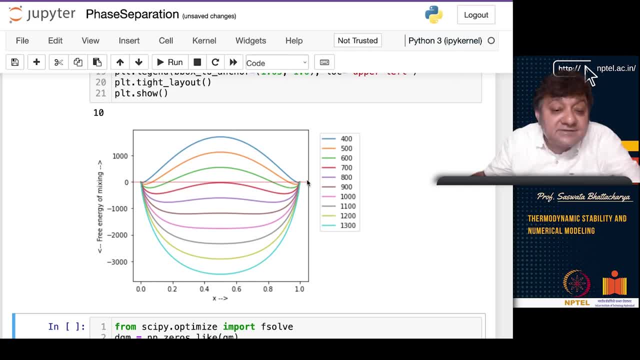 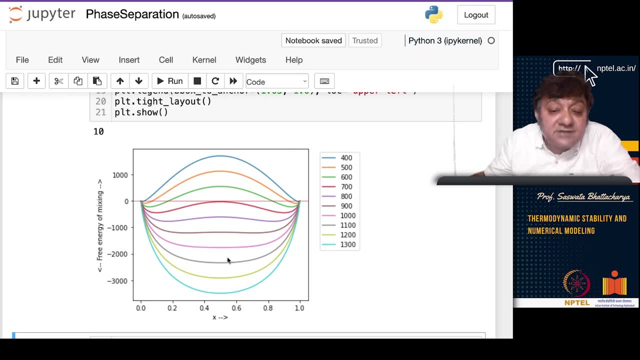 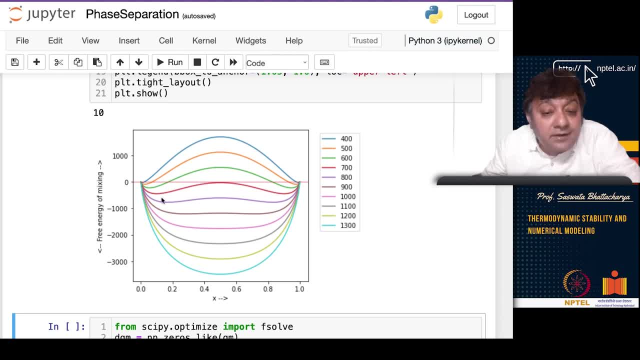 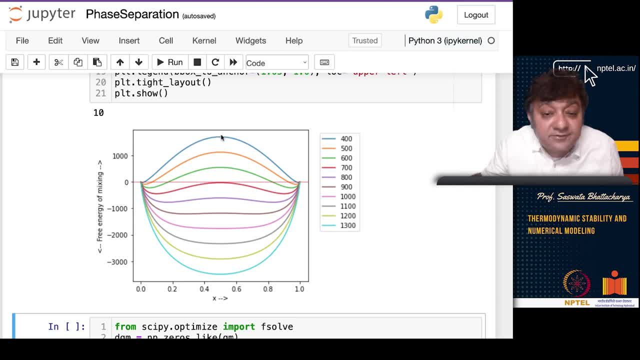 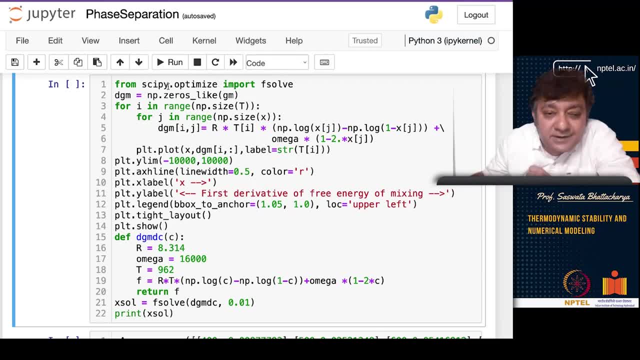 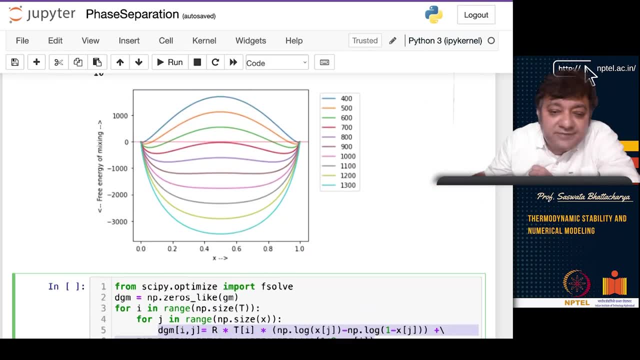 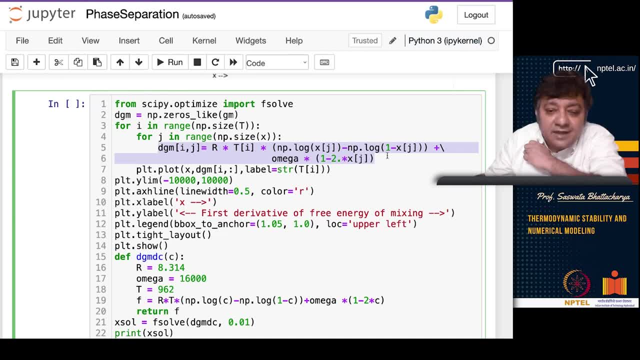 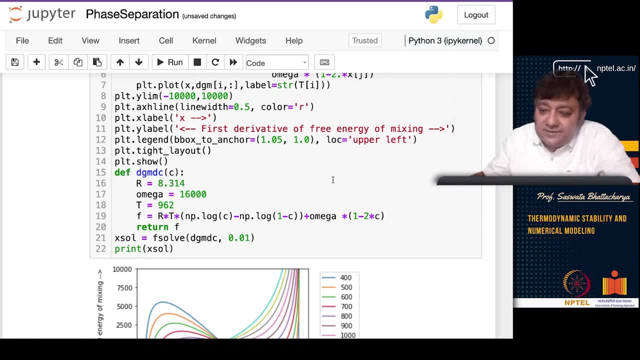 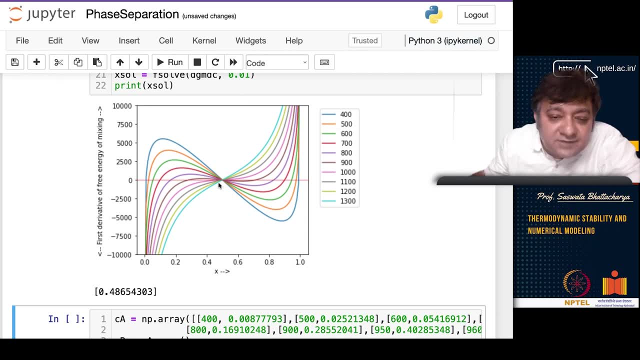 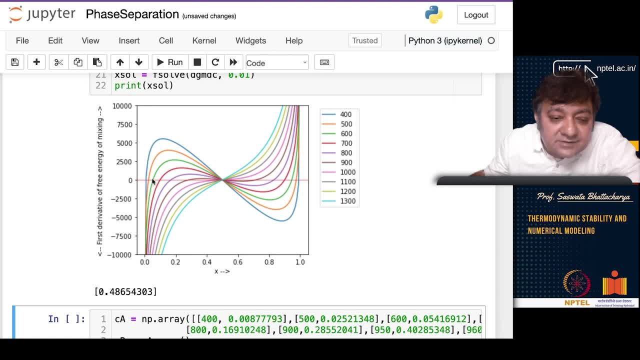 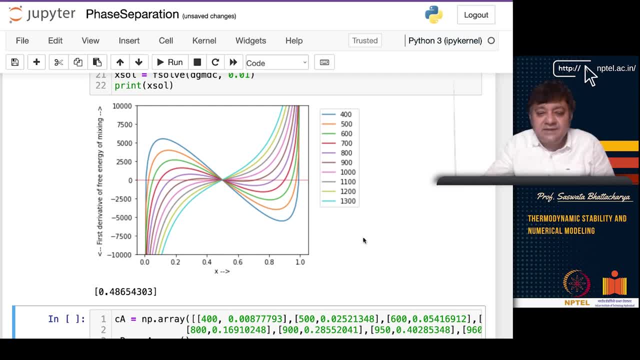 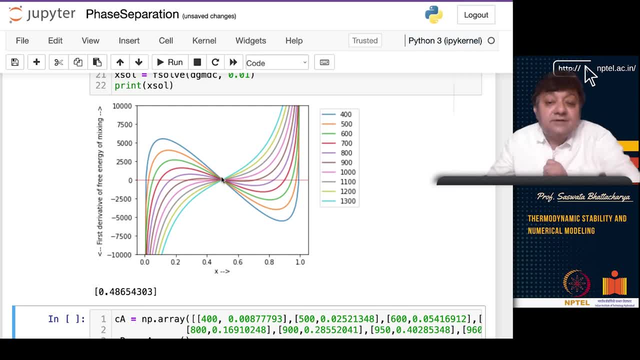 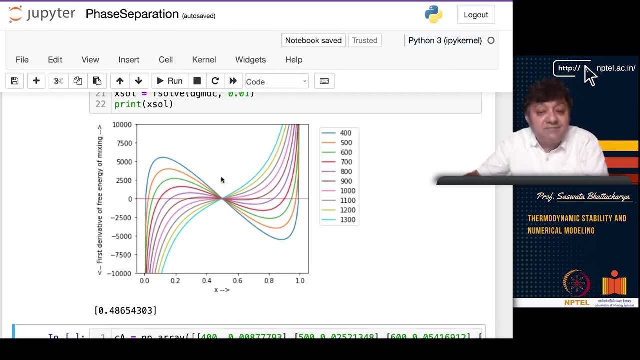 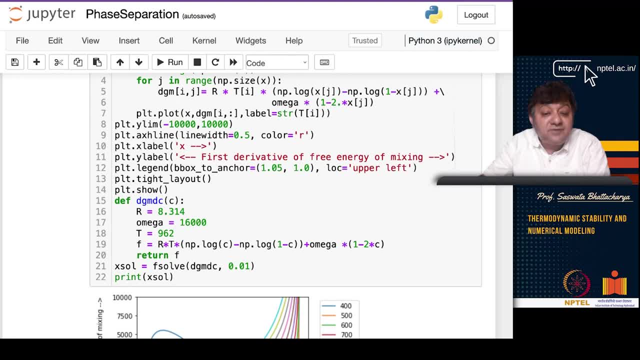 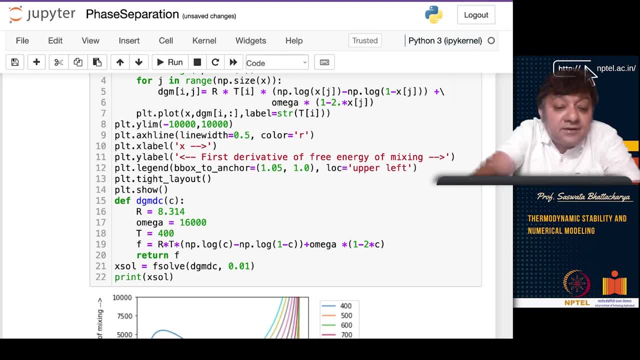 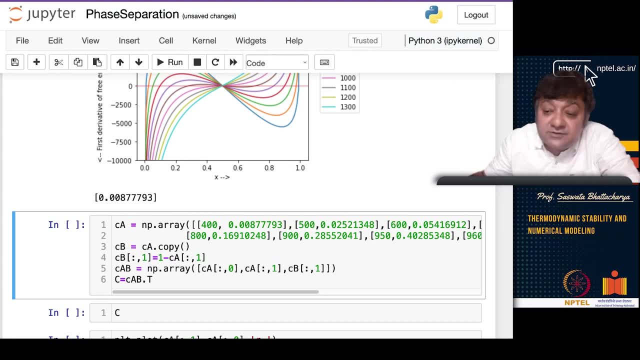 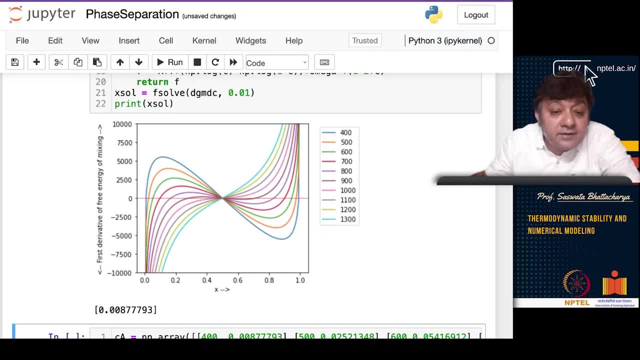 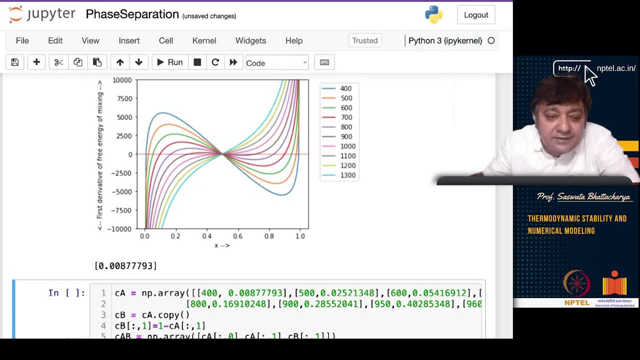 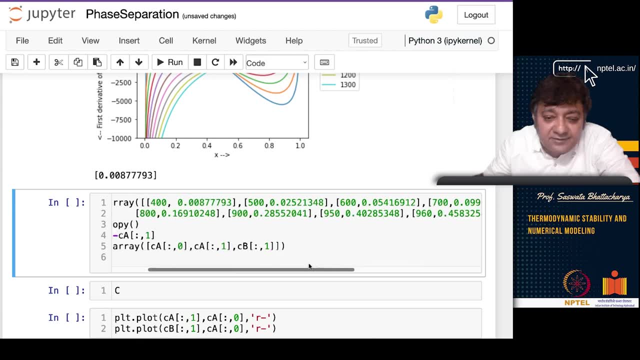 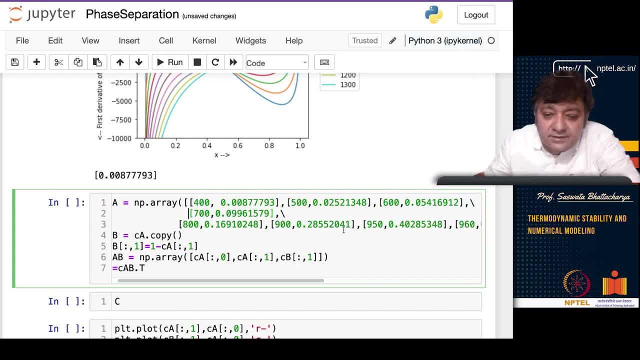 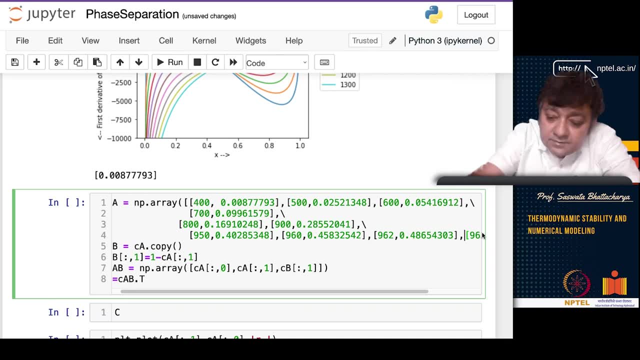 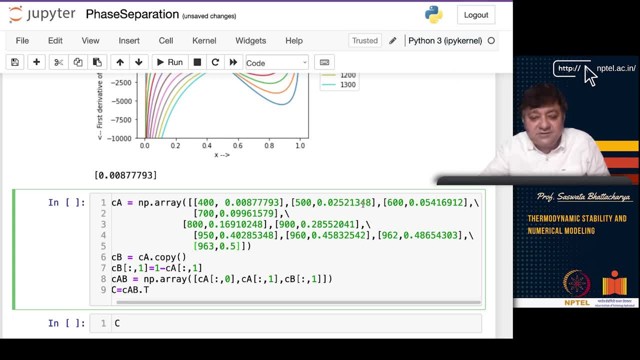 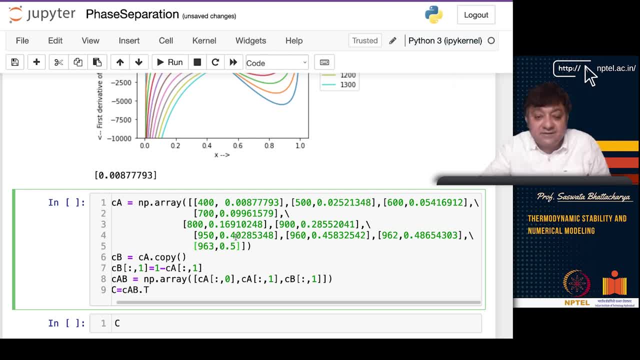 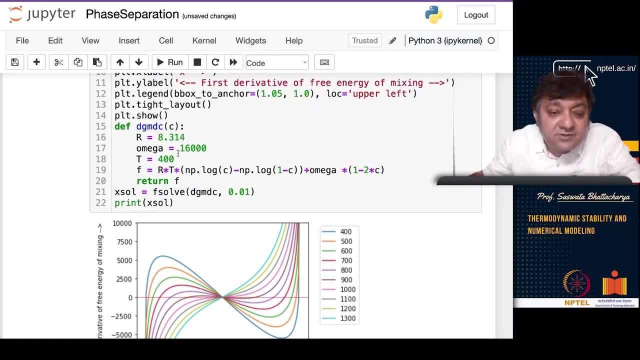 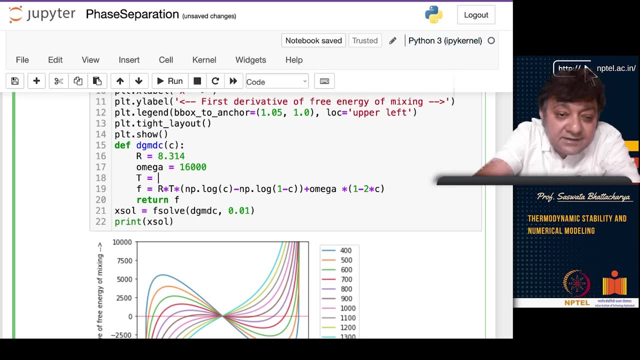 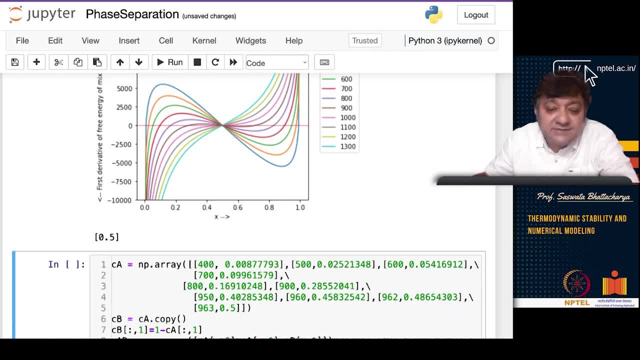 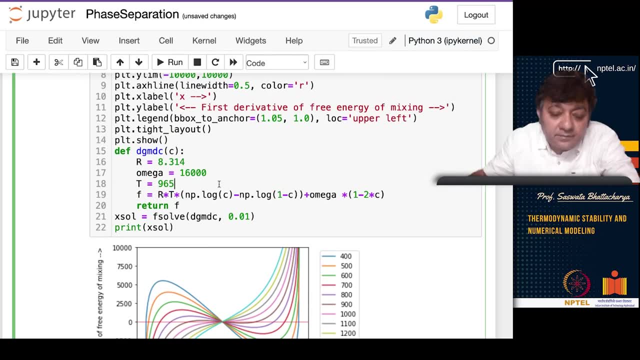 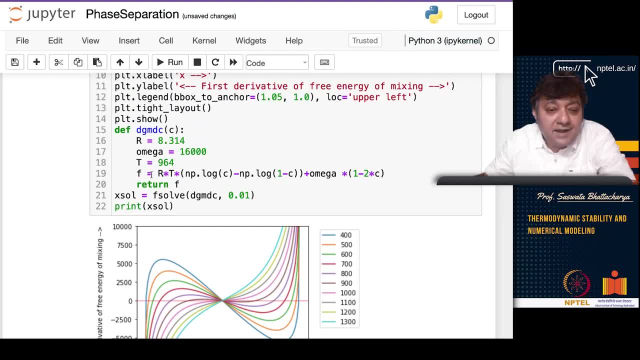 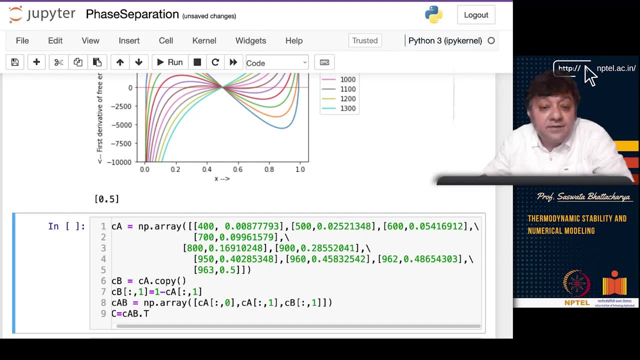 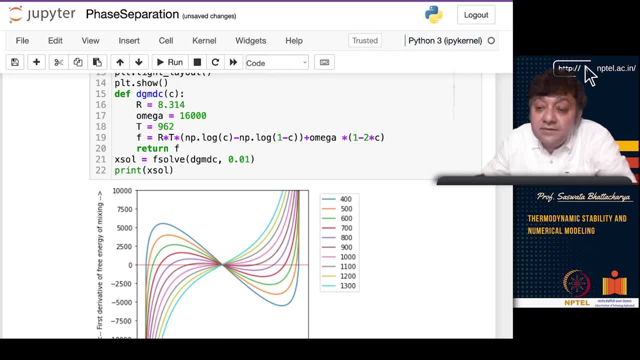 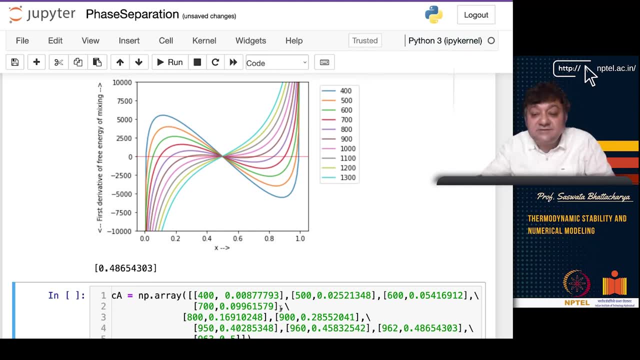 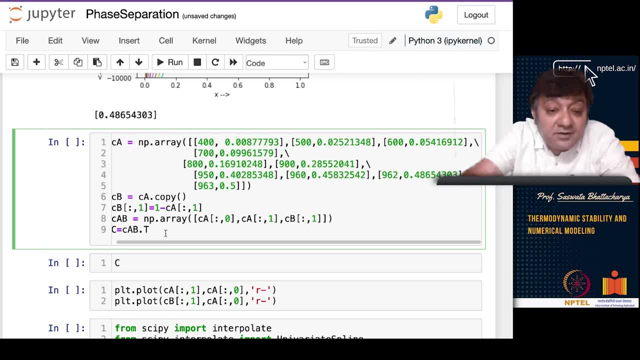 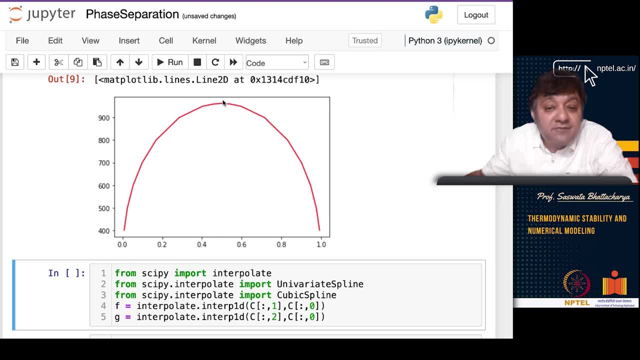 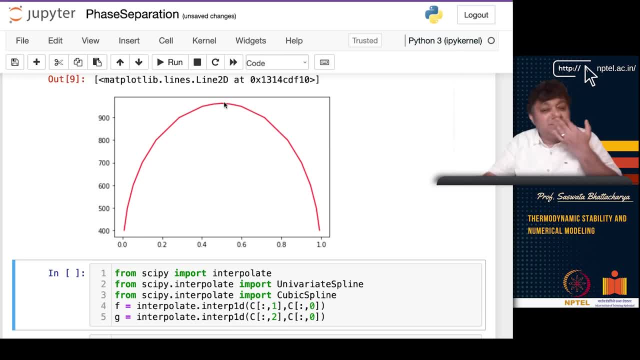 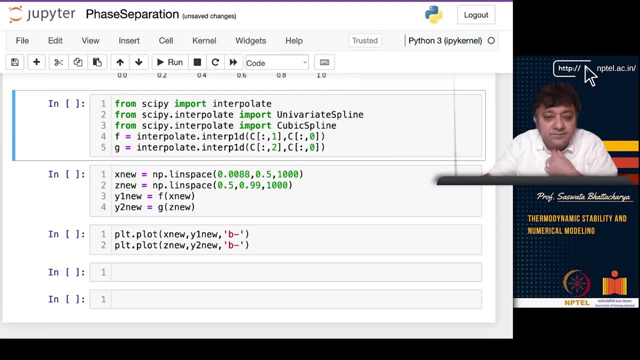 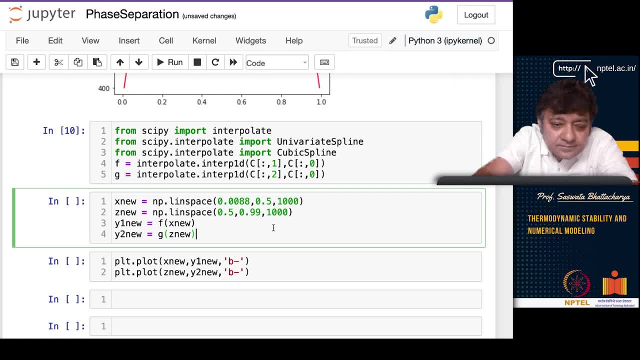 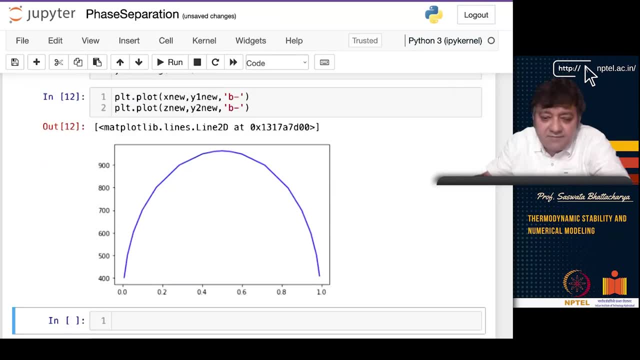 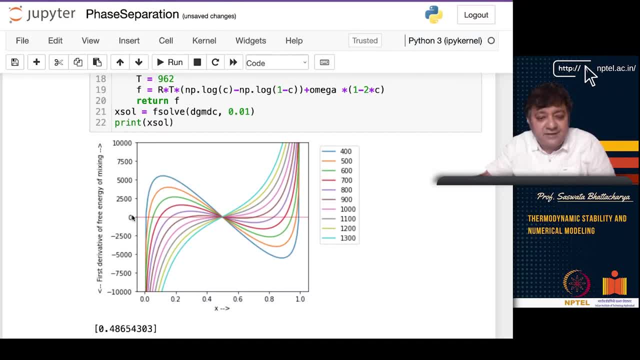 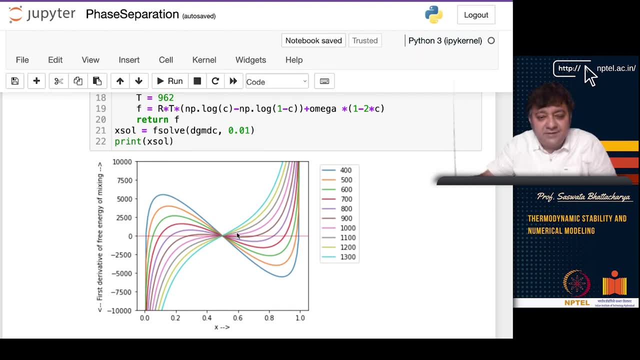 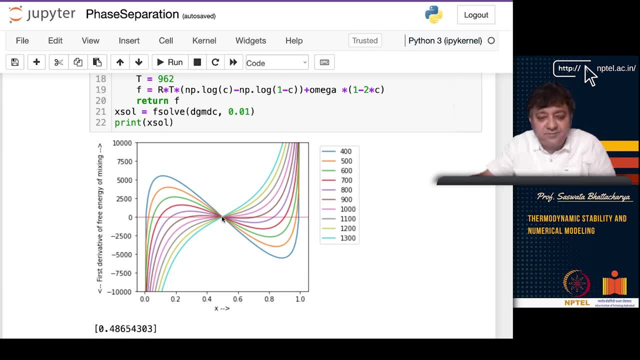 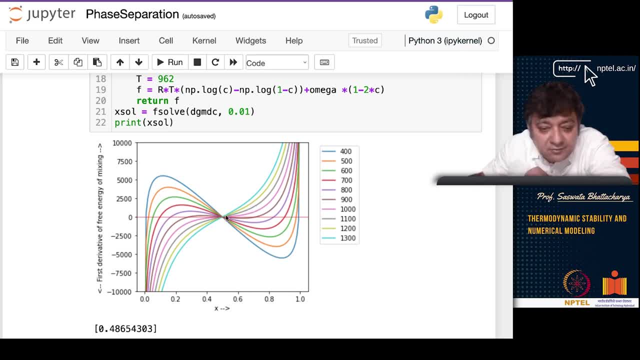 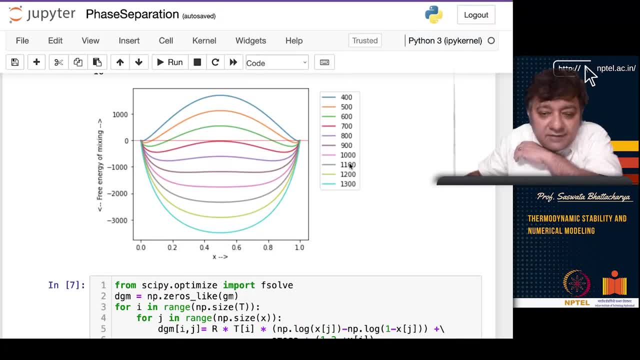 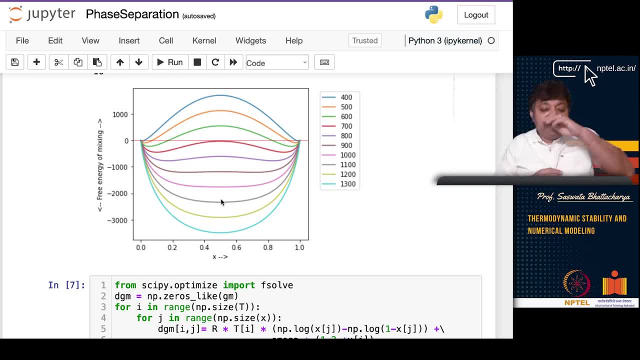 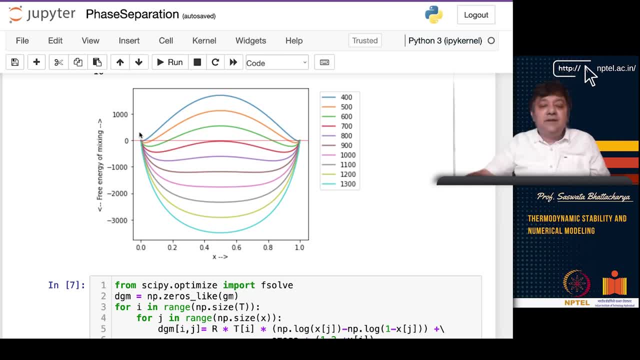 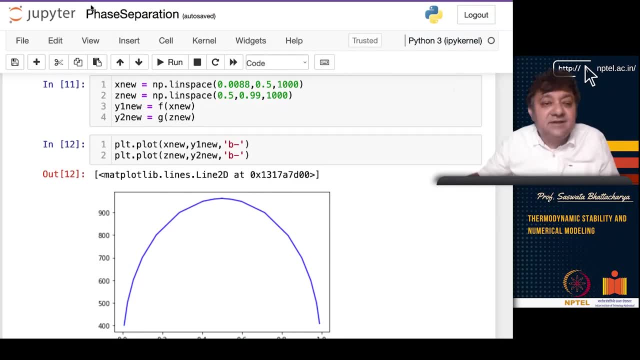 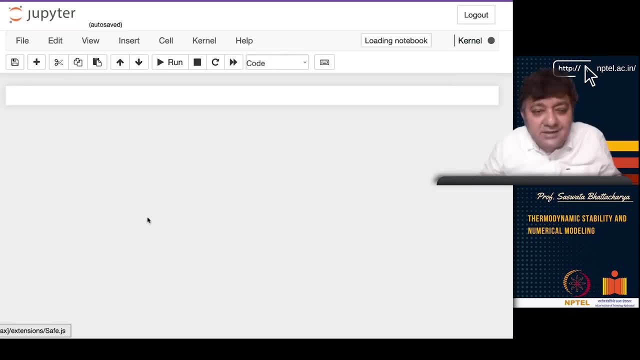 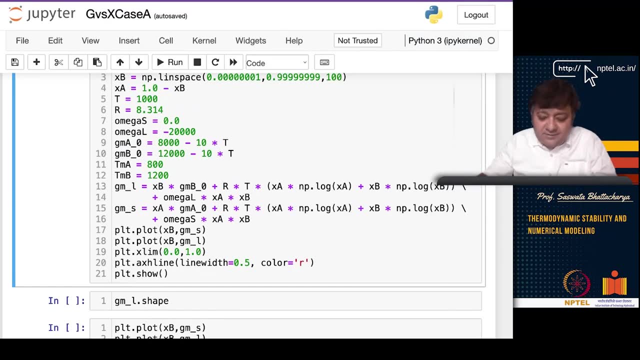 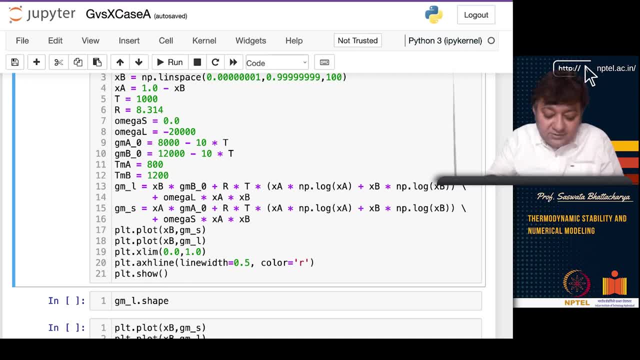 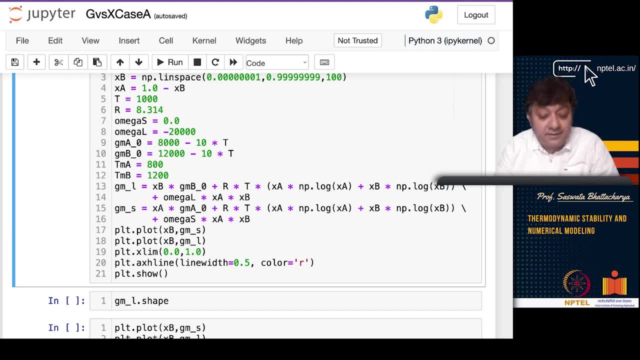 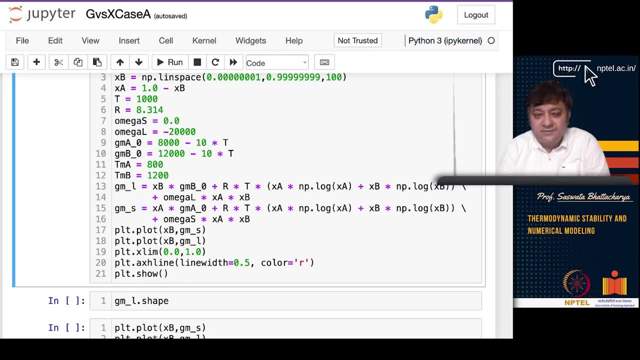 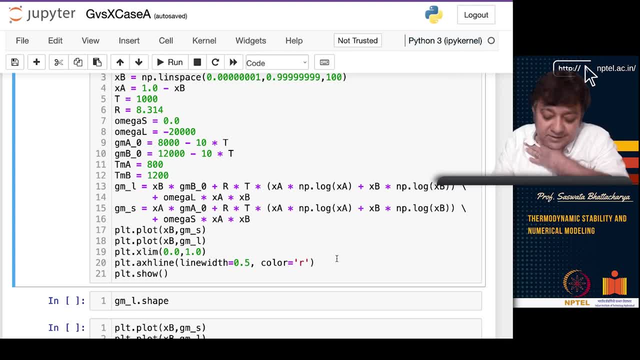 So, xB xA ln xA plus xB ln xB plus omega S xA xB. So, that is the model. So, I am giving you this is the model, right. gm solid is this and gm liquid is this. So, these are 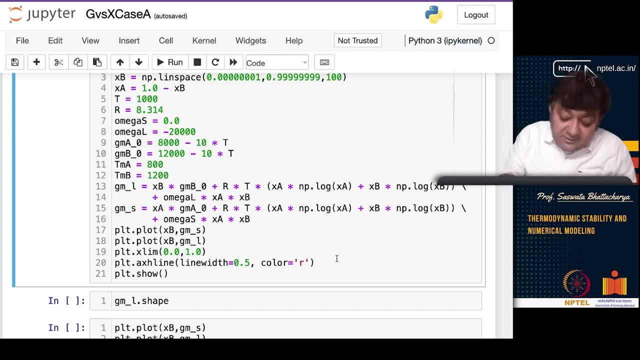 the, this is basically we are telling that here it will be only xA gm is 0. In this case when I am looking at solid and here it will be xA gm is 0, right, xA gm is 0. Now, if 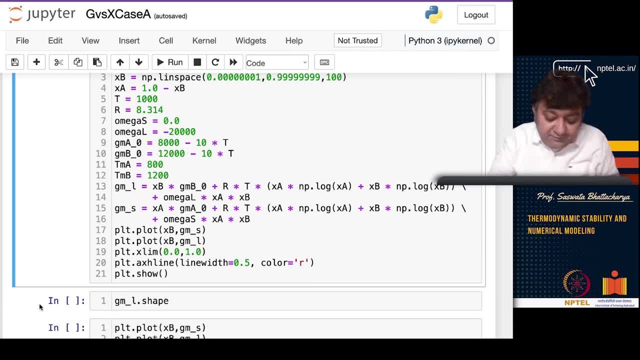 I see that this is for the liquid, for the liquid because the liquid will have, this 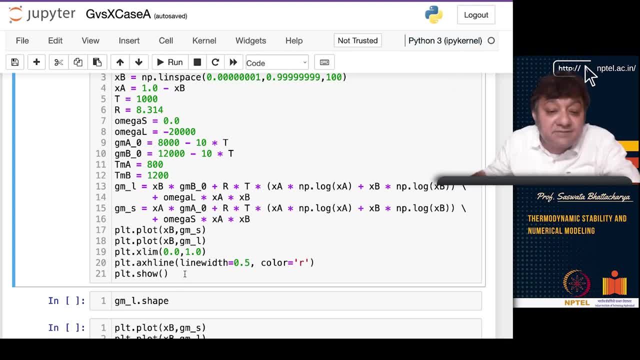 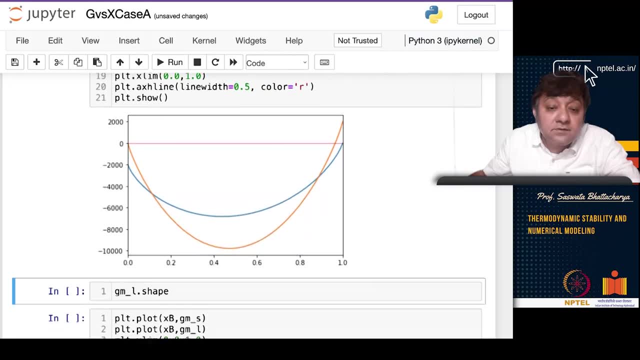 is alot of liquid. Now, if you have, that is like it will be only, this is plastic. What is the real thing you are seeing, this is a starts but motherfucking residAl, vas 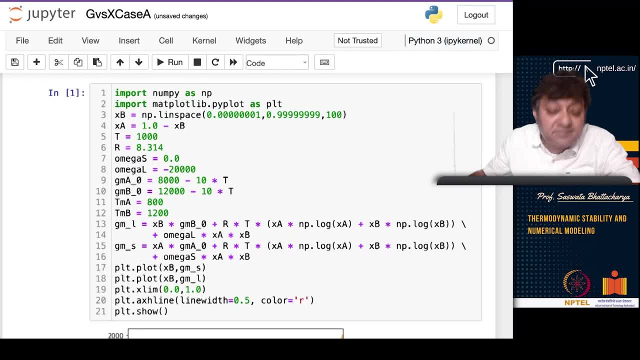 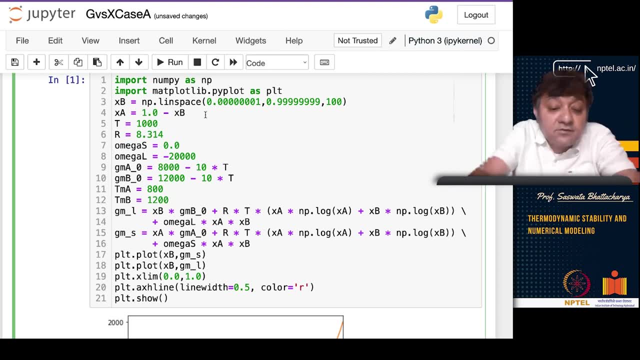 you are, ah, what is that you are, ah, so, ah, so, so, so, you will see that, ok. So, what does that mean. Basically, it gives you, this is the line, so, this is at some temperature of a 1000 degrees, ok. This is at some temperature of 1000 degrees. I can also do it at the temperature of say 1200 degree, I can see which is more stable. Now, if you look at that, if you do it at a, ok, this is the line, alright, this is at, ok, the line exactly, ja. 0 and this so, ja, again, that is a, this is 1. mouth of the body ggm 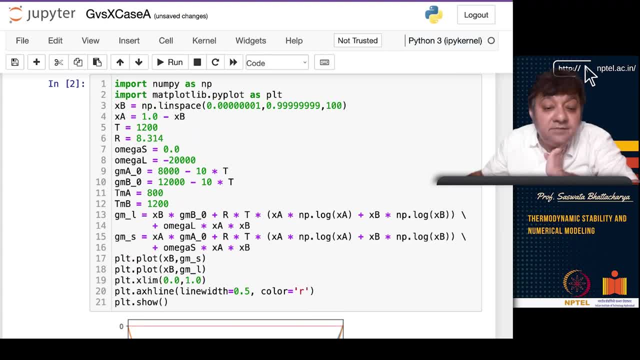 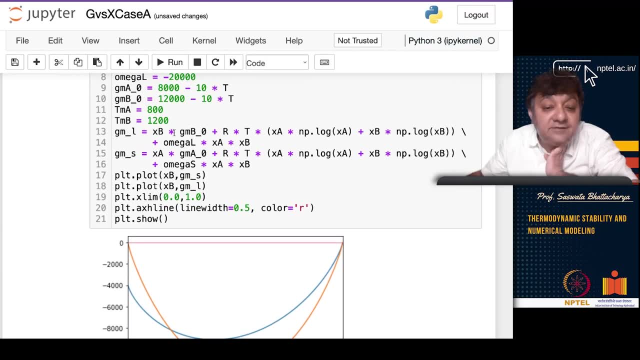 1200 degree. So, you have the first curve basically if I if I if I just see the liquid curve let us look at the liquid curve. So, this is the blue curve is a liquid curve no 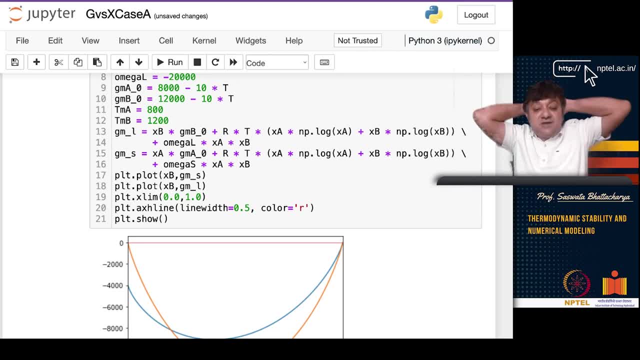 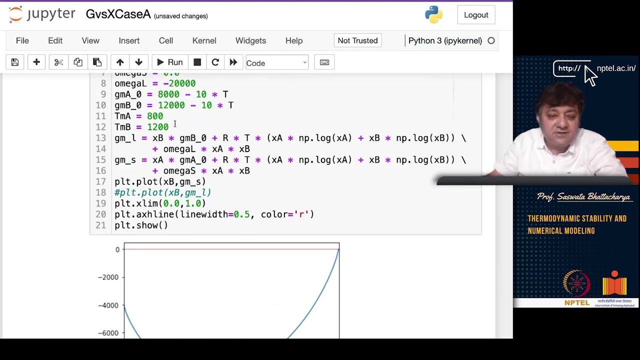 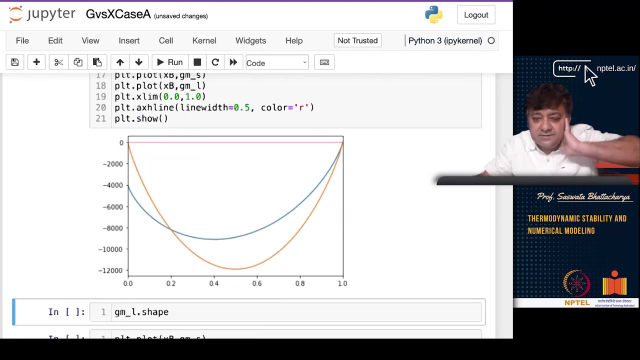 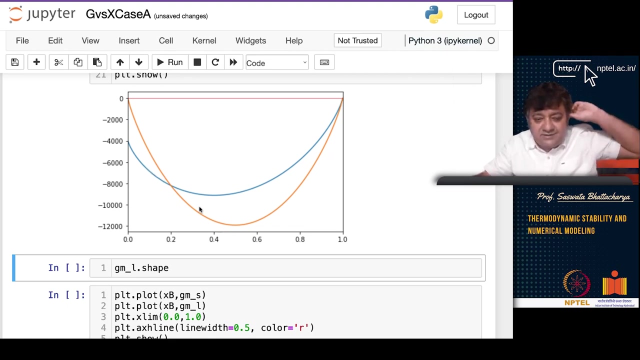 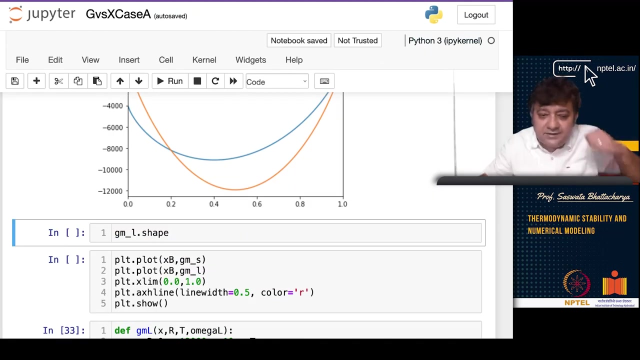 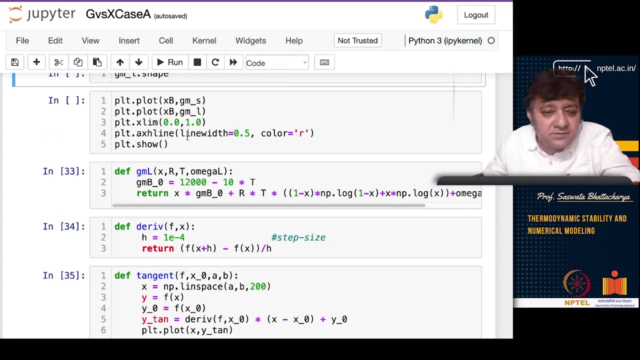 that the orange curve is a liquid curve the orange curve is a liquid curve and the solid curve is the present of the blue curve because if I just write these guys. So, you see as you can see this is the solid curve which has a value of minus yeah. So, you have this value right. So, you have a point. So, you have a minimum. However, it is not the minimum that I am looking at what I am looking at is the tangent construction. So, if I do this then you can immediately see the coexistence so, you have a coexistence here so, right you have a coexistence here. If you can look at my cursor understand that if I draw a common tangent so, that is the ideal. So, if I do that so, you can do the tangent also. 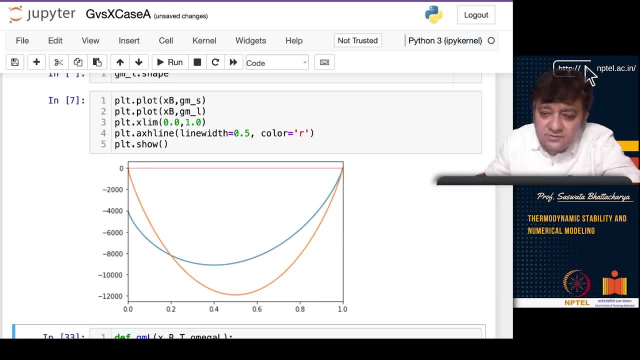 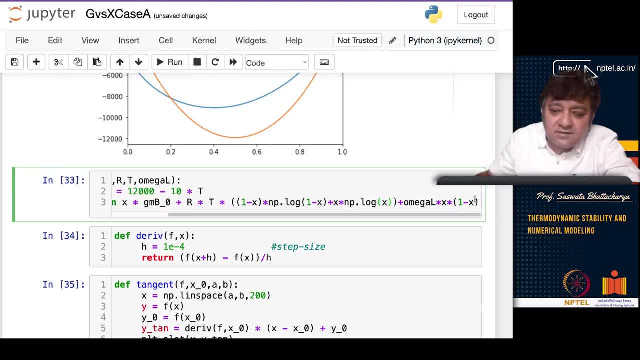 So, so I have this song like this you see this is correct song field ok this is correct ановa as. So, if I do the I will Very good. In the case of electric. If I will take electric for different temperatures, then I create this derivative and the tangent line equation and look 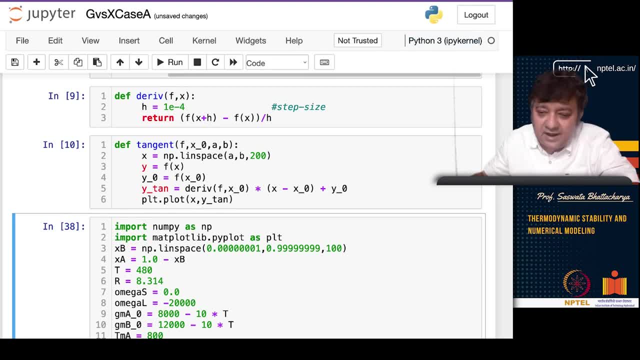 at that, if I do that, then at say some temperature, 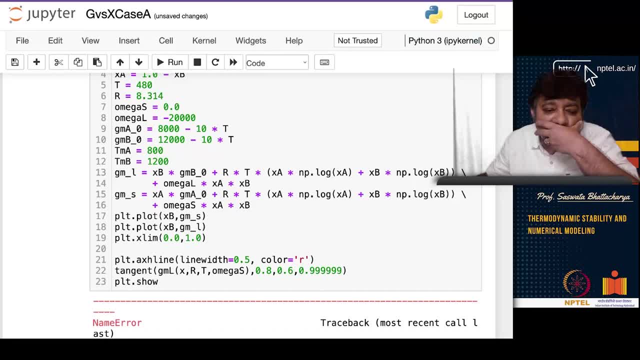 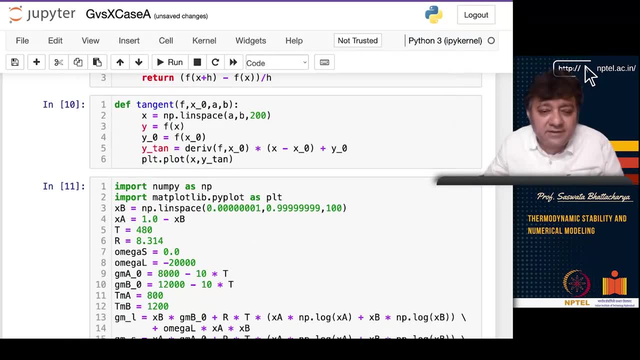 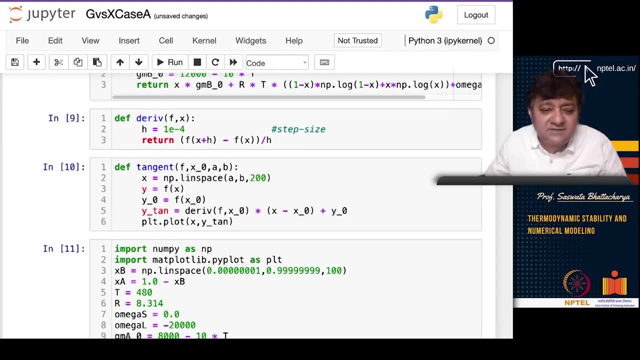 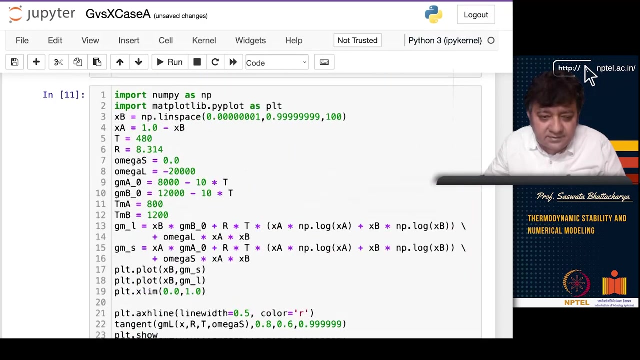 it is not defined, I do not see this, tangent has f x 0 a b, tangent has f, the g m l has x of t. Any other questions? 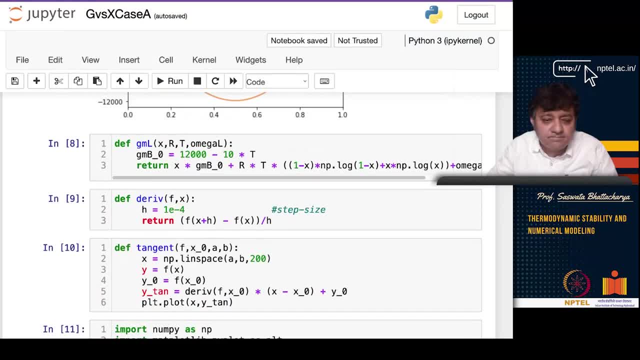 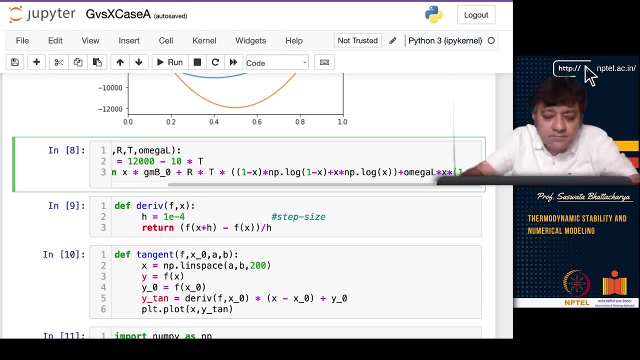 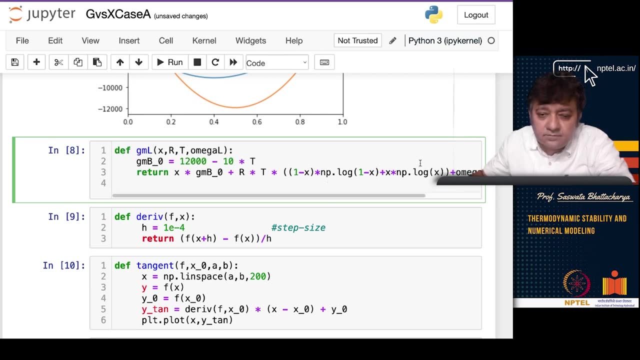 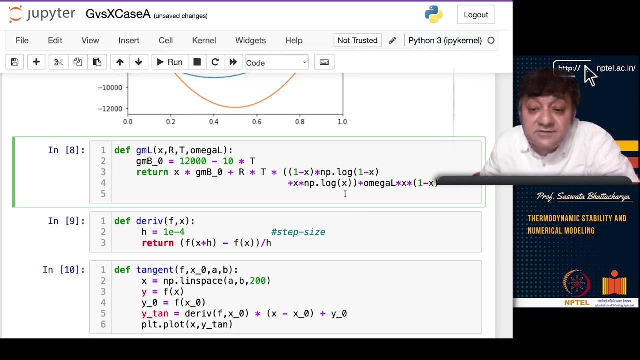 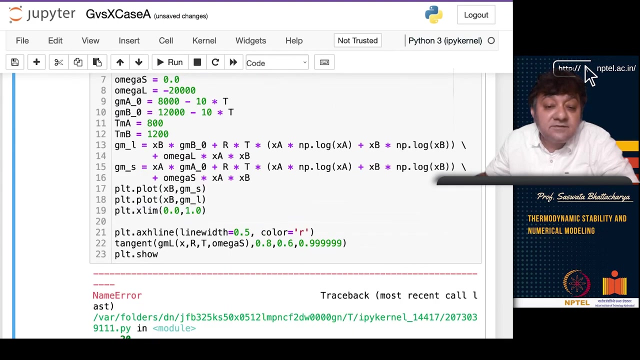 and I can make it a little bit of clean thing so if you look at this you have this term and this term now you have this mozai here here and this is the derivative and this is your tangent and then this becomes tangent and then this becomes tangent and then this becomes and then this becomes eration so I'll build that from this so I'll build that from this 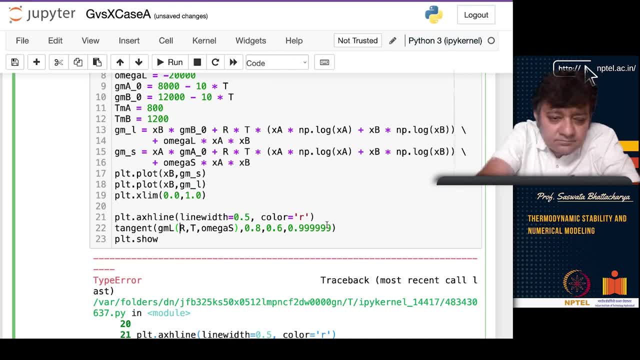 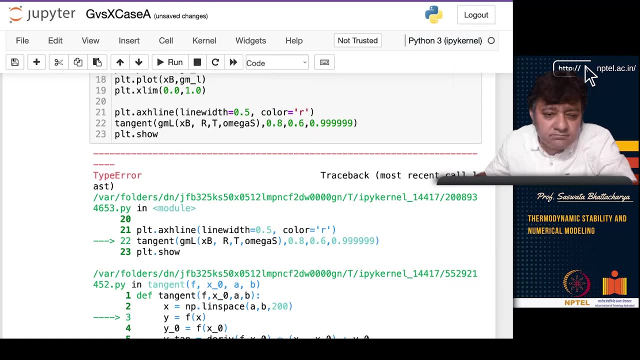 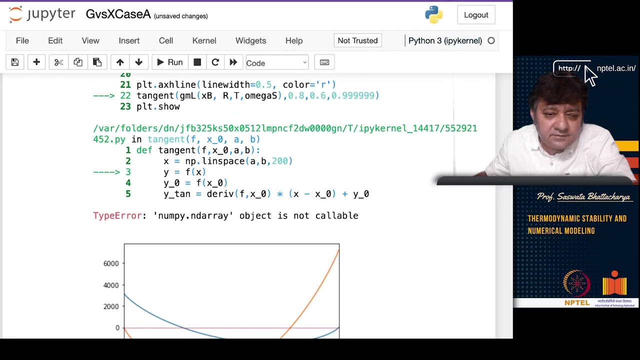 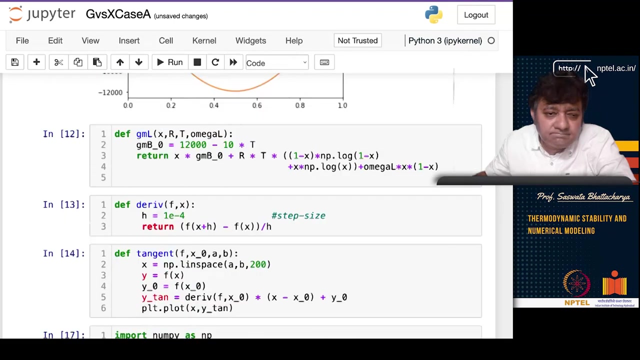 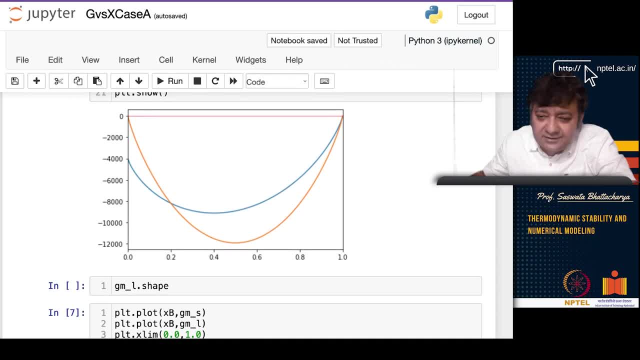 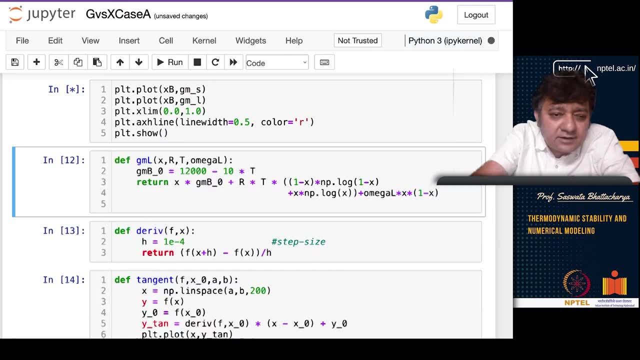 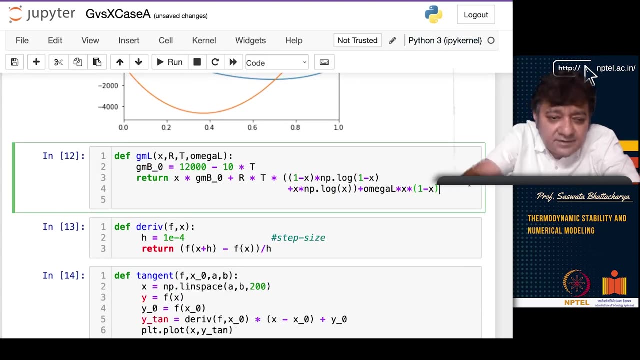 . . . . . . . Now this is the derivative equation, this is the tangent equation. . . Thank you. 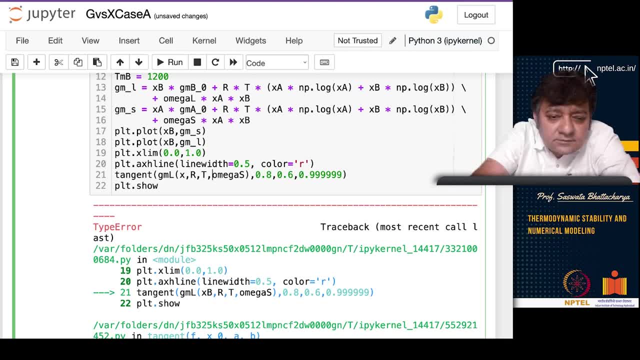 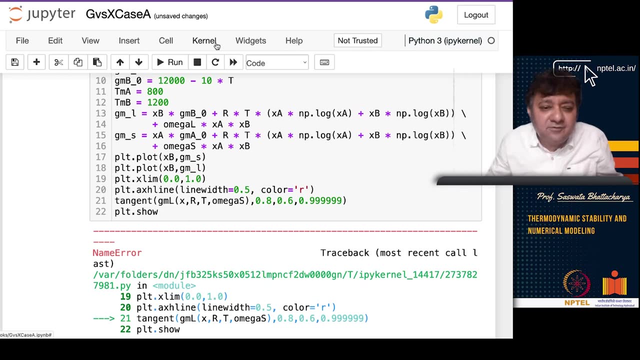 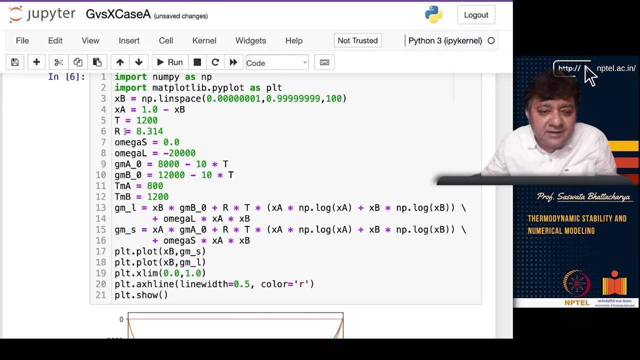 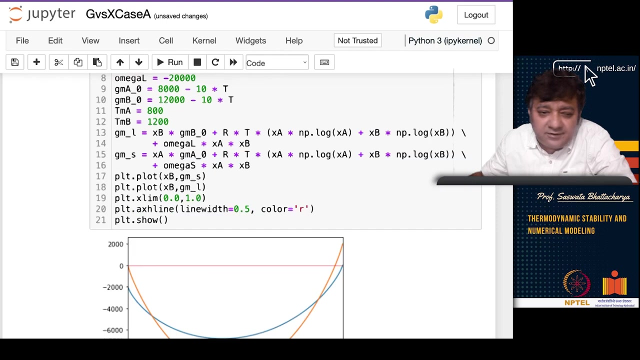 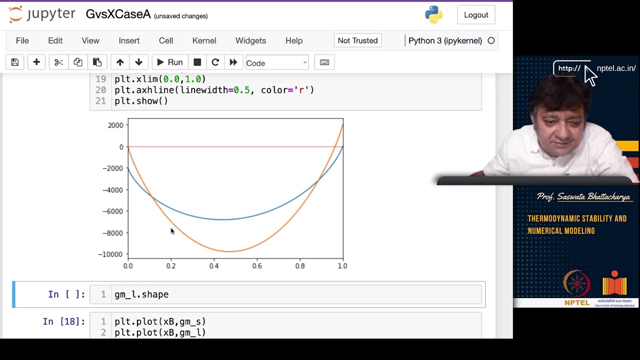 We will check this, I will get back to you, so I will get back to you with this particular error, but what I am trying to say is that for different temperatures, so basically I have done it for 1200, I can do it for 1000. And I can do it for different other temperatures, but what I am trying to say, if you draw the common tangent here, you can basically get the equilibrium values, right, you can get the equilibrium values, right. So, this is exactly what I am telling. 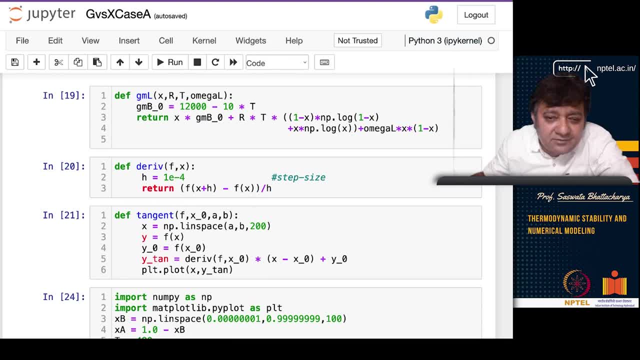 So, again you are plotting it at different temperatures and you are able to get it, right, you are able to get it. 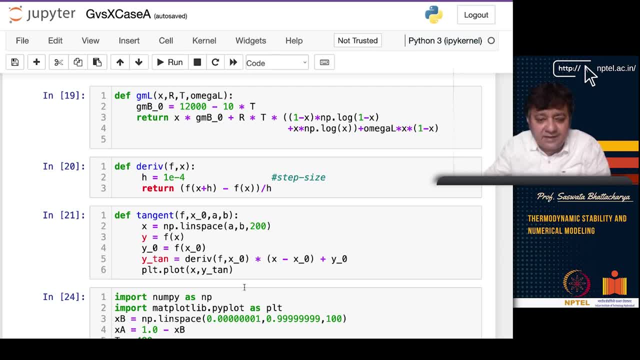 And see this is the GML value and yeah, so I will share this with you, I will just fix this part with the tangent line code. 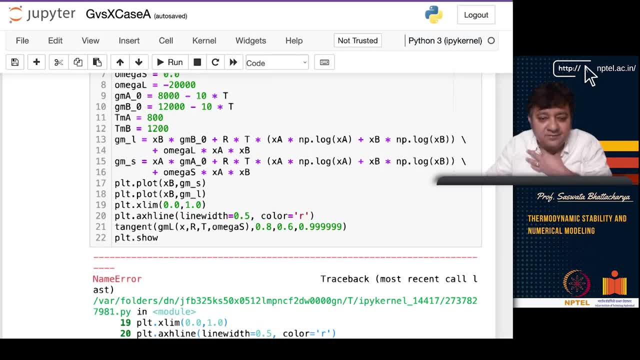 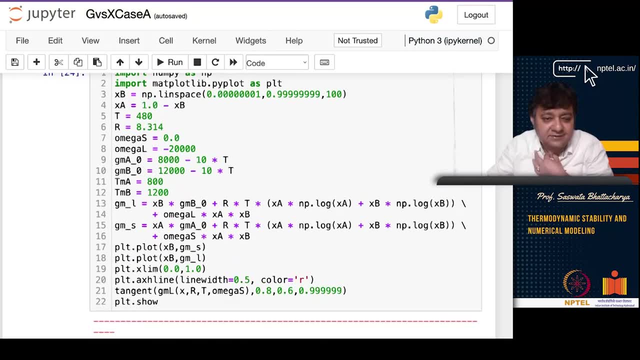 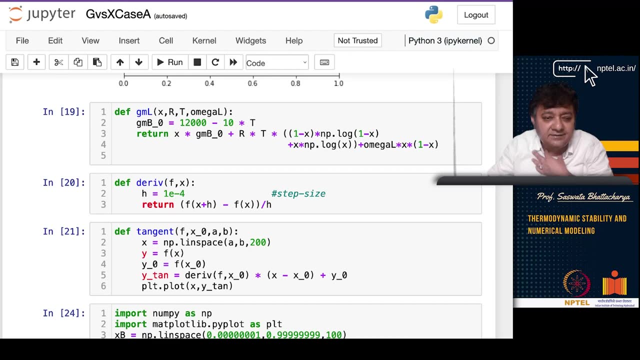 I do not know why suddenly this problem is happening, ok, so I will, I will fix this part and then it is telling name x is not defined, but that is something that looks very weird to me, because the x is definitely defined, so it is x is already defined here, x is nothing but x b. 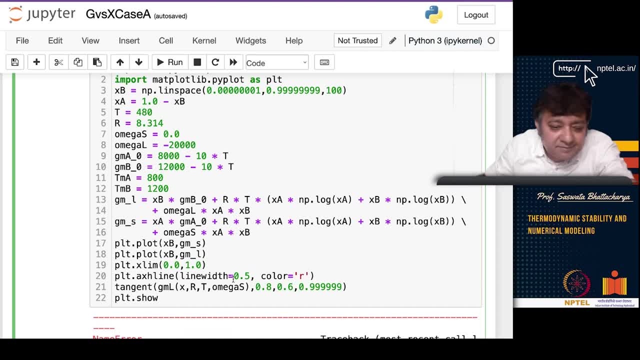 So, why am I doing the x b correctly, am I passing the x b correctly, this one we have a c, so x b. 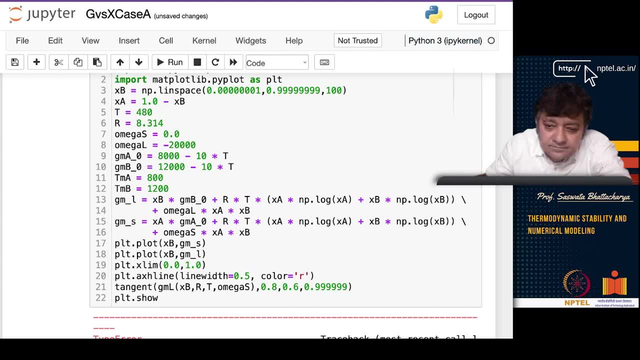 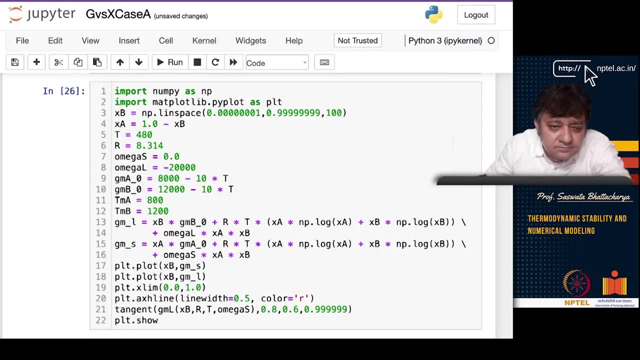 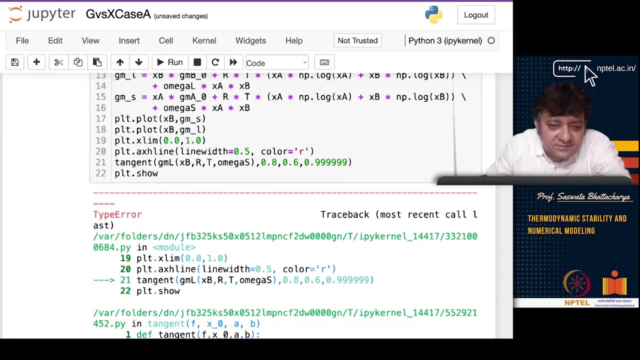 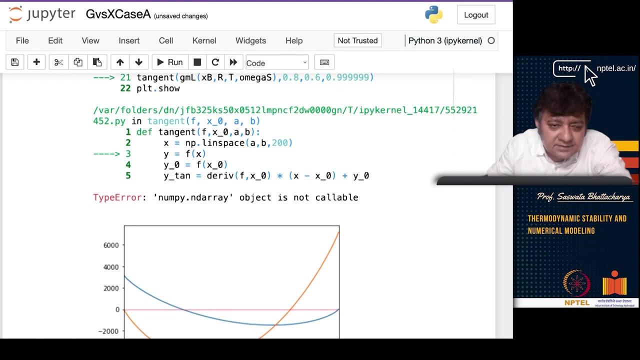 And this is like 0.8 and 0.6, so this is all fine, and it tells me y equal to f x. 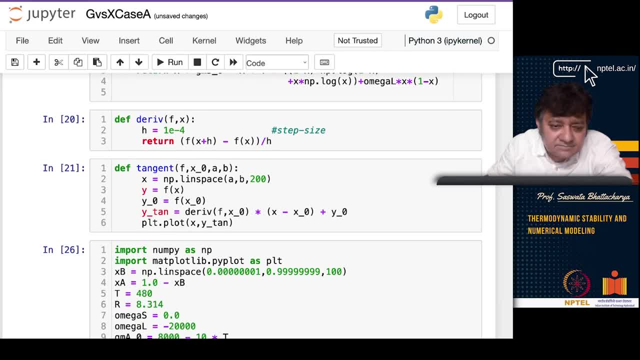 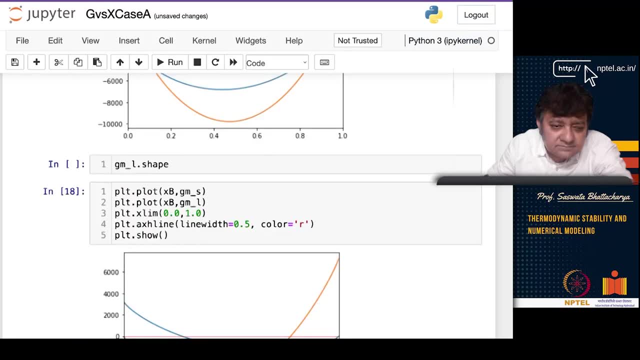 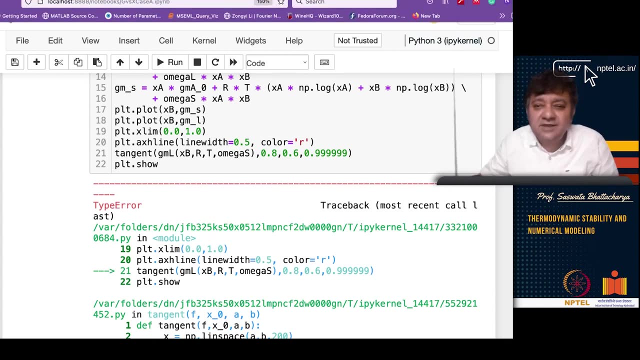 So, I will, I will, I will get back to you and I will share this thing, ok. So, next, in the next lecture I will go into the chemical reactions, ok. 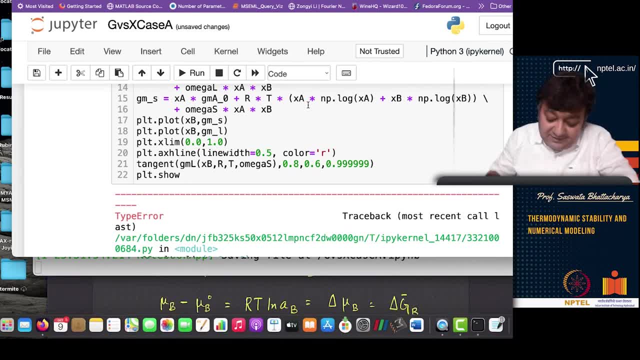 So, basically what I wanted to tell, so this part unfortunately this has some small problem, here we will fix this, ok. 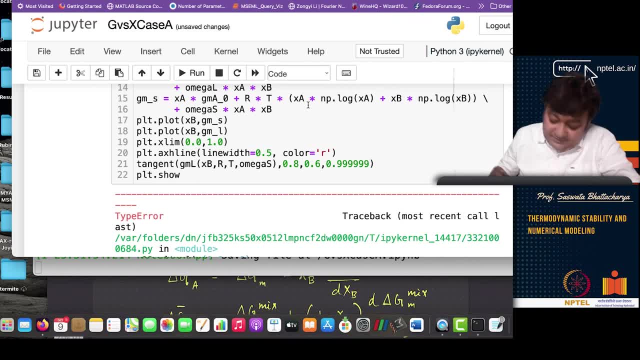 So, what I wanted to tell here is that if you do the delta g a bar, so basically as I am telling you that once you know these values, once you know these values, you can get the from the tangent, common tangent you can get the intercepts, right, you can get the mu a. 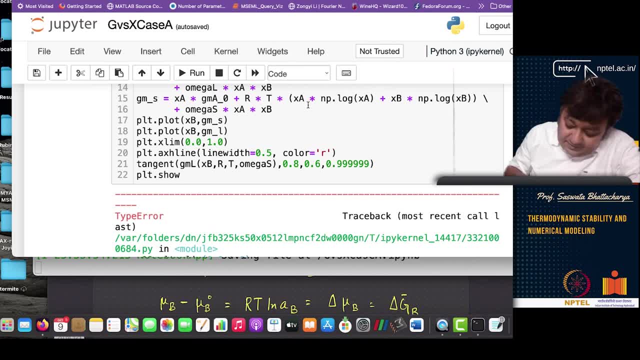 So, here I have anyway calculated them, I just want to show you numerically mu a and mu b, ok. 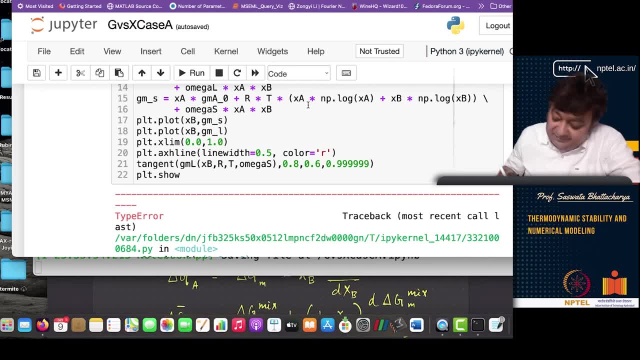 So, you have got it here. So, you get this values and you have the delta g a. 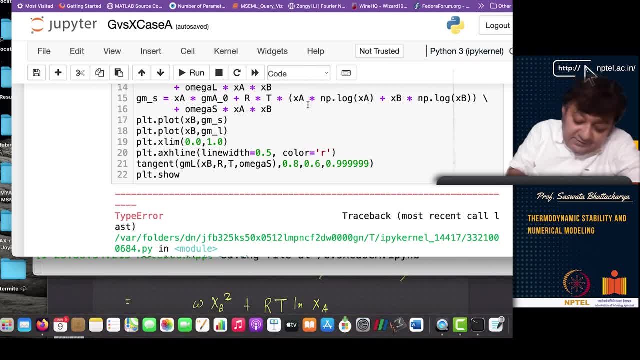 So, delta g a bar and the delta g b bar and you can basically get the activities, right, you can get the activities.